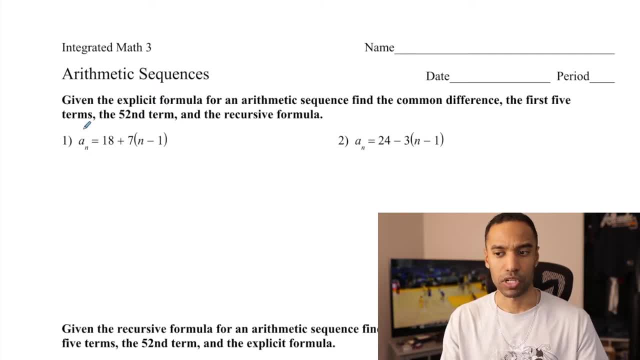 when it comes to whether they use subscripts notation or function notation. I do have older videos where I do have actually something on arithmetic sequences. I can even link it down below, but I use function notation instead. f of n Just depends on what's taught. This isn't necessarily something I do or anything else. 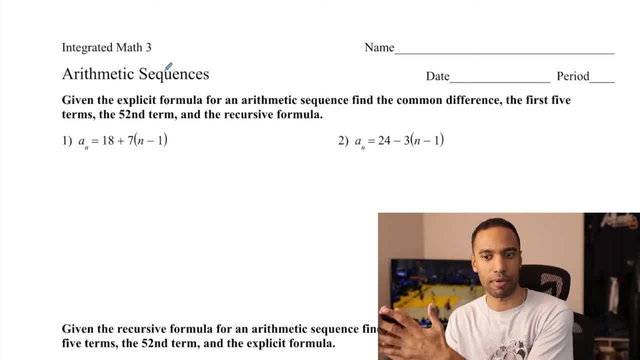 It's just, anything can be used. So just to make sure you know, you can see a sub n or f of n, or what have you there? Now, as far as the explicit formula goes, given the explicit formula, yada, yada. 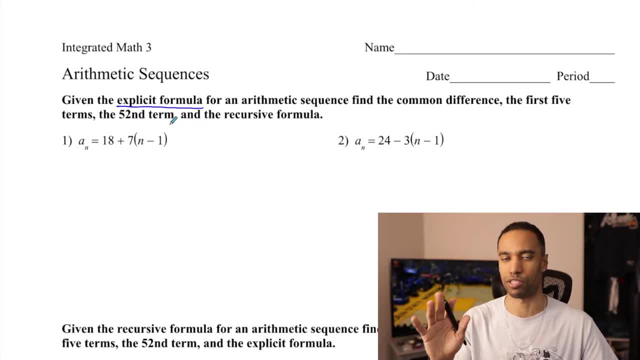 let me tell you what's up, what we're doing, what sequences are, in a very fast fashion and then go and do the problems. A subscript like this, n right here, Represents different varieties of a. We could have a excuse me, sorry. 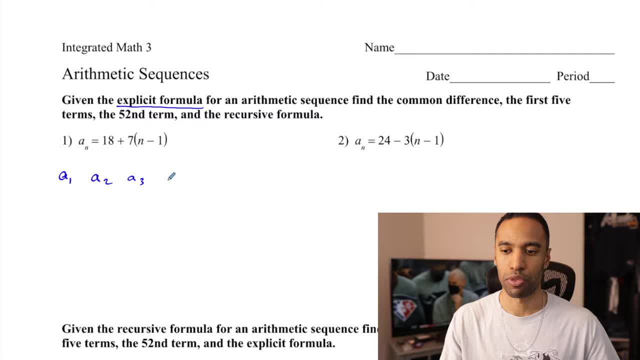 We could have a sub 1, a sub 2, a sub 3, etc. And these are just here are different a's A stands for, it doesn't stand for arithmetic or anything, It's just a letter that's going to represent our output variable, the value in a sequence. 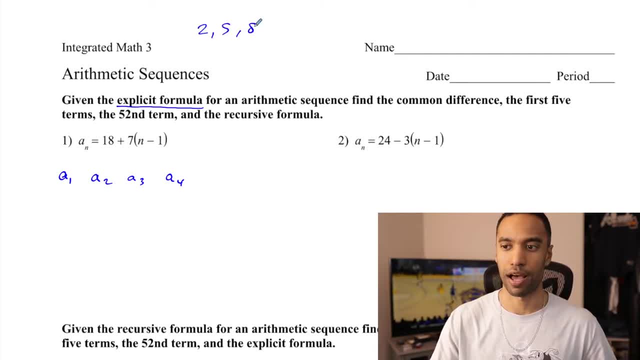 A sequence is just a list of numbers. I could have 2,, 5,, 8,, 11,, 14.. And this is an example of an arithmetic sequence, because it's a list of numbers that feature what's called a common. 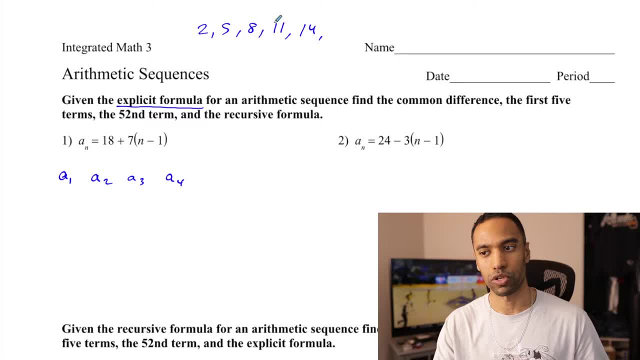 difference That they are separated by the addition or subtraction of the same number over and over, in this case 3.. The common difference there is 3.. So this is the value of the first term. This would be a sub 1.. This is a sub 2, a sub 3, a sub 4, etc. 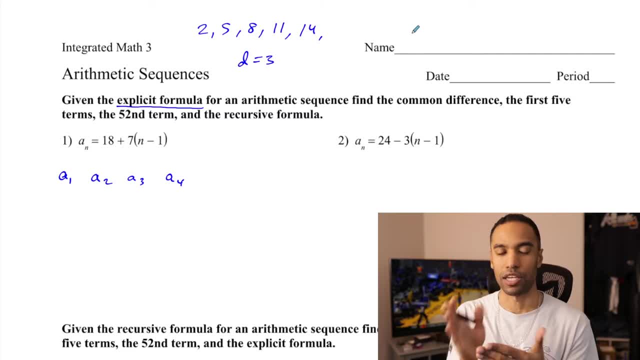 It is implied that the head of the list is the first value and that you increase your value by 1 each time. I'm saying that all very fast, so we can go ahead and get started on this Now. what these equations are showing you is that based on when it says a sub n. 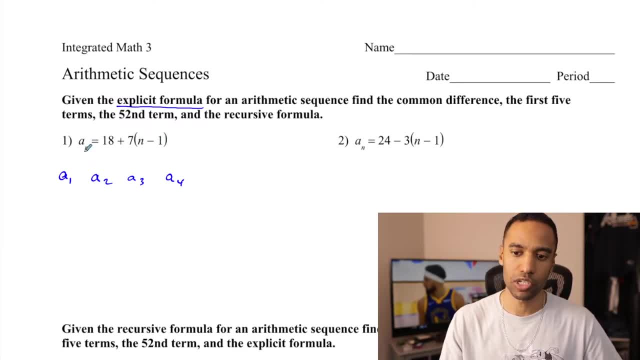 equals 18 plus 7 times n minus 1,. what it's stating is: you can substitute a value in for n, like 1,, 2,, 3,, 4,, 100, whatever it is, And this equation actually uses that number to make your computation right here. 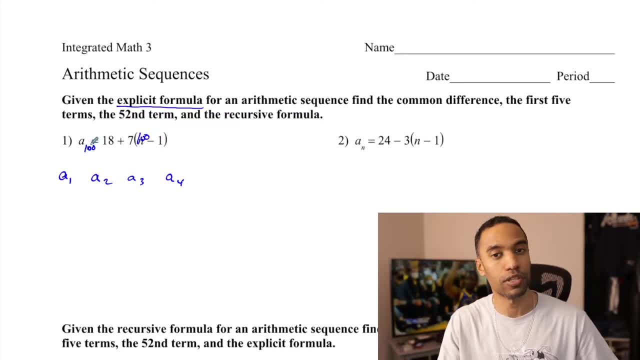 100 could go inside here and you could find the value of the 100th term. You actually literally use the number 100 to compute it, And that's what an explicit formula does, And that's what we're doing here. So we are going to given the explicit formula. oh, by the way, I'll write out the actual formula in and of itself. 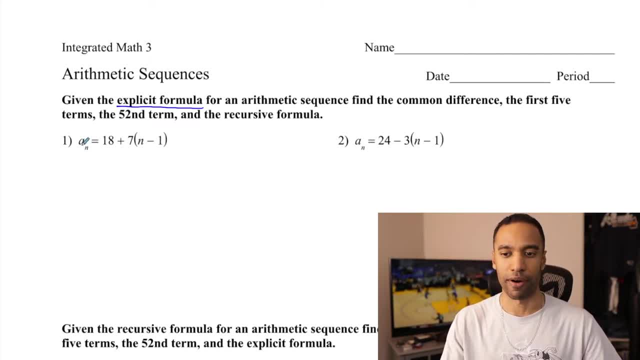 A subscript like this n right here. Represents different varieties of a. We could have a, excuse me, sorry. We could have a sub 1, a sub 2, a sub 3, etc. 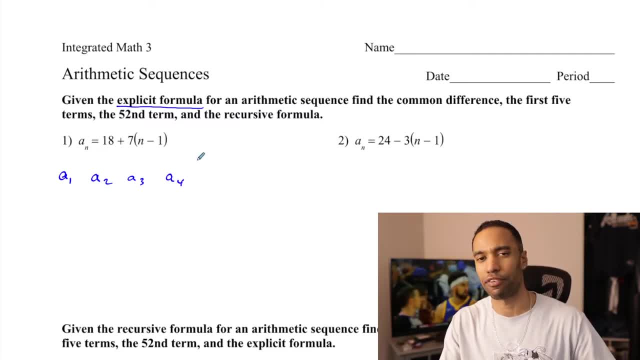 And these are just, here are different a's. A stands for, it doesn't stand for arithmetic or anything. It's just a letter that's going to represent our output variable, the value in a sequence. 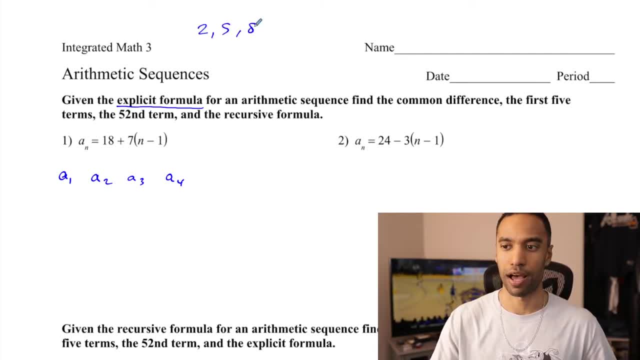 A sequence is just a list of numbers. I could have 2, 5, 8, 11, 14. And this is an example of an arithmetic sequence because it's a list of numbers that feature what's called a common, difference, that they are separated by the addition or subtraction of the same number over and over, in this case, 3. 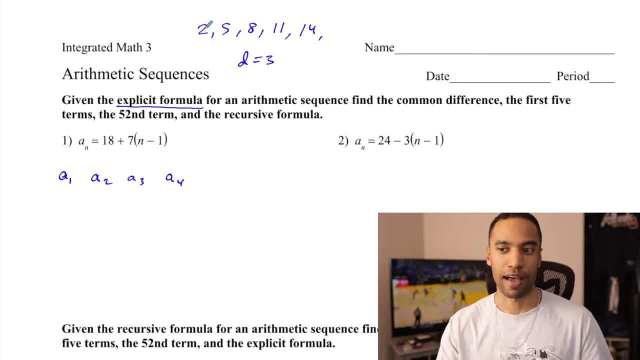 The common difference there is 3. So, this is the value of the first term. This would be a sub 1. This is a sub 2, a sub 3, a sub 4, etc. It is implied that the head of the list is the first value and that you increase your value by 1 each time. 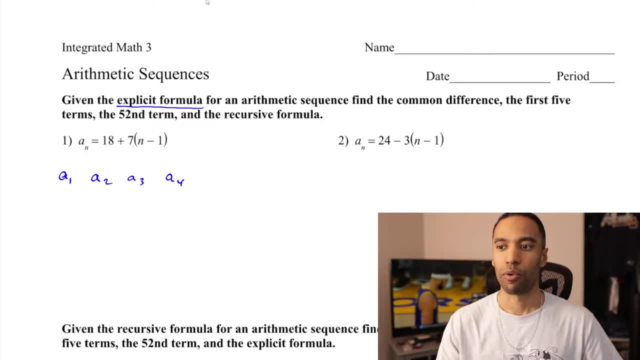 I'm saying that all very fast so we can go ahead and get started on this. Now, what these equations are showing you is that based on when it says a sub n equals, 18 plus 7 times n minus 1, what it's stating is you can substitute a value in for n, like 1, 2, 3, 4, 100, whatever it is. And this equation actually uses that number to make your computation right here. 100 could go inside here and you could find the value of the 100th term. You actually literally use the number 100 to compute it. And that's what an explicit formula does. And that's what we're doing here. So, we are going to, given the explicit formula, oh, by the way, I'll write out the actual formula in and of itself. 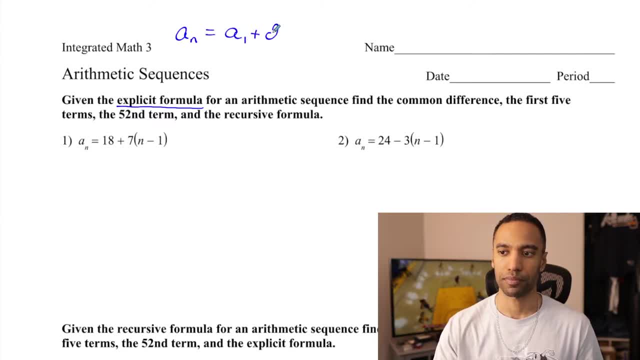 So, it's a sub n equals a sub 1 plus d times n minus 1. 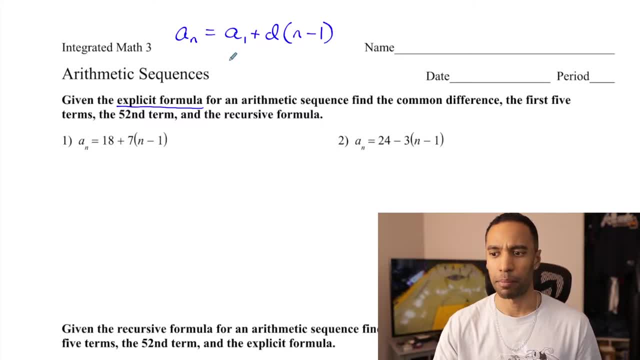 So, this formula very specifically, and there are other versions of it. I don't think the other one is going to show up here, but it would be a sub n equals a sub 0 plus d times n, if you ever see this. 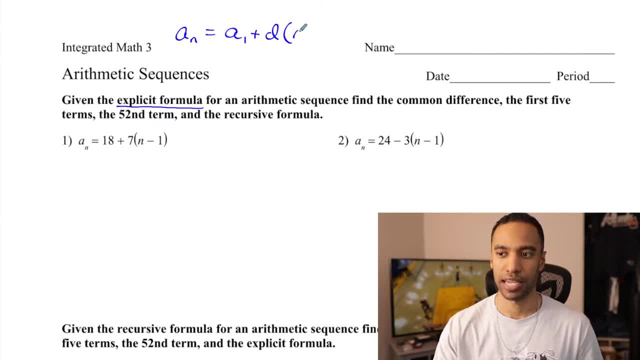 So a sub n equals a sub 1 plus d times n minus 1.. So this formula very specifically- and there are other versions of it. I don't think the other one is going to show up here, but it would be- a sub n equals a sub 0 plus d times n, if you ever see this. 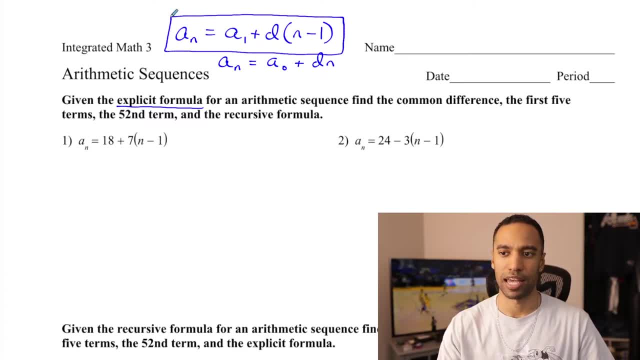 But this initial one, right here. what it's saying is that to find the value of any nth term, whatever term you want to find the 10th term, the 25th term, you start from the first term and you add that common difference a certain number of times, over and over and over. 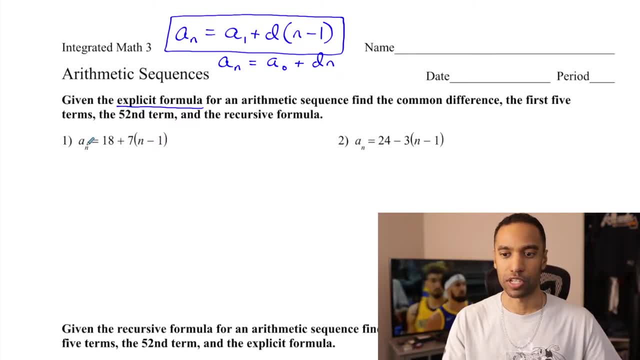 Again. so for this one, if I want to find some term like the 20th term, I would start from the number 18, which actually is the first term, And I'm going to add 7 over and over 20 minus 1 times 19 times. 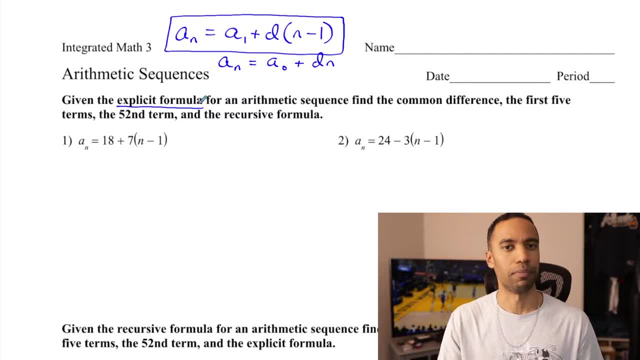 Why would I add 7, 19 times to get to the 20th term, or 99 times to get to the 100th term? Well, because we start on. the first term is 18.. So if I wanted to find the second term, I would do plus seven just once to find the second term. 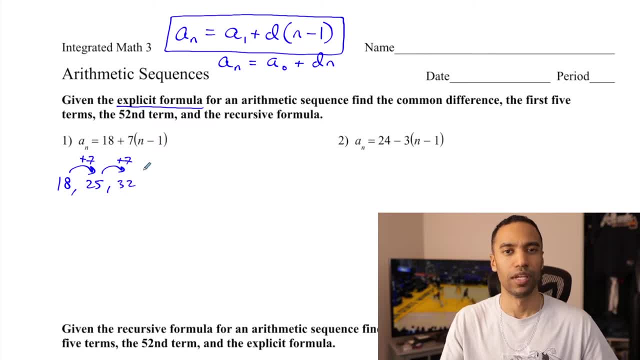 Right Plus seven twice To find the third term. So you see, you're always adding one less seven than you would before. That's what this formula say. This formula gives you a theoretical, a sub zero, some zeroth term, a term that existed before these ever did. 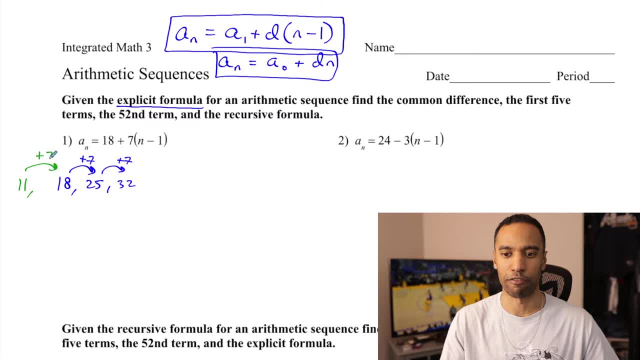 Seven units before. like this and says: to find the value of the first term you add seven once. To find the value of the second term, you add seven twice. Kind of a neat, little way to do it, The way that our school is teaching it, our department and such. 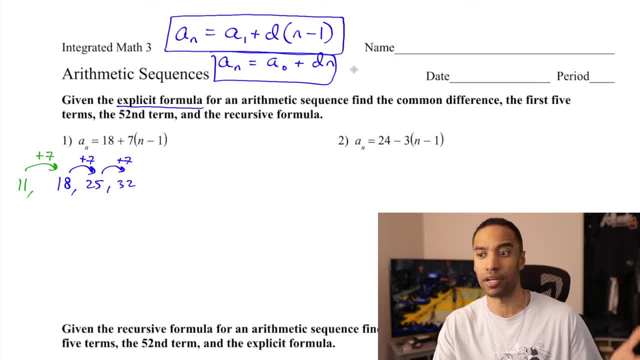 is mostly with the a sub one and the n minus one right here, But you can see either the idea of an explicit rule, And I know I haven't started, This is just me teaching it to begin with. The idea of an explicit rule, though, is that you do substitute your position. 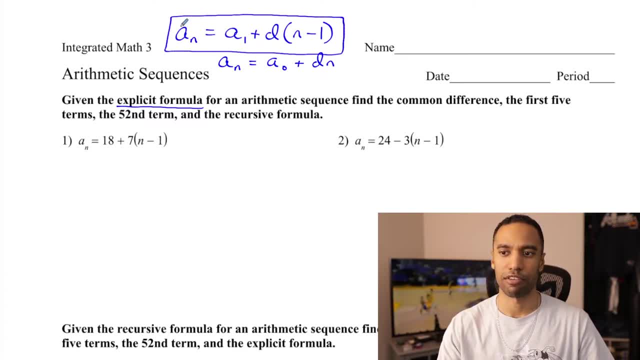 But this initial one right here, what it's saying is that to find the value of any nth term, whatever term you want to find, the 10th term, the 25th term, you start from the first term and you add that common difference a certain number of times over. And over and over again. So, for this one, if I want to find some term, like the 20th term, I would start from the number 18, which actually is the first term. 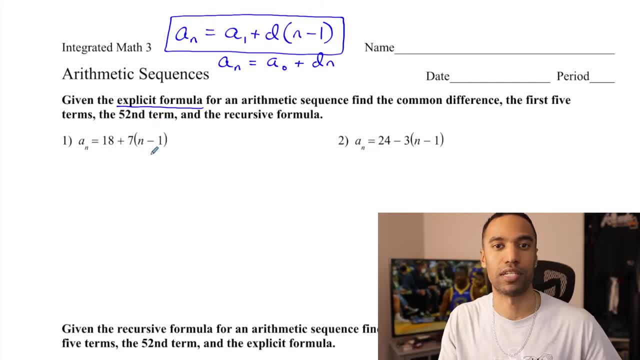 And I'm going to add 7 over and over. 20 minus 1 times. 19 times. Why would I add 7 19 times to get to the 20th term? Or 99 times to get to the 100th term? Well, because we start on the first term as 18. So, if I wanted to find the second term, I would do plus 7 just once to find the second term. Plus 7 twice to find the third term. So, you see you're always adding 1 less 7 than you would before. That's what this formula is saying. This formula gives you a theoretical a sub 0, some 0th term, a term that existed before these ever did. 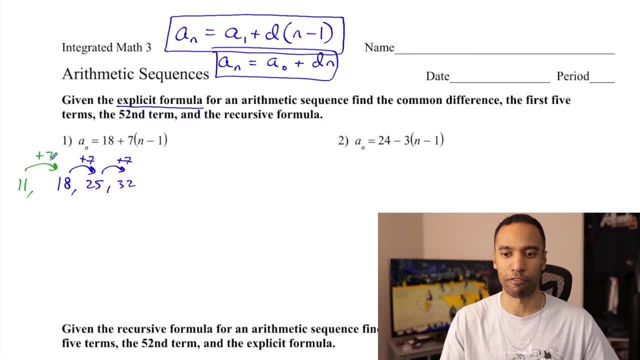 7 units before, like this. And says to find the value of the first term, you add 7 once. To find the value of the second term, you add 7 twice. Kind of a neat little way to do it. The way that our school is teaching it, our department and such, is mostly with the a sub 1 and the n minus 1 right here. But you can see either the idea of an explicit rule, and I know I haven't started. This is just me teaching it to begin with. 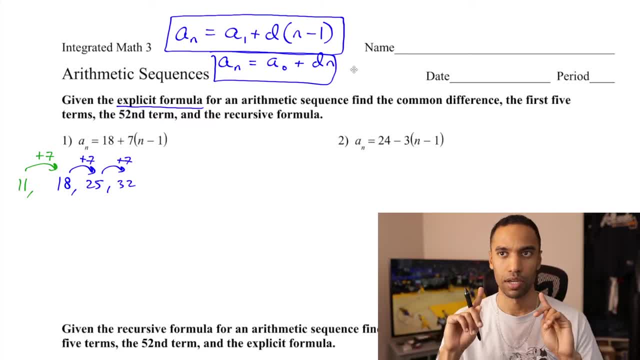 The idea of an explicit rule, though, is that you do substitute your position, 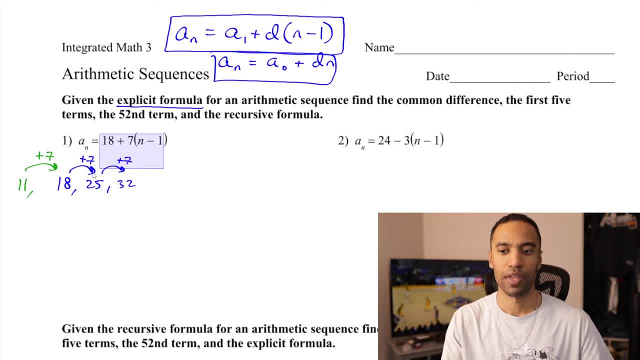 the n, into your equation to find the values. And we're going to go ahead and do that right here. And I actually just came up with some values for you, but we'll go ahead and restart. 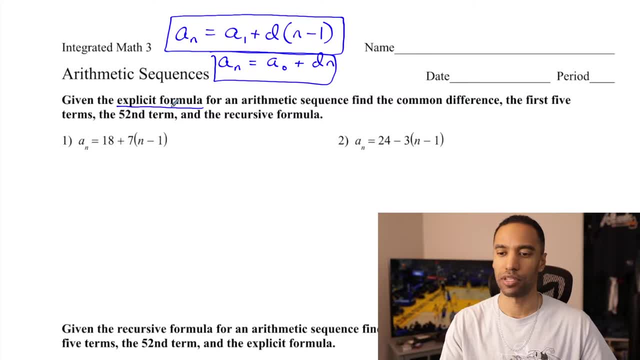 Given the explicit formula for the sequence, find the common difference, the first 5 terms, the 52nd term, very specifically, and the recursive formula, which I'll get into next. 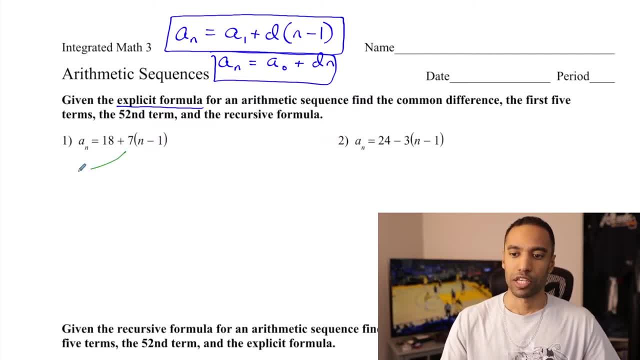 Let's start with the common difference. 7 ends up actually representing the common difference here. That is d. Either by non-reference, knowledge of the formula itself, that that's d right here, which stands for common difference, or understanding that that is the number that you're adding over and over as you increase your term position. 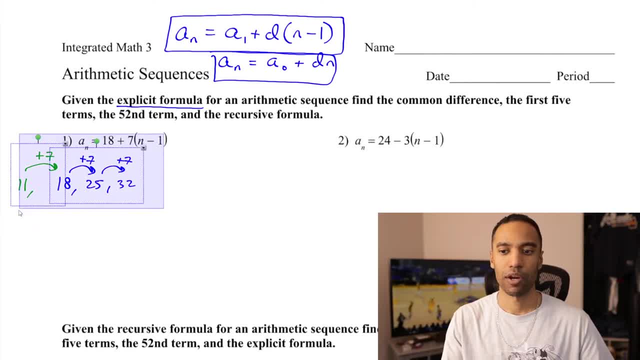 the n into your equation to find values, And we're going to go ahead and do that right here And I actually just came up with some values for you, but we'll go ahead and restart, Given the explicit formula for the sequence: find the common difference. 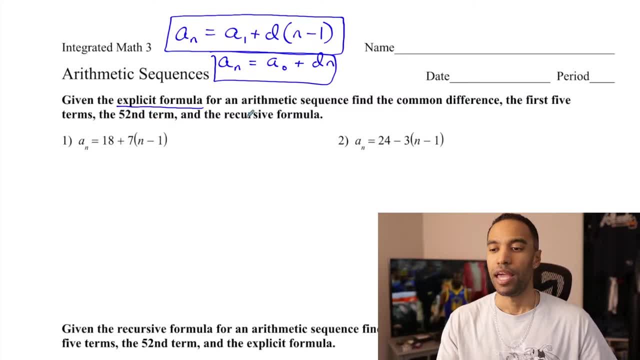 the first five terms, the 52nd term, very specifically, and the recursive formula, which I'll get into next. Let's start with the common difference. Seven ends up actually representing the common difference here, That is, d, either by knowledge of the formula. 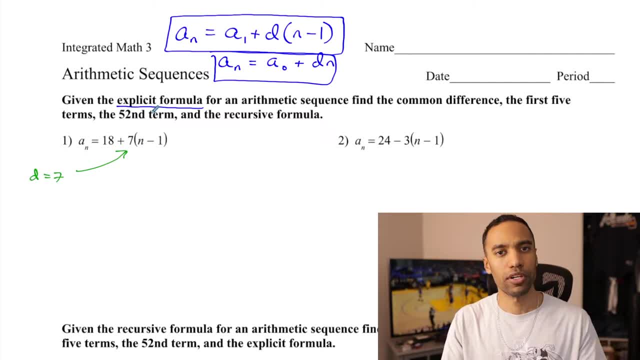 the formula itself, that that's d right here, which stands for common difference, or understanding that that is the number that you're adding over and over as you increase your term position. As you increase n by one, you're multiplying seven by one larger number. 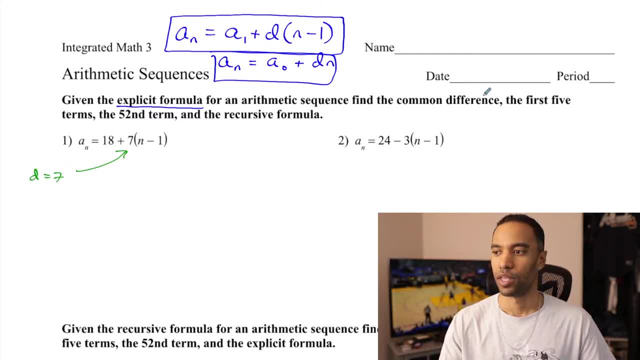 So you're adding one more seven. That makes that your common difference. Find the first five terms Now, a literal way we can do it, through the explicit rule once more, is that knowledge of the first term is by substituting one- excuse me, one- in for n. 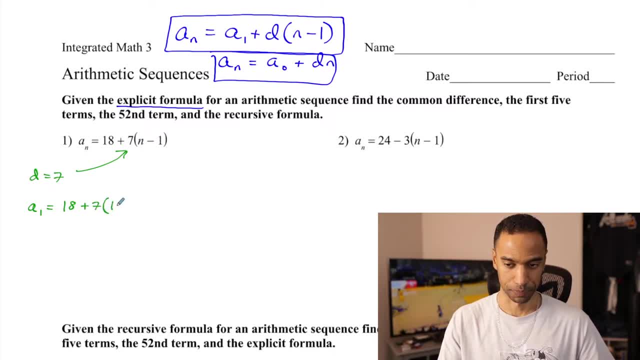 So that's 18 plus seven times minus one, which is 18.. I already know I probably got to drink water in a second: 18 plus seven times zero, which is 18 plus zero, which is 18.. That's a heck of a lot of even just mundane work to get that one in. 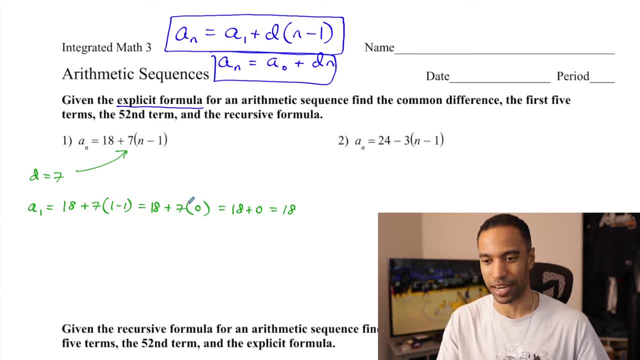 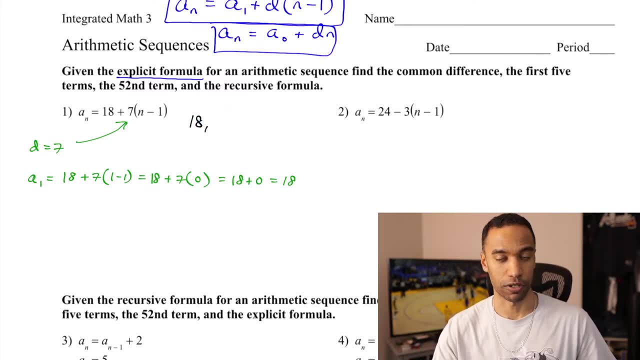 Obviously we could have saved ourselves a lot of steps on that thing. We probably didn't have to do all that. But you're substituting one for n to get your value. So 18 is the value of your first term in the sequence. 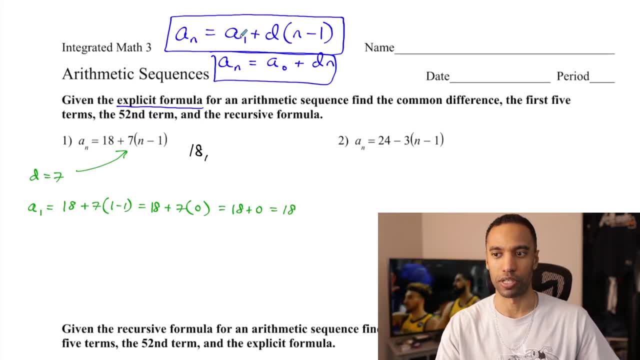 We already mentioned that before And you actually can realize that by the formula saying it's a sub one. But let's say you didn't know the formula, Let's say it wasn't of this variety. You substitute one for n. Now you substitute two for n. 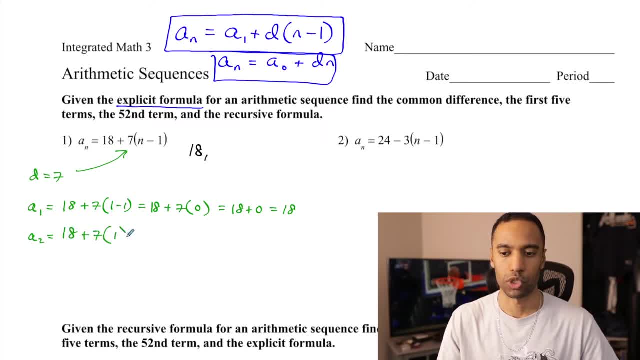 That's 18 plus seven times two minus one, which is one Seven times one is seven, And 18 plus seven is 25.. So you see that 25 is the next term in the sequence. A sub three is 18 plus seven times three minus one or two. 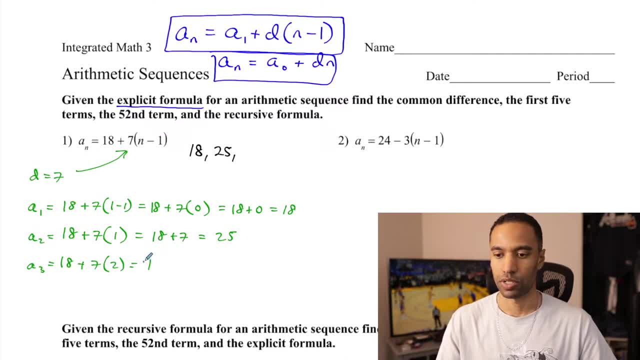 which is 18 plus 18 plus 14, which is 32.. So you can see how that one's 32.. And if you recognize enough through an arithmetic sequence that separates by a common difference, such as seven, you can recognize that as you're setting. 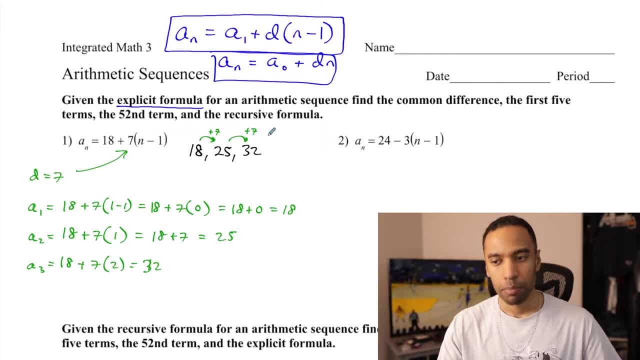 as you're adding seven over and over here, it appears that you could continue forward and say: what if we do plus seven again, We would get 39. Is that? is that a sub four? Was a sub four equal to 18 plus seven times four minus one or three? 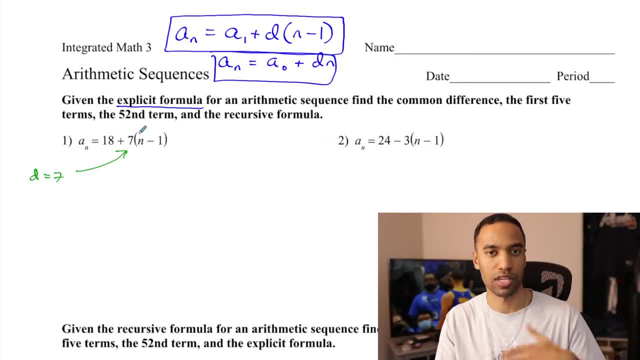 As you increase n by 1, you're multiplying 7 by one larger number. So you're adding one more 7. 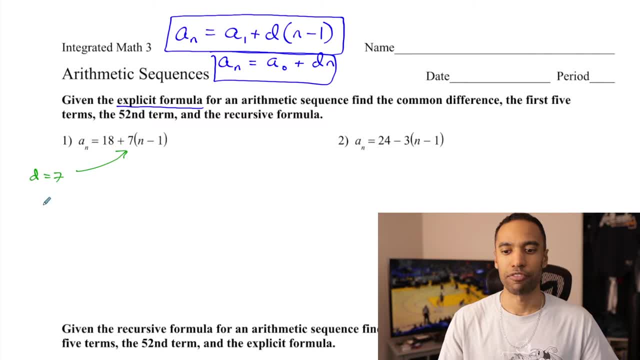 That makes that your common difference. Find the first 5 terms. 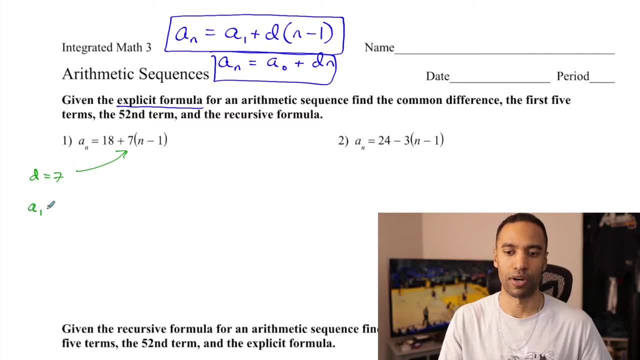 Now, a literal way we can do it through the explicit rule once more is that knowledge of the first term is by substituting 1, excuse me, 1 in for n. So that's 18 plus 7 times 1. 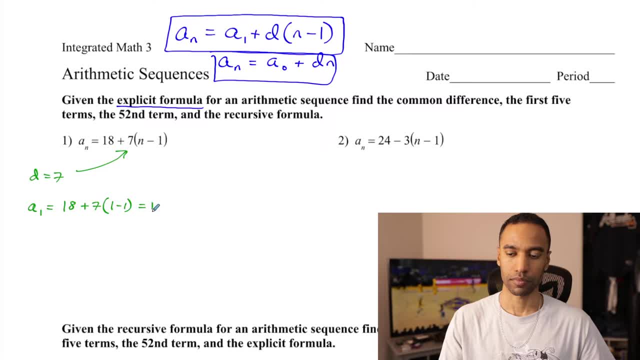 1 minus 1, which is 18. I already know I probably got to drink water in a second. 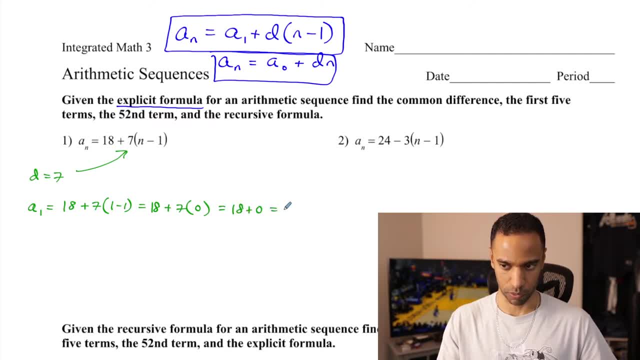 18 plus 7 times 0, which is 18 plus 0, which is 18. 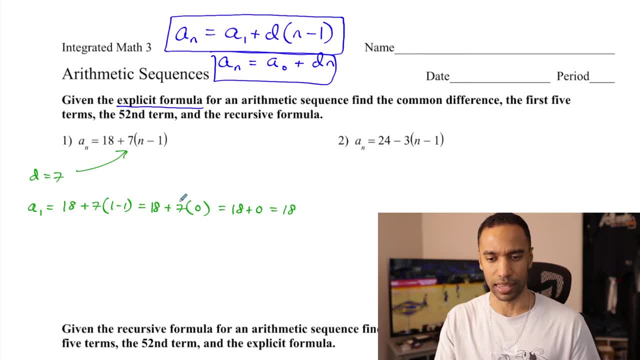 That's a heck of a lot of even just mundane work to get that 1 in. Obviously, we could have saved ourselves a lot of steps on that thing. We probably didn't have to do all that. 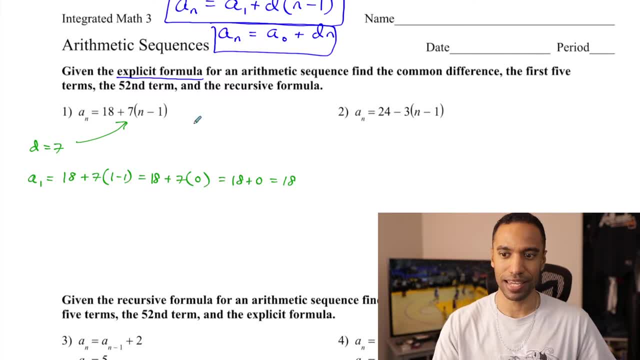 But you're substituting 1 for n to get your value. So 18 is the value of your first term in the sequence. 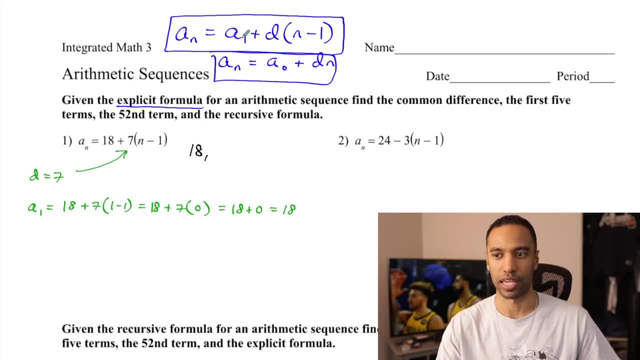 We already mentioned that before. And you actually can realize that by the formula saying it's a sub 1. 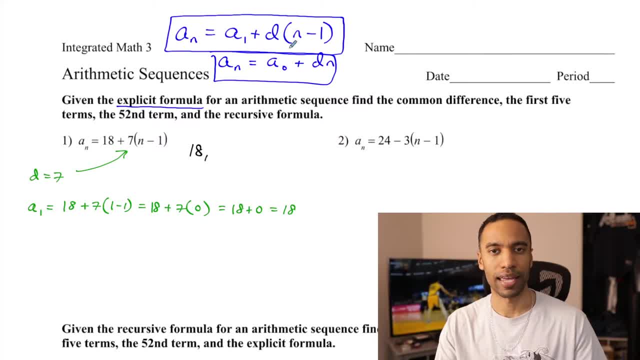 But let's say you didn't know the formula. Let's say it wasn't of this variety. You substitute 1 for n. Now, you substitute 2 for n. That's 18 plus 7 times 2 minus 1, which is 1. 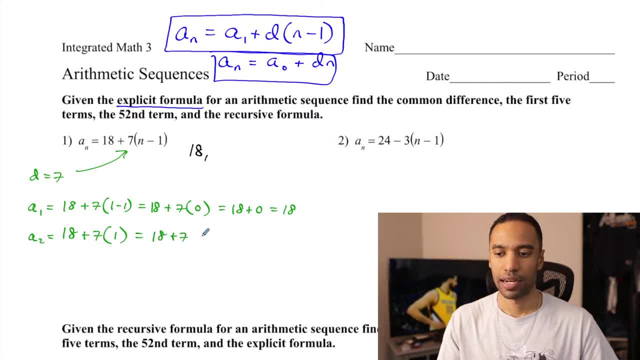 7 times 1 is 7. And 18 plus 7 is 25. So you see that 25 is the next term in the sequence. a sub 3 is 18 plus 7 times 3 minus 1, or 2. Which is 18 plus 14, which is 32. So you can see how that one's 32. And if you recognize enough through an arithmetic sequence that separates by a common difference, such as 7, you can recognize that as you're adding 7 over and over here, it appears that you could continue forward and say, what if we do plus 7 again? We would get 39. 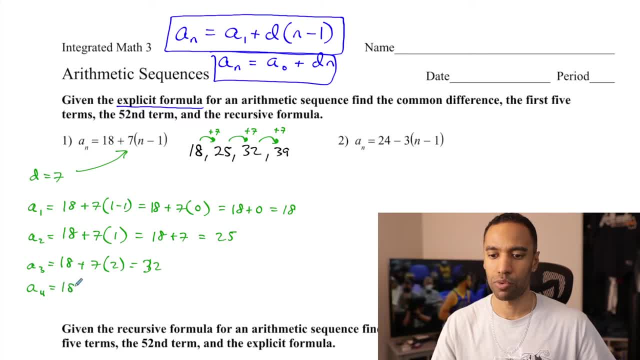 Is that a sub 4? Was a sub 4 equal to 18 plus 7 times 4 minus 1? 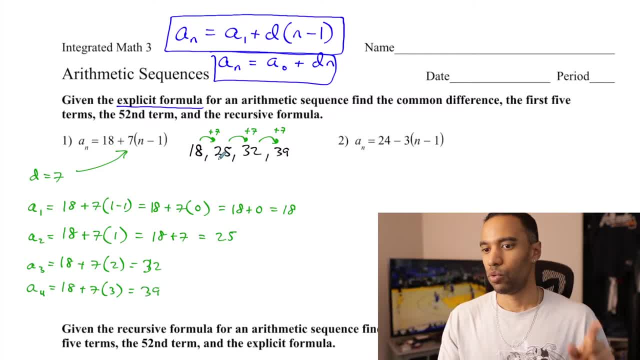 18 plus 21, 39?? Yes, it was. What I'm showing you. actually, right now is a matter of what's called recursion. Recursion is taking the previous value or values to potentially obtain future values. An explicit rule used the terms position. 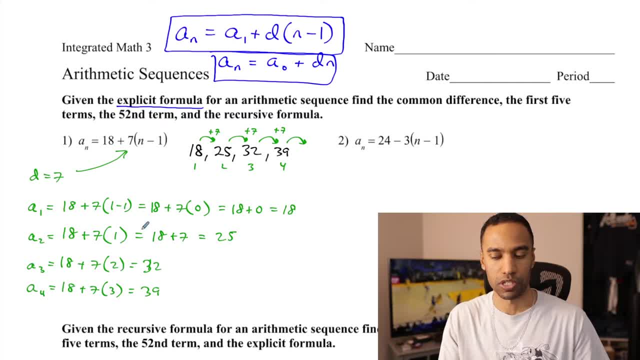 the first position, the second position, the third- Remember, I'm plugging those numbers into this equation- And a recursive rule says: let's take that 39 and add seven to it. What are we going to get? And that's 46.. 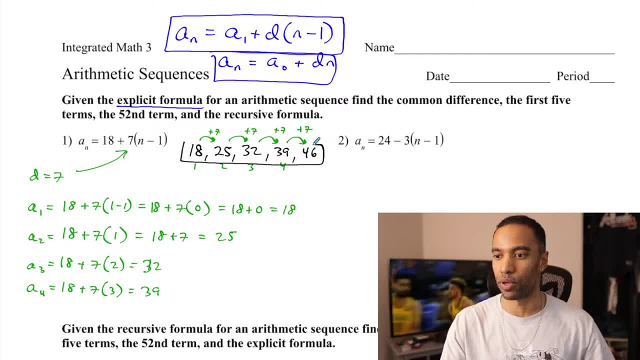 And honestly, that's how most people tend to come up with these or think about what the rule is. If I said what's happening in the sequence, you wouldn't say: oh you're, you know you're. you're 18 plus seven times that, minus one. 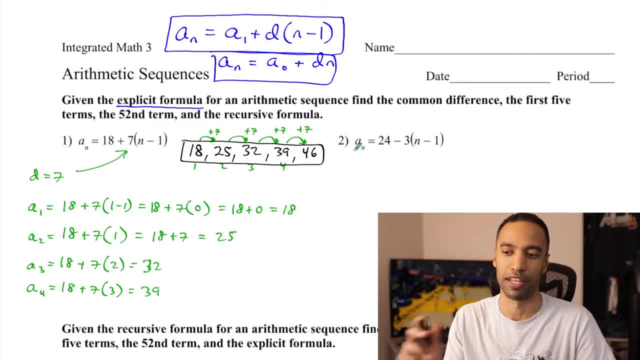 You know you're not doing that. You're saying: add seven, add seven each time, add seven each time, And that's what you're doing. And that's actually what a recursive formula has to do with which we'll dive into. 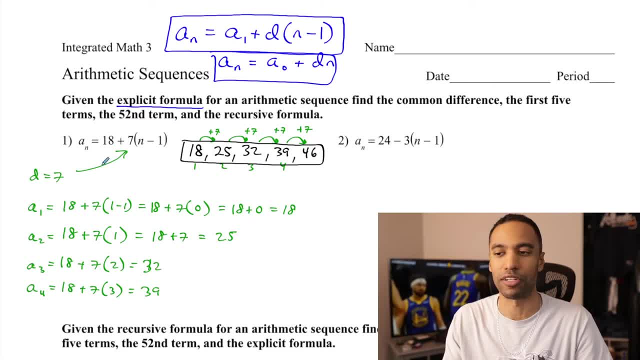 I just want to let you know that. But yeah, a sub five, you would plug five into there and you get it. You'll see me more often do the plus seven thing, because if you have the formula then you understand what's going on in the process. 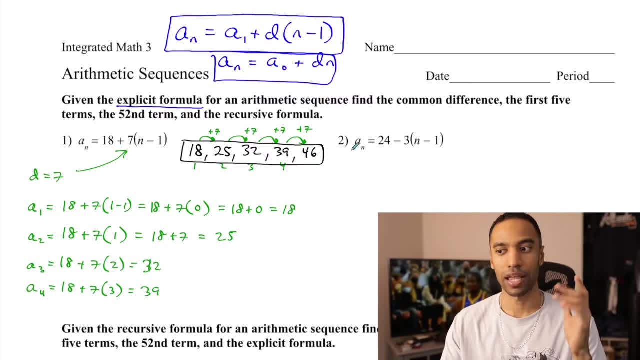 But if you don't have this formula or this one, and if it doesn't match the formula, then you're going to have to have a different means, which is plug them in. Let's find the 52nd term Now a recursive formula. before was really good. 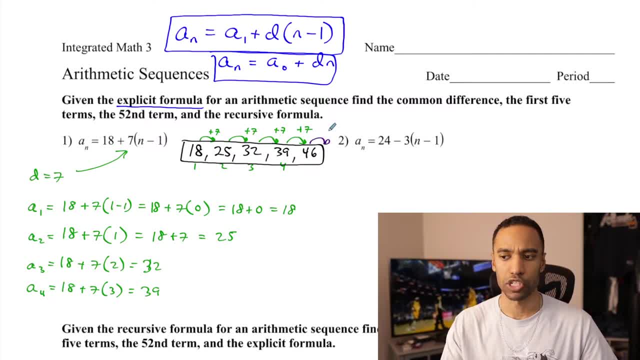 for just saying add seven, add seven, add seven. But would I want to just keep doing plus seven and figure out all my numbers 52 times or 51 times, you know, up to the 52nd term? Not necessarily, No, I'd rather work on the explicit formula. 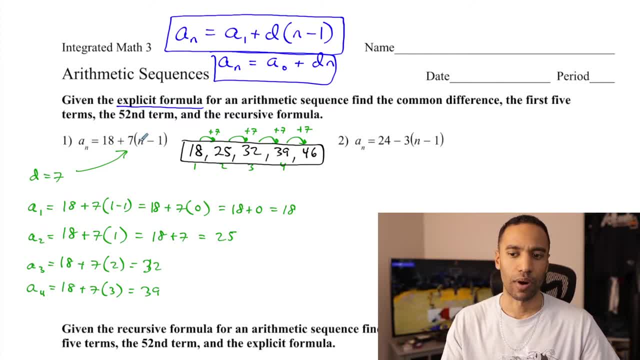 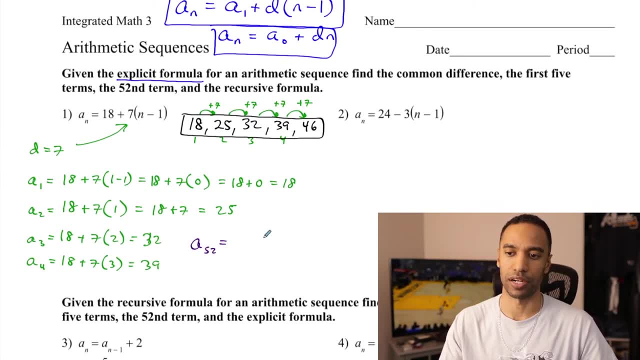 See, I could substitute 52 in for N right here, And I'm going to calculate that number. This is something that the explicit formula is really good for. So a sub 52 here is going to be 18 plus seven times 52 minus one. 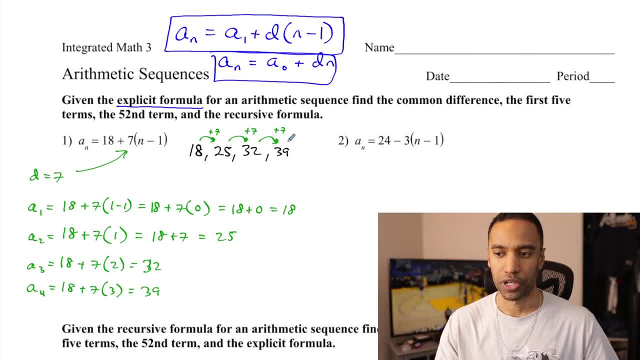 What I'm showing you actually right now is a matter of what's called recursion. Recursion is taking the previous value or values to potentially obtain future values. An explicit rule used the terms position. The first position, the second position, the third. 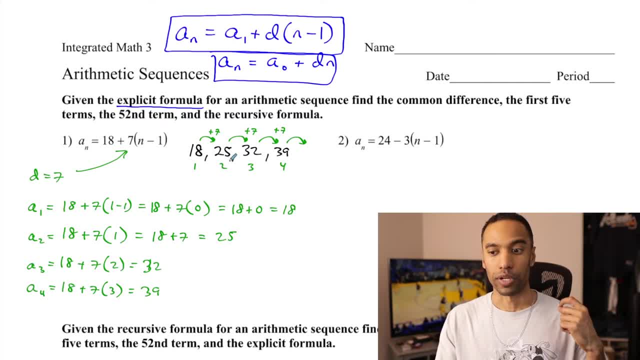 Remember, I'm plugging those numbers into this equation. And a recursive rule says, let's take that 39 and add 7 to it. What are we going to get? And that's 46. 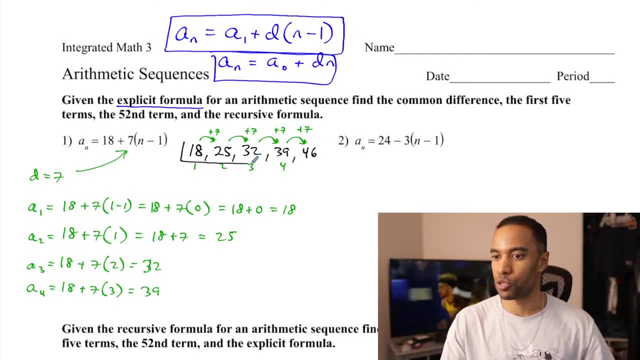 And honestly, that's how most people tend to come up with these or think about what the rule is. If I said what's happening in the sequence, you wouldn't say, oh, you're 18 plus 7 times that minus 1. You're not doing that. You're saying add 7, add 7 each time, add 7 each time. And that's what you're doing. 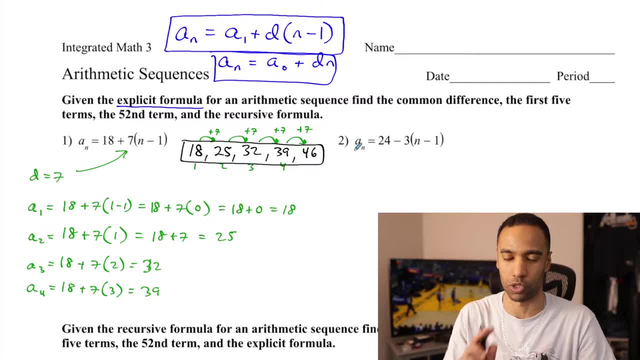 And that's actually what a recursive formula has to do with, which we'll dive into. I just want to let you know that. 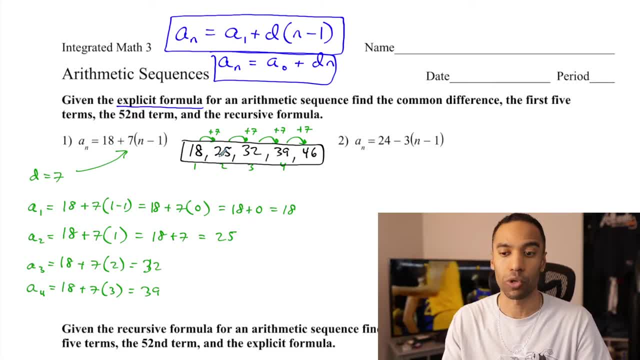 But yeah, a sub 5, you would plug 5 into there and you get it. You'll see me more often do the plus 7 thing because if you have the formula, then you understand what's going on in the process. But if you don't have this formula or this one, and if it doesn't match the formula, then you're going to have to have a different means, which is plug them in. Let's find the 52nd term. Now, a recursive formula before was really good for just saying add 7, add 7, add 7. 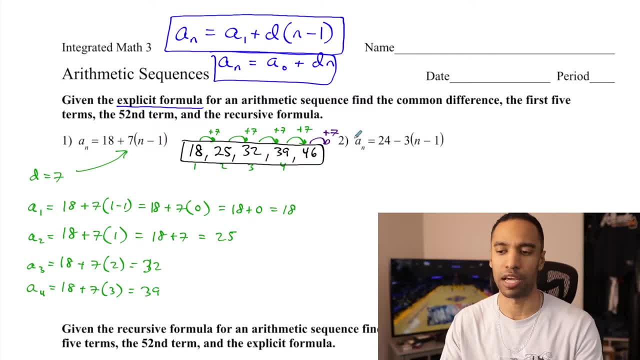 But would I want to just keep doing plus 7 and figure out all my numbers 52 times or 51 times, you know, up to the 52nd term? Not necessarily. 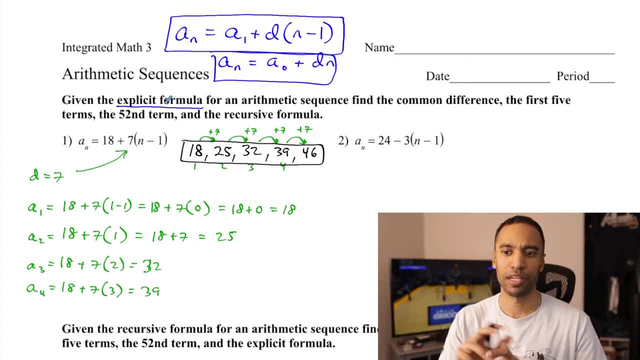 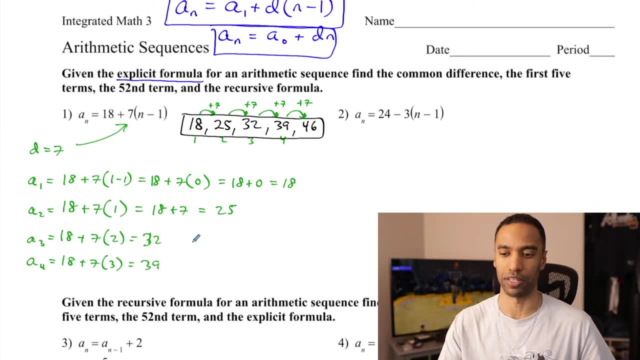 No, I'd rather work on the explicit formula. See, I could substitute 52 in for n. Right here, I'm going to calculate that number. This is something that the explicit formula is really good for. So a sub 52 here is going to be 18 plus 7 times 52 minus 1 or 51 here. I have a calculator on the side here, but I believe 7 times 51 is 357 plus 18 should be 375. 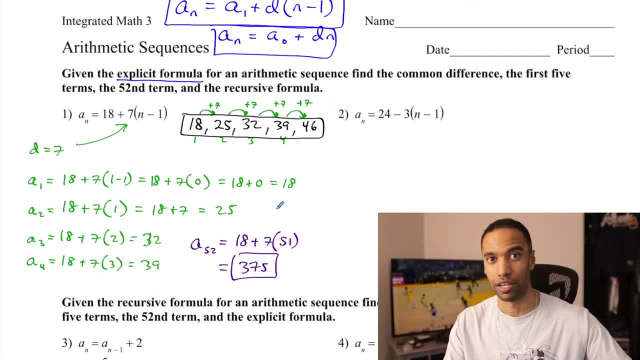 If I make a mistake, I do apologize, especially when I have a calculator handy on my phone right here. Okay, so I believe it's going to be 375. 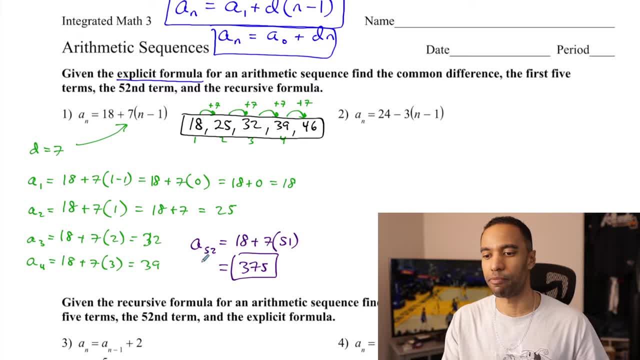 Yeah, so that's a sub 52. That is the value of the 52nd term. 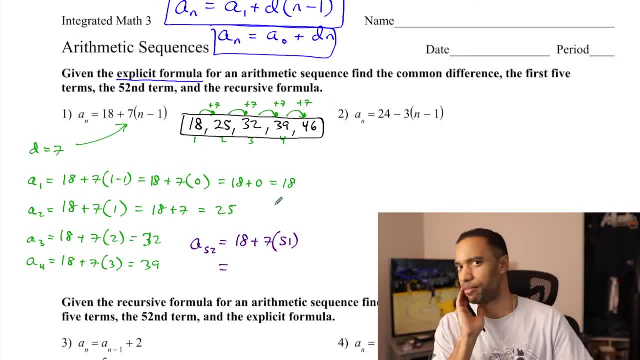 or 51 here. I have a calculator on the side here, but I believe seven times 51 is 357. plus 18 should be 375.. If I make a mistake I do apologize, especially when I have a calculator handy on my phone right here. 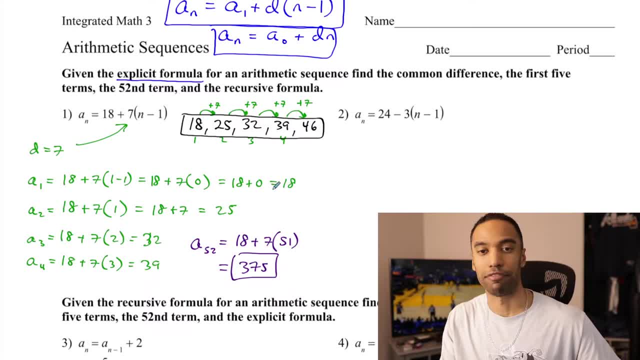 Okay, so I believe it's going to be 375.. Yeah, so that's a sub 52.. That is the value of the 52nd term. The last thing we need here- as I'm limited on space- is the recursive formula. 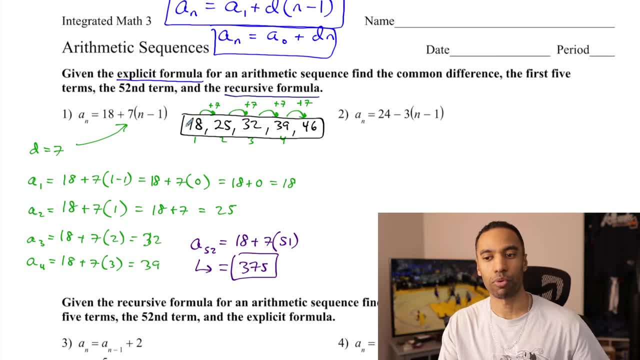 Now, recursion is what I stated before: taking previous values in order to get and obviously the common difference in order to get next values. So if I want to find the sixth term, I'm going to rely on the fifth term to do it. 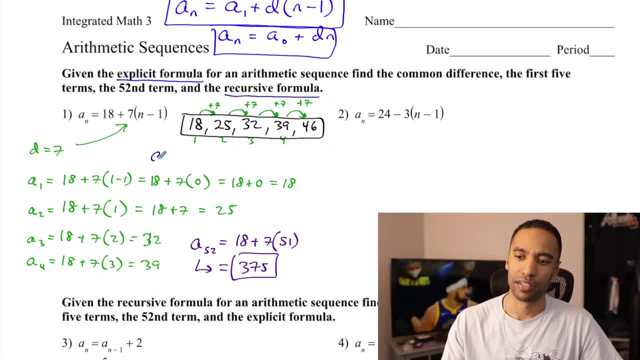 46 plus seven, et cetera. So if a sub N is in reference to- and I should really label everything that I'm doing here, but this is what I'm doing- This is going to be the recursive formula here with an R. 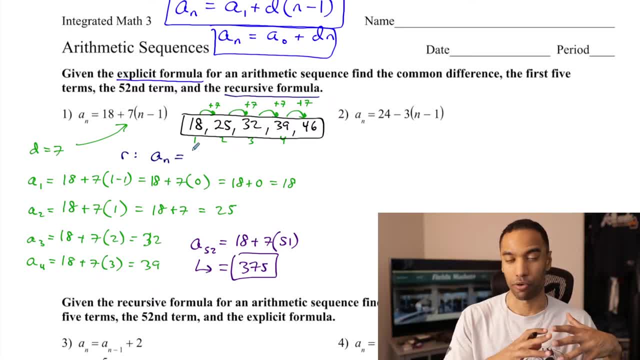 If a sub N references the value of the specific term I'm looking for, then a sub N minus one on the subscript refers to the value of the term before it. I'll show you what I mean when we do it in a second Now, plus your common difference. 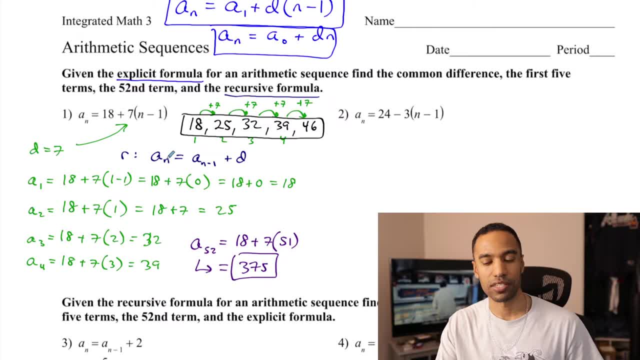 this is where we can get recursive formula. What this says is to find the value of a term. take the value of the term before it and add your common difference. In our case, our common difference is seven like that. Now there's another portion to recursive formulas. 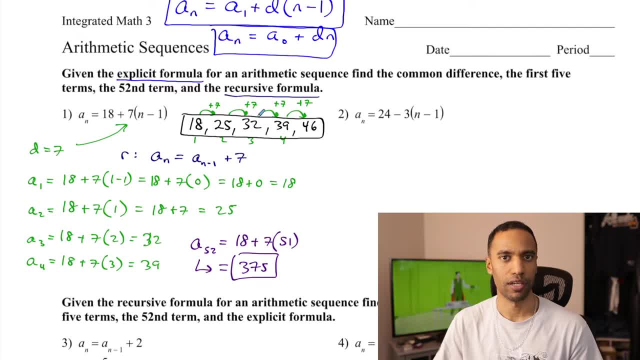 that's important for us, which is you have to mention a term specifically, So it's best to probably just mention the first term, as you have it provided even in the formula in and of itself, and say: a sub one is 18.. There are two portions to it. 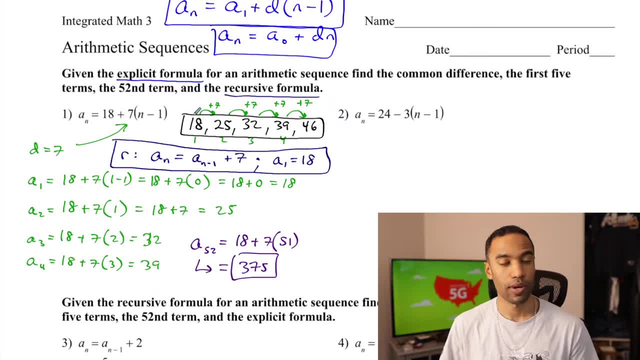 You do have to mention a term because otherwise if I just tell you to add seven over and over, you can't assume I meant from zero. You can't. There is no default assumption to anything there. We're starting from 18 and I have to mention that. 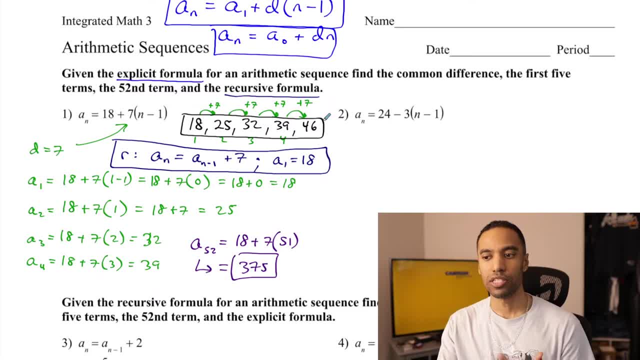 Starting from 18, add seven over and over. Let's see if it works. to get that fifth term that I never wrote out explicitly, I could say: if I want to find the value of a sub five, this 46,. if I wanted to find out 46 here. 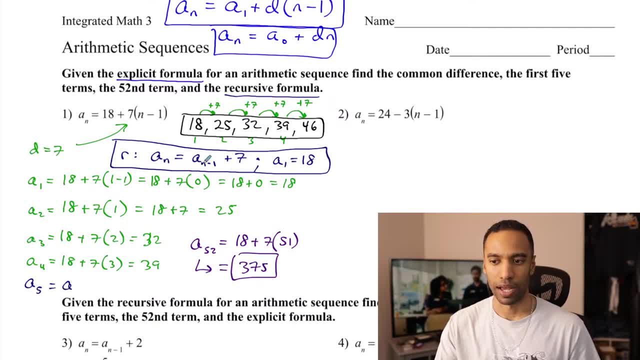 I would have to take a sub five minus one, that's a sub four, and add seven to it. Well, a sub four, we know, is 39.. So a sub five is 39 plus seven. You see where that goes in. 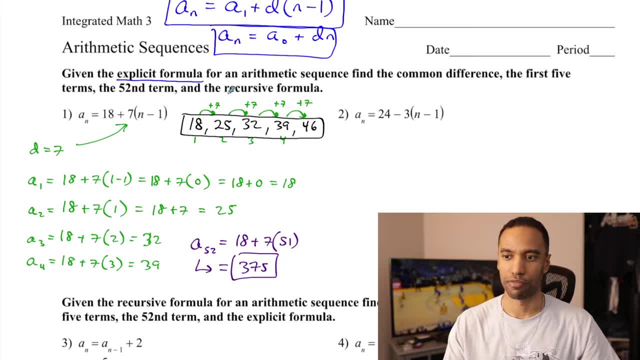 The last thing we need here, as I'm limited on space, is the recursive formula. Now, recursion is what I stated before, taking previous values in order to get, and obviously the common difference, in order to get next values. 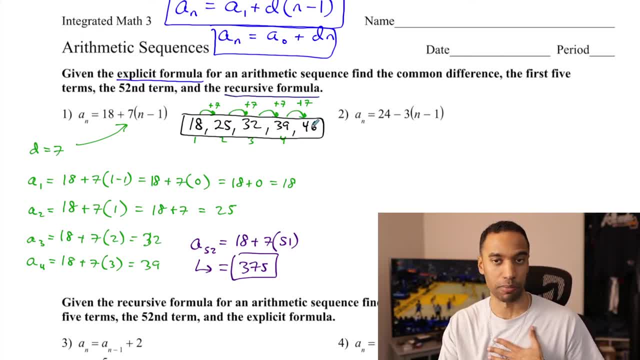 So if I want to find the 6th term, I'm going to rely on the 5th term to do it. 46 plus 7, et cetera. 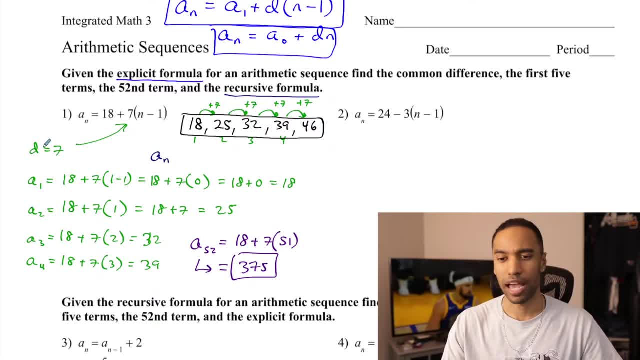 So if a sub n is in reference to, and I should really label everything that I'm doing, 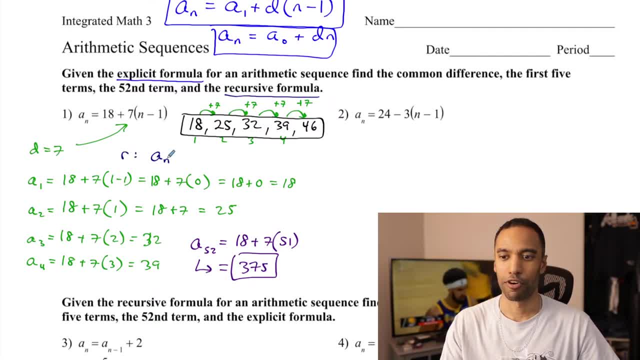 but this is going to be the recursive formula here, with an r. If a sub n references the value of the specific term I'm looking for, then a sub n minus 1, all in the subscript, refers to the value of the term before it. I'll show you what I mean when we do it in a second. Now, plus your common difference, this is where we can get recursive formula. What this says is, to find the value of a term, take the value of the term before it, and add your common difference. In our case, our common difference is 7. 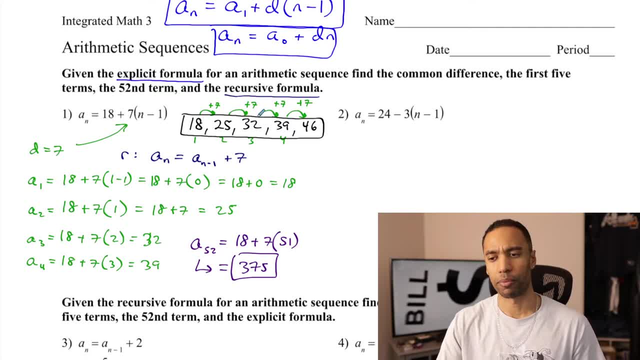 Like that. Now, there's another portion to recursive formulas that's important for us, which is you have to mention a term specifically. So it's best to probably just mention the first term, as you have it provided, even in the formula in and of itself, and say a sub 1 is 18. There are two portions to it. You do have to mention a term. Because otherwise, if I just tell you to add 7 over and over, you can't assume I meant from 0. You can't. There is no default assumption to anything there. 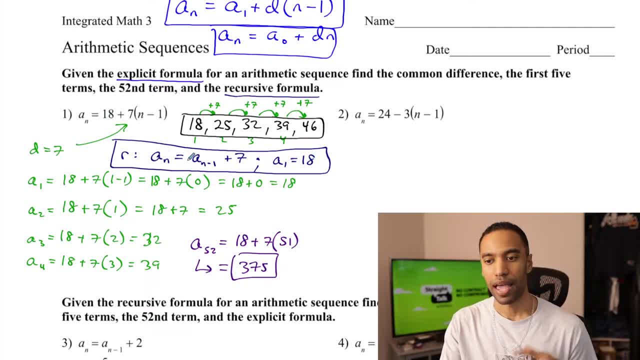 We're starting from 18, and I have to mention that. Starting from 18, add 7 over and over. 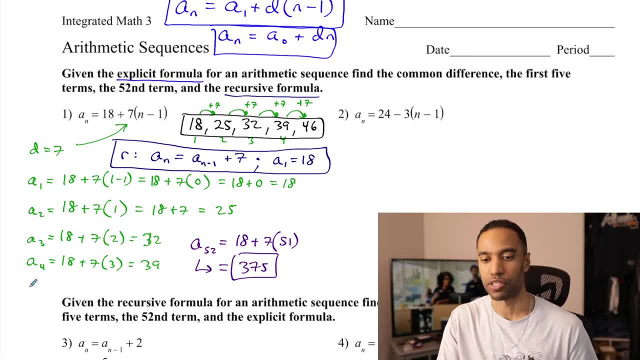 Let's see if it works to get that fifth term that I never wrote out explicitly. I could say, if I want to find the value of a sub 5, this 46, if I wanted to find out 46 here, I would have to take a sub 5 minus 1, that's a sub 4, and add 7 to it. 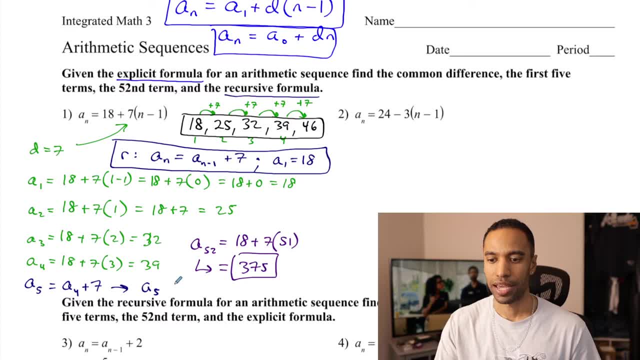 Well, a sub 4, we know, is 39. So a sub 5 is 39 plus 7. You see where that goes in? 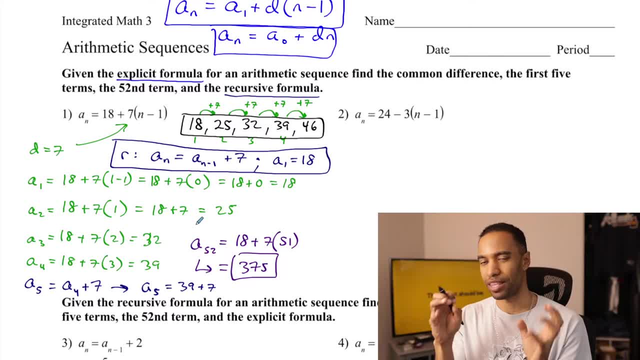 So that's, you know, you don't have to use the formula in the way, I mean, you do, but you don't have to write it out in that way to present it. But that is what's happening. That's what's happening in the formula. 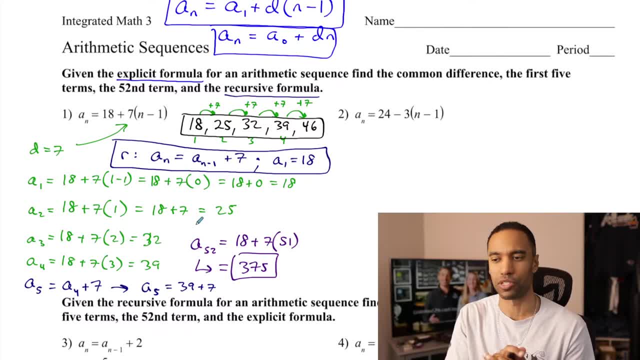 You can do a lot of different formulas to represent things. Fibonacci sequence is good through recursion. 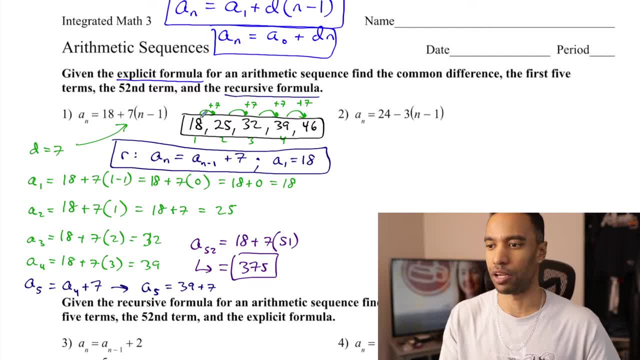 So they have their pros and cons, but that is both of them. And I spent a good long 11 minutes explaining all that, but it speeds things up in the end. 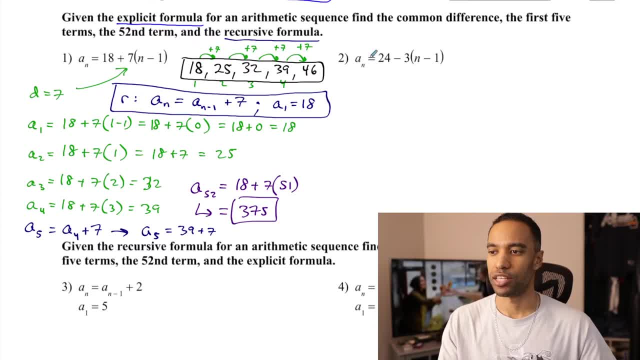 So let's keep moving forward into number 2. Number 2, a sub n equals 24 minus 3 times n minus 1. We are going to follow all the same things as before. Given this formula here, it is explicit. Let's find the common difference. I'm going to locate that one as d. 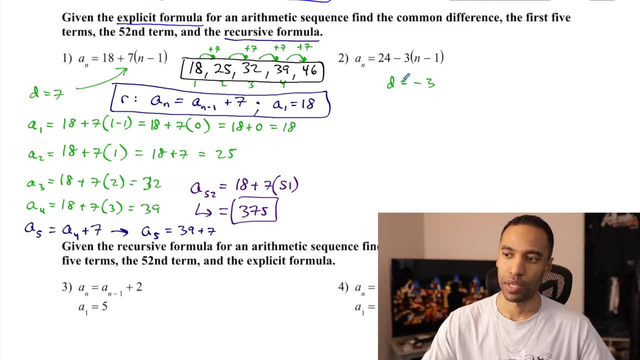 That d is, in this case, negative 3. You might notice we're subtracting 3 there, and we're adding a negative. So when I said we're adding the same number over and over, you could be subtracting as well. 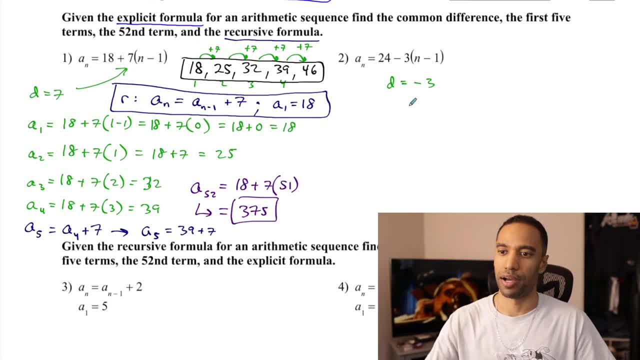 Sequences can decrease in this list. Now, the first five terms. 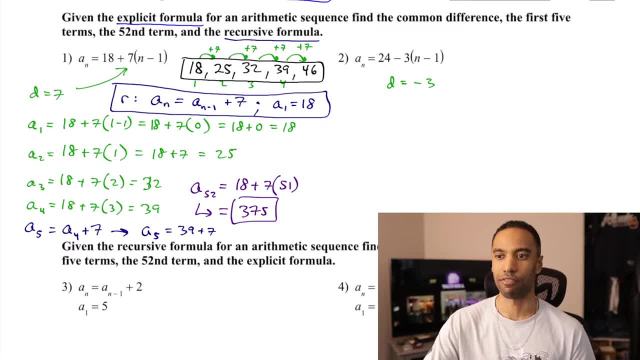 So I'm going to use the recursive path to get the first five terms for you. 24 is your first term. 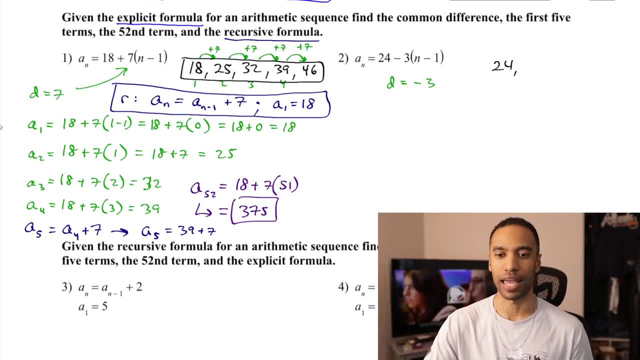 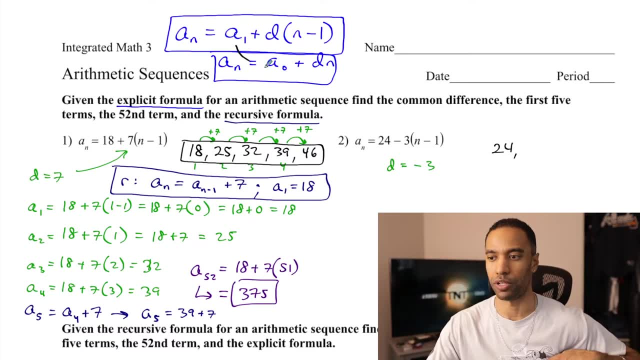 24 is your first term here. That is the a sub 1. And I know that for one of two reasons. You can make your choice. Either you recognize it is represented in this format here with a sub 1 clearly presented as 24, or if you'd like to substitute 1 into this equation, 1 minus 1 is 0, and this term goes away. 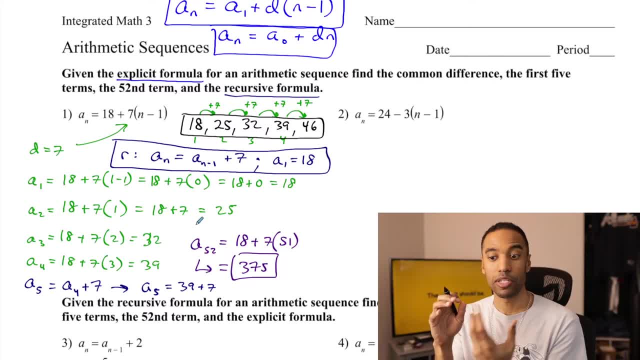 You don't have to use the formula in the way I mean you do, but you don't have to write it out in that way to present it. but that is what's happening. That's what's happening in the formula. You can do a lot of different formulas to represent things. 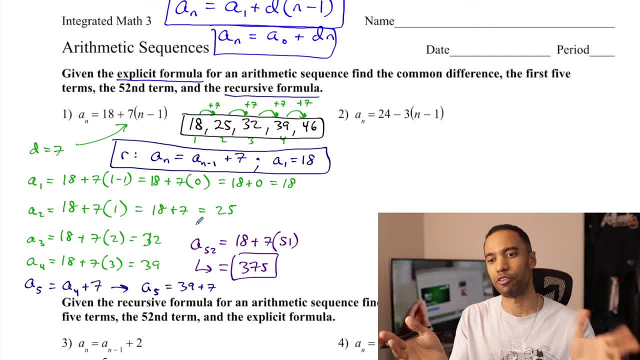 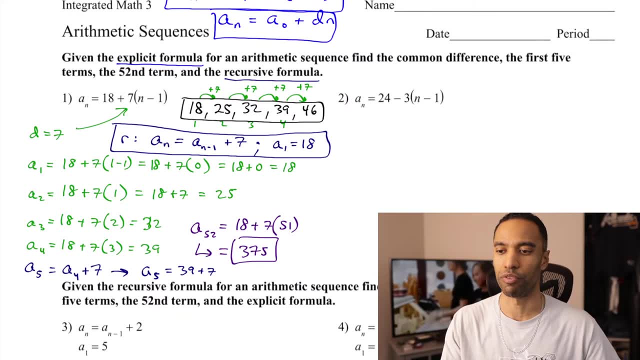 Fibonacci sequence is good through recursion, So they have their pros and cons, but that is both of them, And I spent a good long 11 minutes explaining all that, but it speeds things up in the end, So let's keep moving forward into number two. 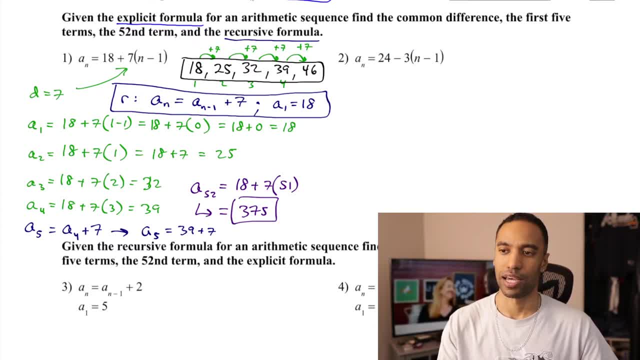 Number two, a sub n equals 24 minus three times n minus one. We're going to follow all the same things as before, Given this formula here it is explicit. Let's find the common difference. I'm going to locate that one as d. 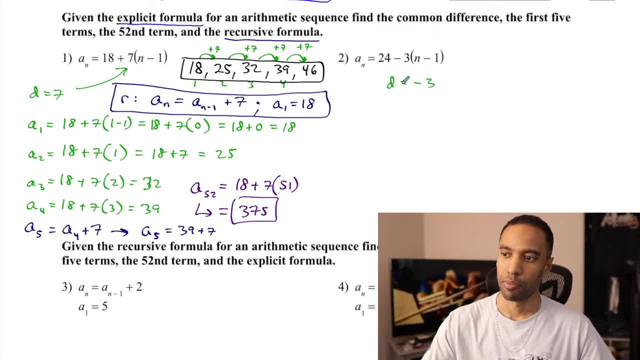 That d is in this case negative three. You might notice we're subtracting three there and we're adding a negative. So when I said we're adding the same number over and over, you could be subtracting as well. Sequences can decrease in this list. 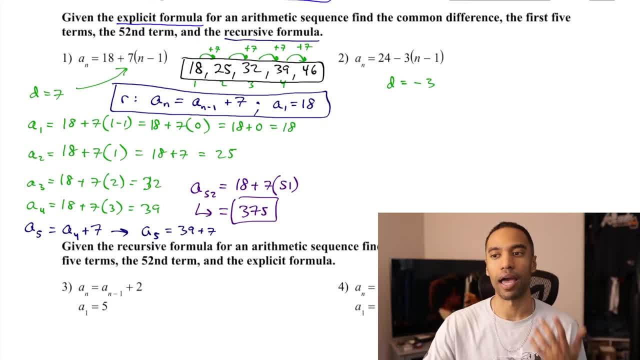 Now the first five terms. so I'm going to use the recursive path to get the first number, The first five terms for you. 24 is your first term. 24 is your first term here. That is the a sub one. 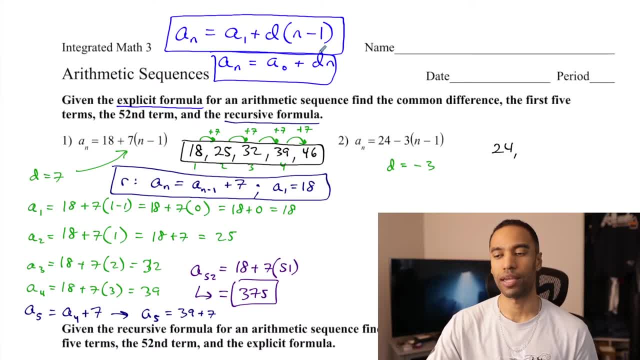 And I know that for one of two reasons you can make your choice. Either you recognize it is represented in this format here, with a sub one clearly presented as 24, or, if you'd like to substitute one into this equation, one minus one is zero. 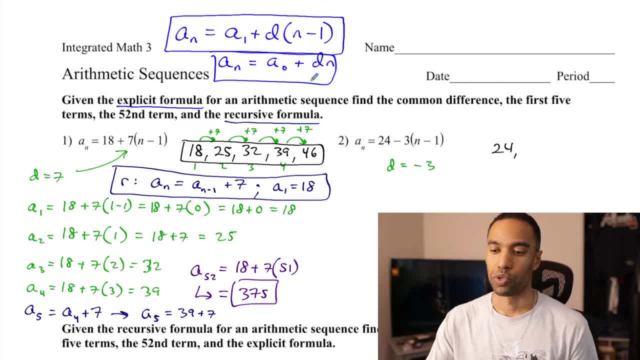 and this term goes away, That quantity completely goes away. Now, if negative three is your common difference, that means that you're subtracting three to get to the next term. So each time, for the first five terms, I will recursively subtract three from the previous value. 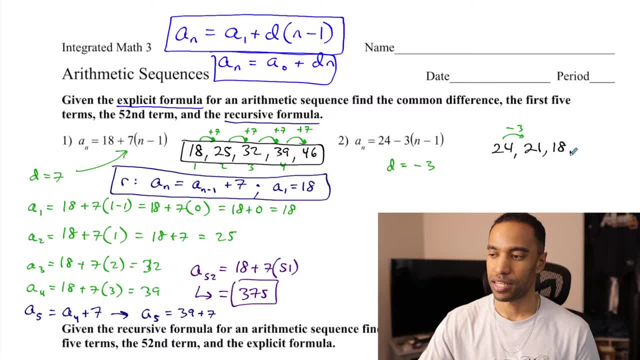 24 minus three is 21.. 21 minus three is 18.. 18 minus three is 15.. 15 minus three is 12.. This is your first five terms here. Now the 52nd term. I would very much like to use the explicit formula. 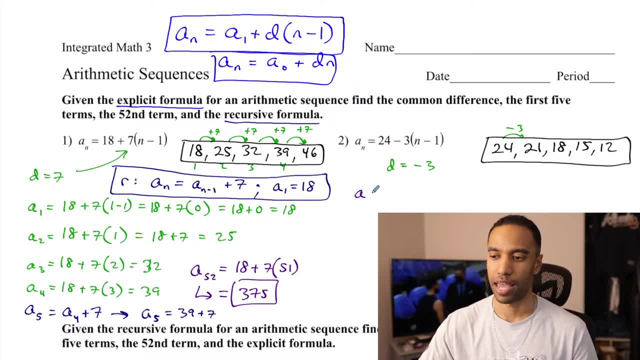 as I did before. So I'm going to go ahead and find out. hey, a sub 52 is 24. minus three times 52 minus one Again, that's going to be 51.. Three times 51 is 153.. 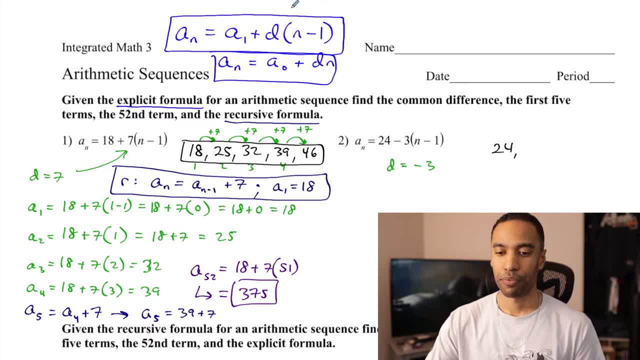 That quantity completely goes away. Now, if negative 3 is your common, that means that you're subtracting 3 to get to the next term. So each time, for the first five terms, I will recursively subtract 3 from the previous value. 24 minus 3 is 21. 21 minus 3 is 18. 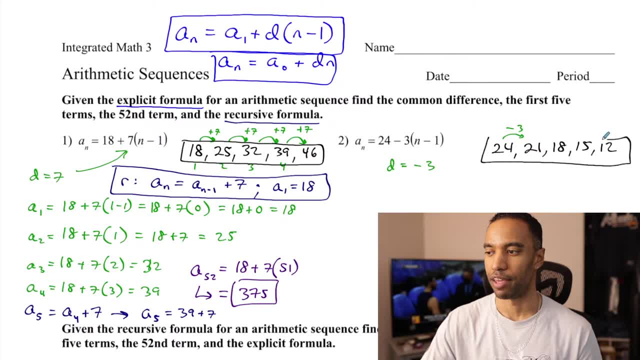 18 minus 3 is 15. 15 minus 3 is 12. This is your first five terms here. 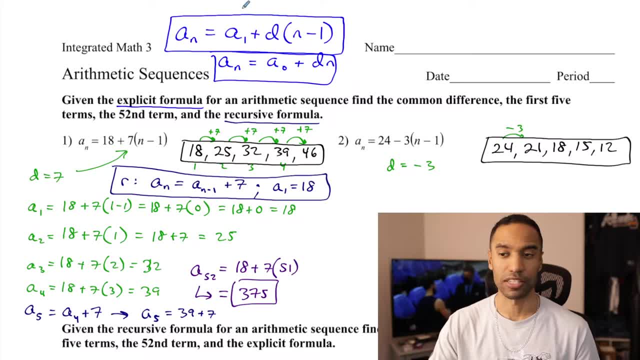 Now, the 52nd term, I would very much like to use the explicit formula as I did before. So I'm going to go ahead and find out, is 24 minus 3 times 52 minus 1. Again, that's going to be 51. 3 times 51 is 153. 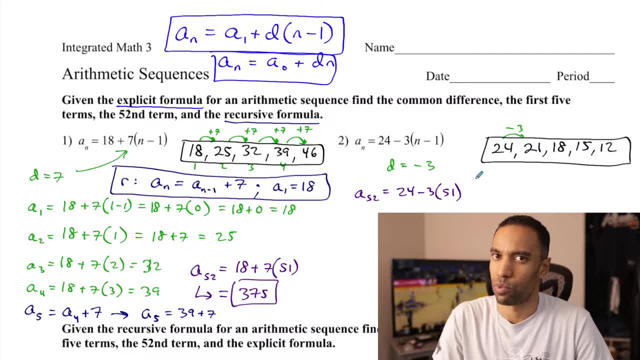 And 153 minus 24 is negative 129.. 24 minus 153, excuse me- is negative 129. And if I'm wrong I'm sorry. So that is negative 129.. And we'll go to the calculator Whoops when need be. 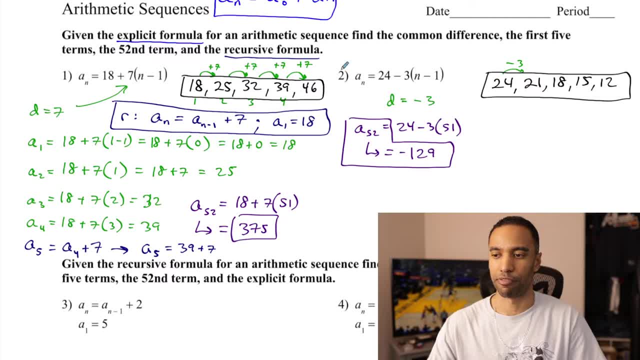 You'll definitely see me do that in time. All right, there's a sub 52.. And the last thing is the recursive formula, which, point blank one more time. we are going to say: to find the value of some term, you take the value of the term before it. 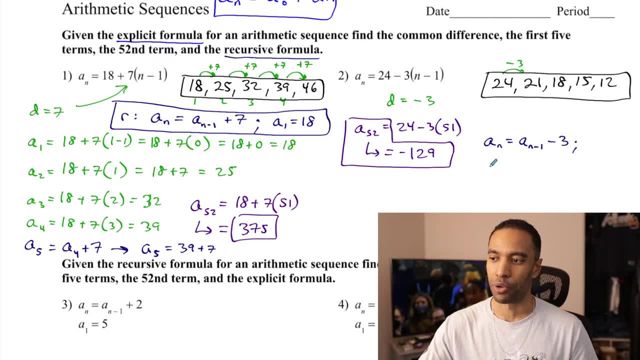 and we subtract three. And oh, by the way, the value of the first term is 24.. You do need both parts. Totally required This: a sub n equals a sub n minus. one thing is not going to change. Take the value of the term before it. 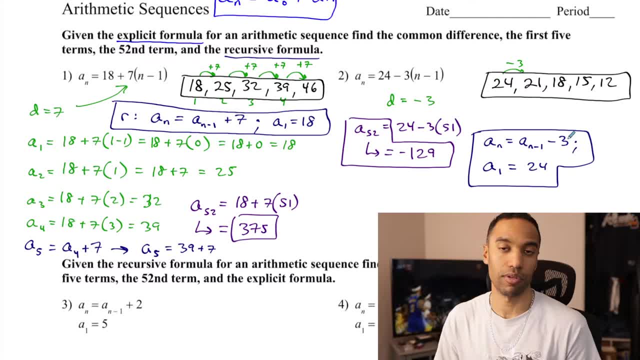 It's the common difference portion that's going to be applied. You'll see it when we do geometric sequences as well, And I'm going to assume, when I do my geometric sequence video, that you've seen this to make sense of what explicit rule means. 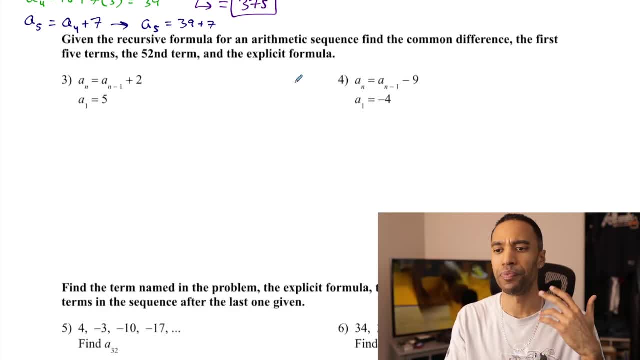 And what recursive rule means, The differences speaking of common ratio. And there are other instances. I'm going to talk a little bit about arithmetic sequences again. when we do the geometric sequences, All right, Given the recursive formula for an arithmetic sequence, 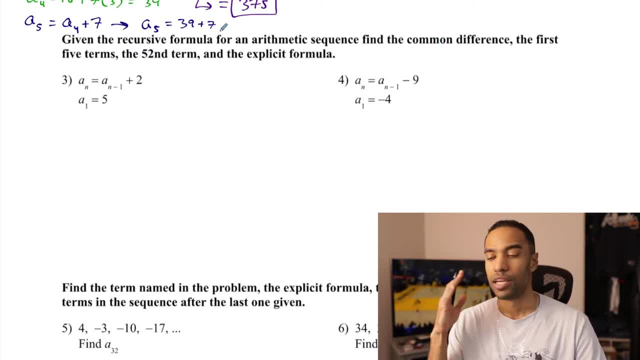 find the common difference. first, five terms, 52nd term and explicit formula: Same ish only from the other end. So you can notice here, excuse me, You can notice here that they use the same thing To find the value of some term. 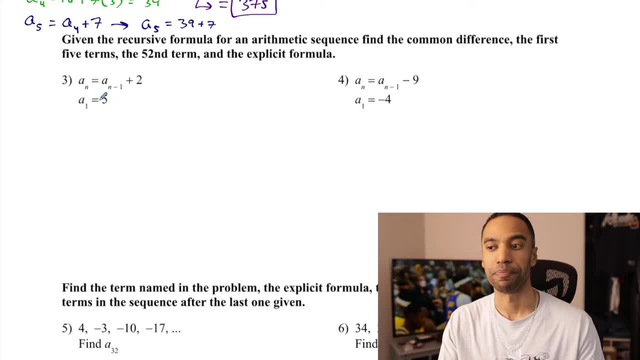 take the value of the term before it and add two, starting from five. So add two That you know. two is your common difference. That's going to be: D equals two. Every time we're going to add two from the previous set. 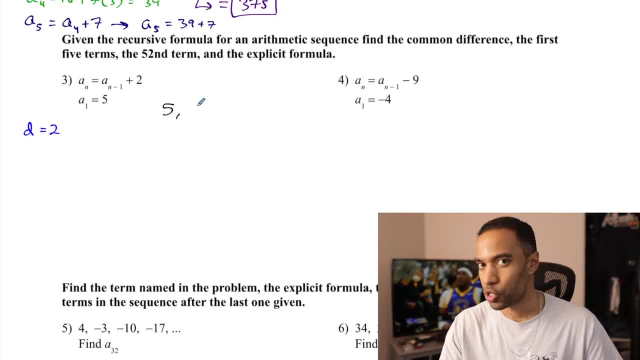 Your first five terms are five plus two. seven plus two is nine plus two is 11 plus two is 13.. There's your first five terms. Sorry if I kind of I'm not writing out where things go, but I've been kind of color coding the same way. 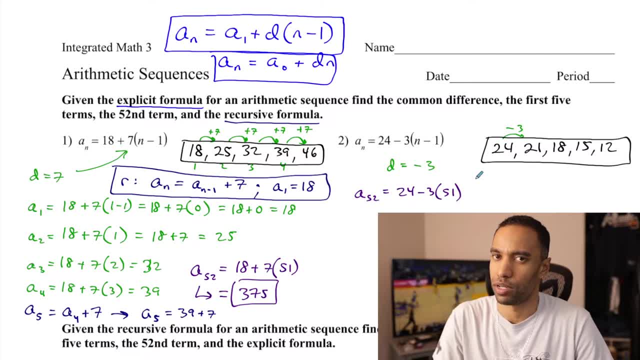 And 153 minus 24 is negative 129. 24 minus 153, excuse me, is negative 129. 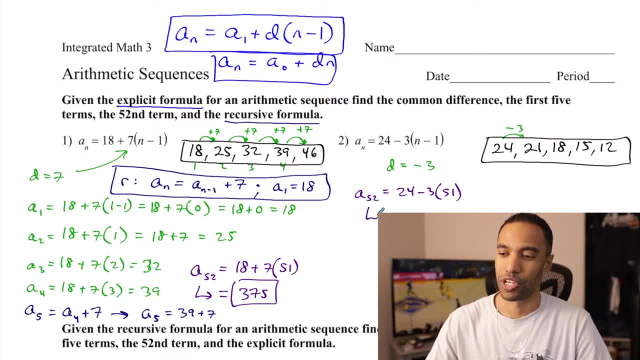 And if I'm wrong, I'm sorry. So that is negative 129. 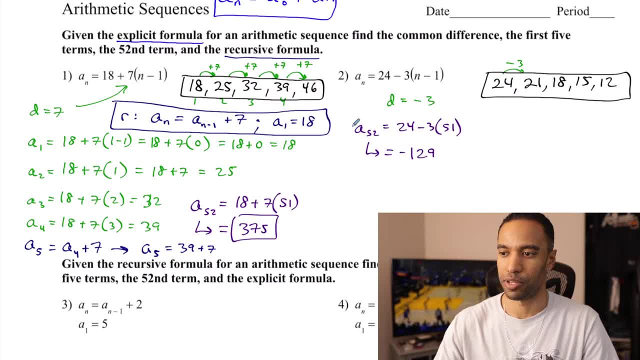 I will go to the calculator. Whoops, when need be. In time. 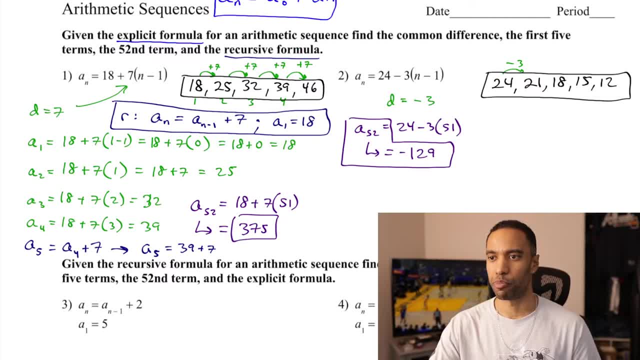 Alright, there's a sub 52. And the last thing is the recursive formula, which point blank one more time, we are going to say to find the value of some term, you take the value of the term before it, and we subtract 3. And oh, by the way, the value of the first term is 24. You do need both parts. 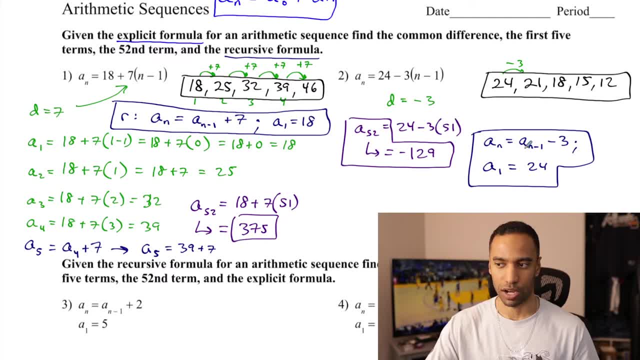 Totally required. This a sub n equals a sub n minus 1 thing is not going to change. 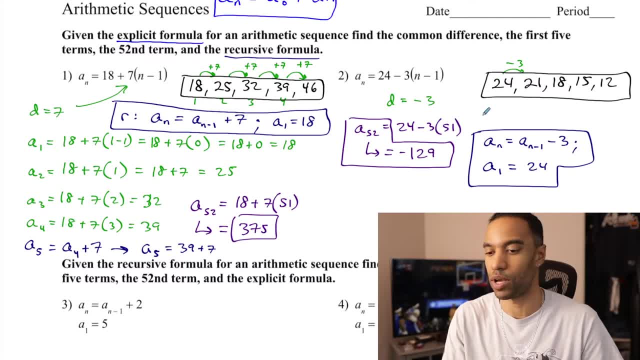 Take the value of the term before it. It's the common difference portion that's going to be applied. And I'm going to assume when I do my geometric sequence video that you've seen this to make sense of what 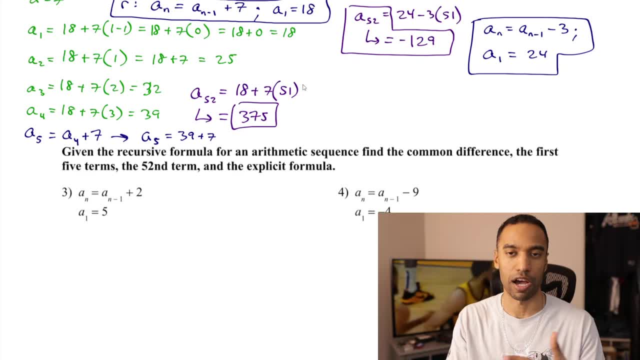 explicit rule means and what recursive rule means. The differences, speaking of common ratio. 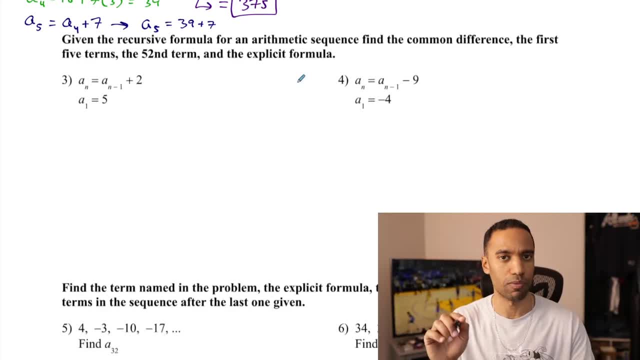 And there are other instances. I'm going to talk a little bit about arithmetic sequences again 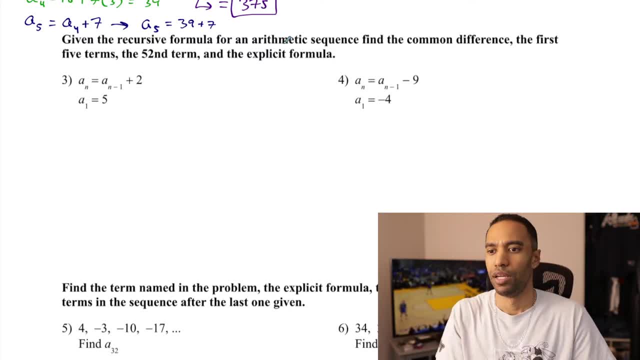 when we do the geometric sequences. Alright. Given the recursive formula for an arithmetic sequence, find the common difference first five terms, 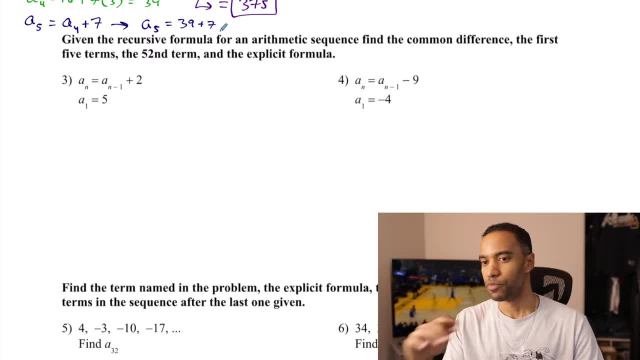 52nd term and explicit formula. Same ish, only from the other end. So you can notice here, excuse me, you can notice here that they use the same thing. 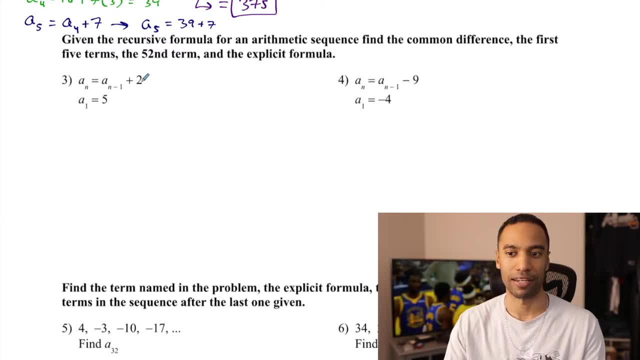 To find the value of some term, take the value of the term before it and add 2. Starting from 5. So, add 2. 2 is your common difference. That's going to be d equals 2. Every time we're going to add 2 from the previous set. Your first five terms are 5 plus 2 7 plus 2 is 9 plus 2 is 11 plus 2 is 13. 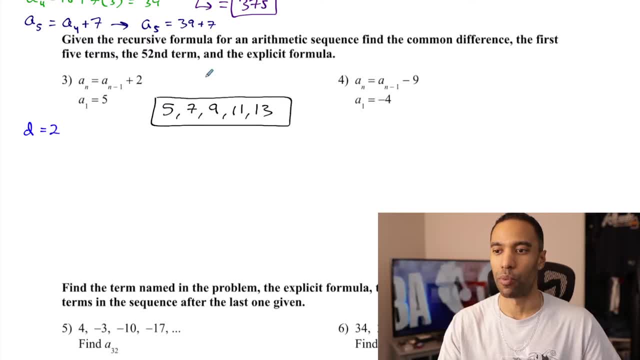 Those are your first five terms. Sorry if I'm not writing out where things go. 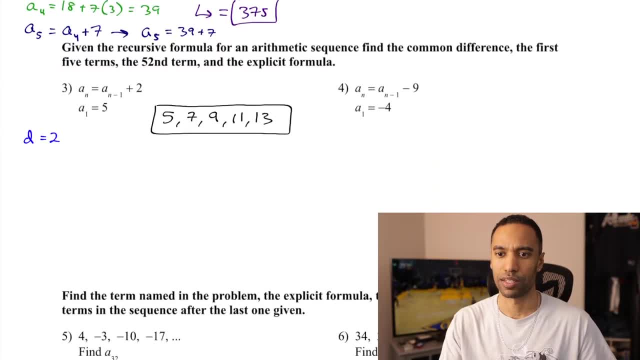 But I've been kind of color coding the same way for the most part. 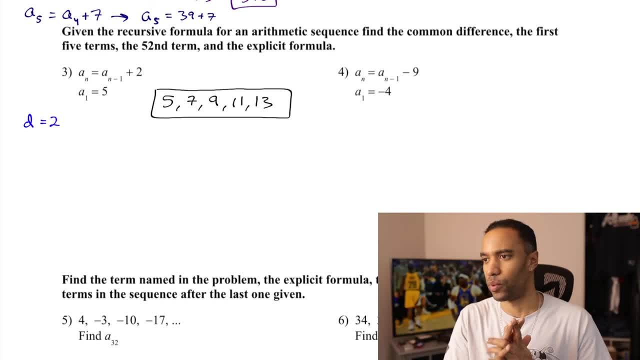 You can see that common difference there. Yeah, so that's where we're working that out. 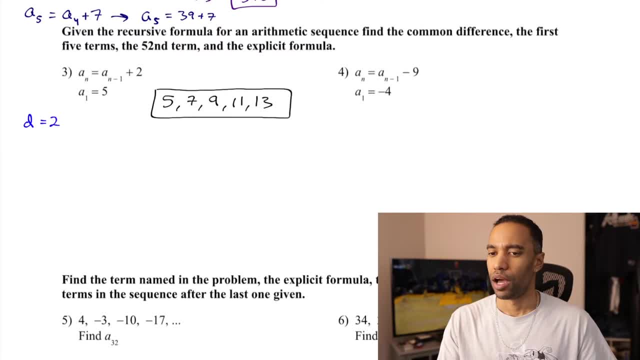 for the most part, Except for that common difference there. Yeah, so that's where we're working that out. Now, the 52nd term: that would be nice to get that explicit formula. So what you'd want to do is construct an equation. 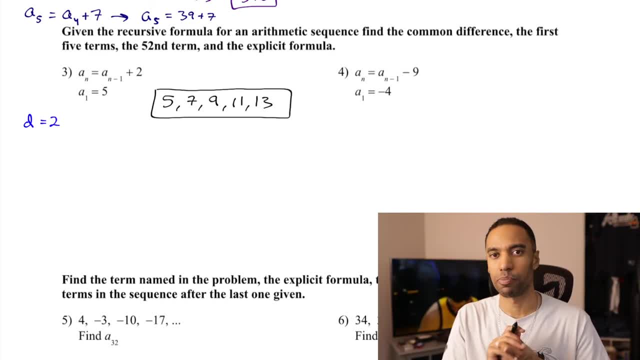 Now the 52nd term, that would be nice to get that explicit formula. So what you'd want to do is construct an equation out of what's presented 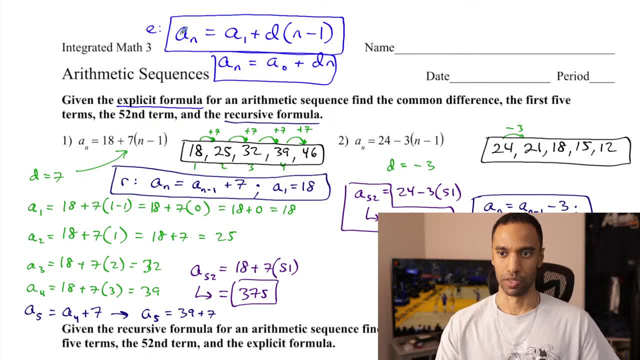 right here for the, let me put an e here. The explicit formula is presented as such. 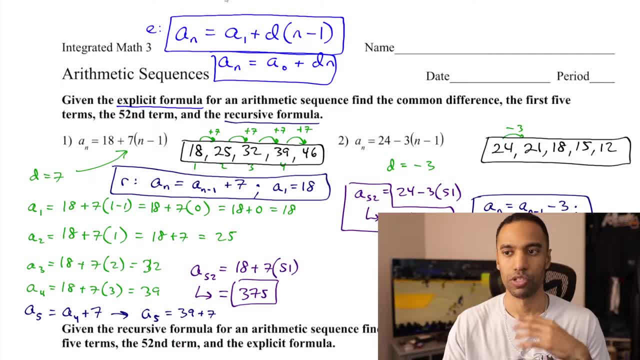 Use the first term, use the common difference to create it. We have to, you know, we have to do that anyway. 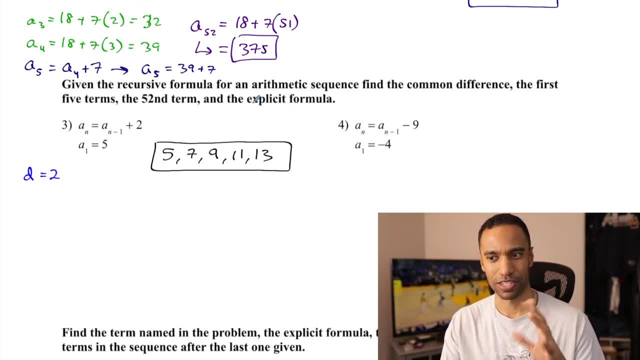 I'm not really a fan of the fact that this is kind of in this order. 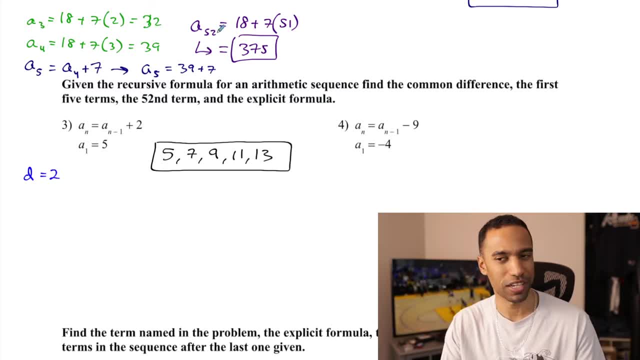 You know, I want to find the explicit formula before I find the 52nd term. If that makes sense, because I'm going to use it to find the 52nd term. 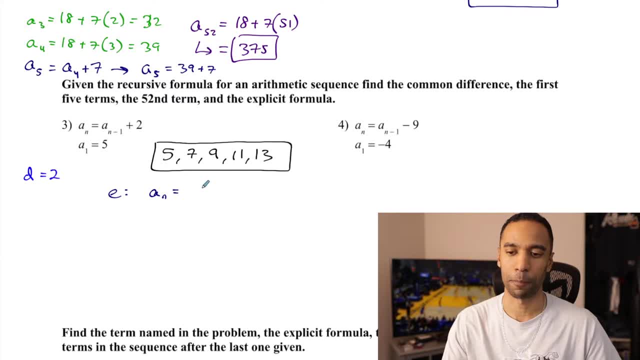 So the explicit formula, the rule is going to be to find the value of some term n, I'm going to start from the first term 5 and I'm going to add 2 one less time than the term that I'm looking for. Because again, we start on the first term and we've got to add 2 51 times to get to the 52nd term. 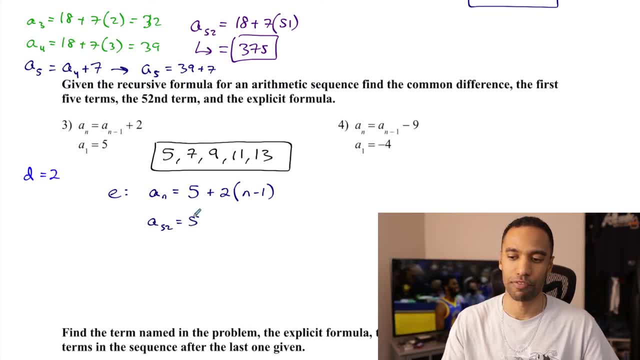 Which is how we're going to do this. a sub 52 equals 5 plus 2 times 51. I mean, do you have to write, well you do have to write the formula because they're asking that we have to. But do you have to say, gosh, what was that formula to make sense of what we're logically doing that we are adding 2 51 times from 5 to get that answer? No, you can still come up with that calculation on your own without that. 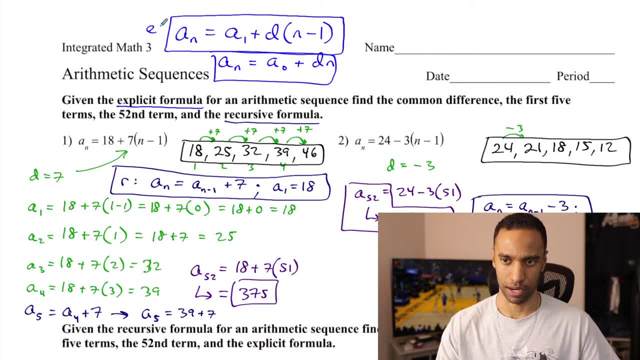 out of what's presented right here. for the, let me put an E here. The explicit formula is presented as such: Use the first term, use the common difference to create it. We have to, you know we have to do that anyway. 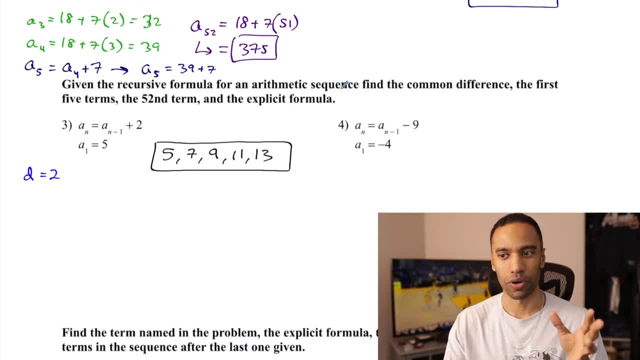 I'm not really a fan of the fact that this is kind of in this order. You know, I want to find the explicit formula before I find the 52nd term, if that makes sense, because I'm going to use it to find the 52nd term. 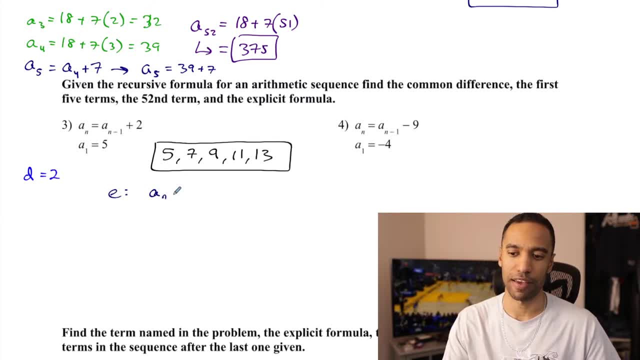 So the explicit formula, the rule, is going to be to find the value of some term n. I'm going to start from the first term, five, and I'm going to add two, one less time than the term that I'm looking for. Because, again, 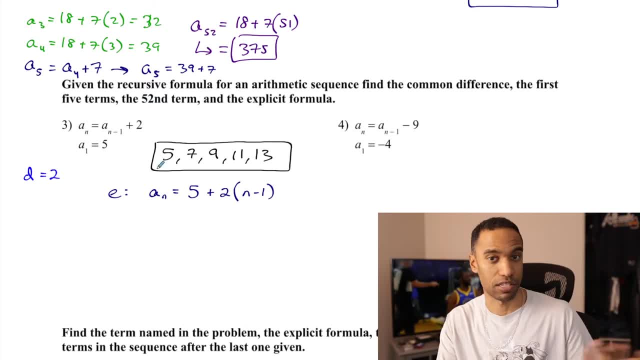 we start on the first term and we got to add two 51 times to get to the 52nd term, which is how we're going to do this. A sub 52 equals five plus two times 51.. I mean, do you have to write? 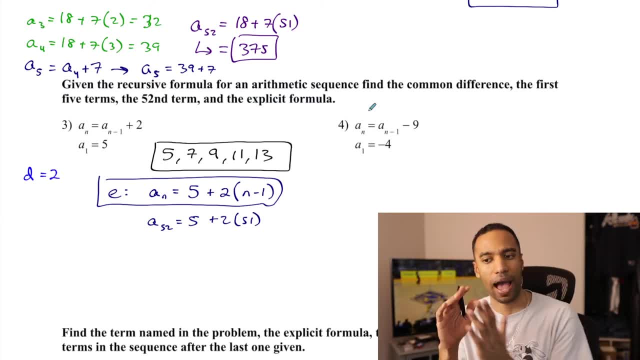 you don't have to write the formula because they're asking that we have to, but do you have to say gosh, what was that formula to make sense of what we're logically doing? that we are adding two, 51 times from five to get that answer. 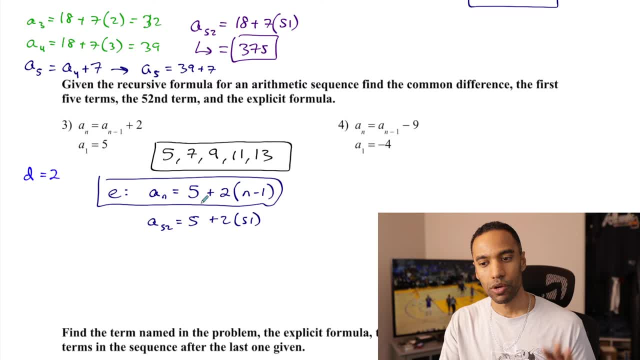 No, you can still come up with that calculation on your own without that, So you don't have to write the formula, except for the fact that it's required, But the 52nd term here you know we're going to do it that way. 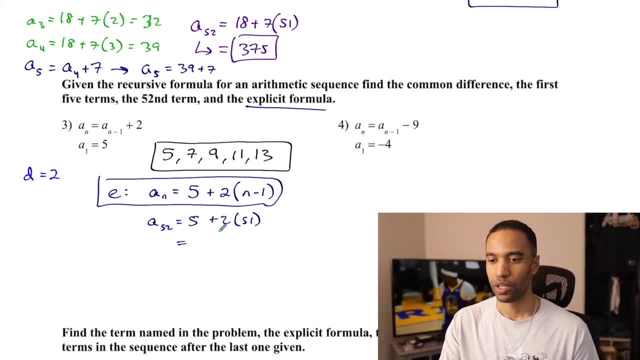 So two times 51 is 102 plus five is 106.. So a sub 52, 52nd term is 107.. Was that it Common difference: first five terms, 52nd term, x plus the formula That was it. 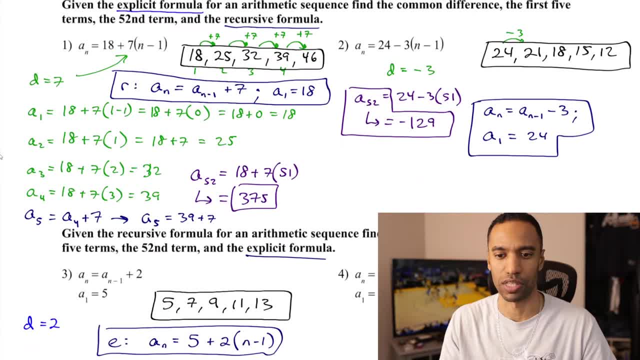 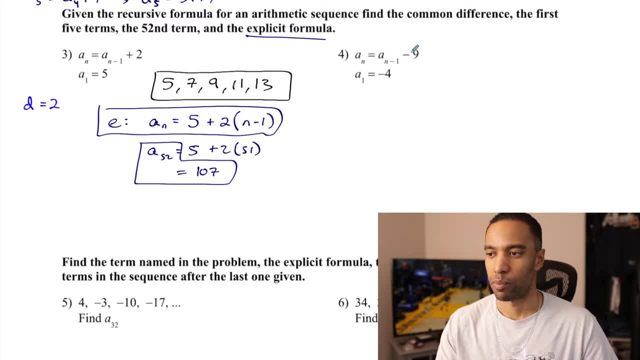 Why did this feel like so much more? Oh, probably just because I was using the output there. All right. And last one here, number four for these problems: a sub n equals a sub n minus one minus nine, And a sub one is negative four. 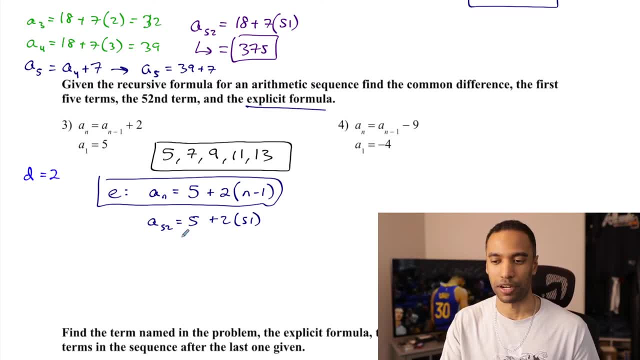 So you don't have to write the formula except for the fact that it's required. 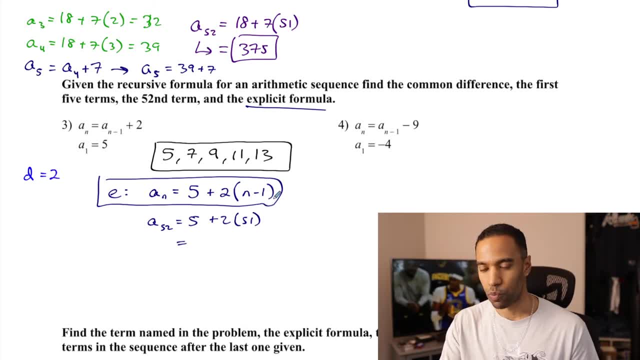 But the 52nd term here, we're going to do it that way. So 2 times 51 is 102 and 5 is 107. So a sub 52 52nd term is 107. 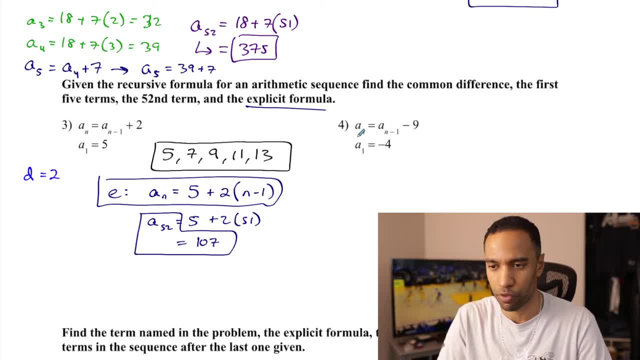 Was that it? Common difference, first 5 terms, 52nd term, x plus the formula. That was it. Why did this feel like so much more? Oh, probably just because I was using the output there. 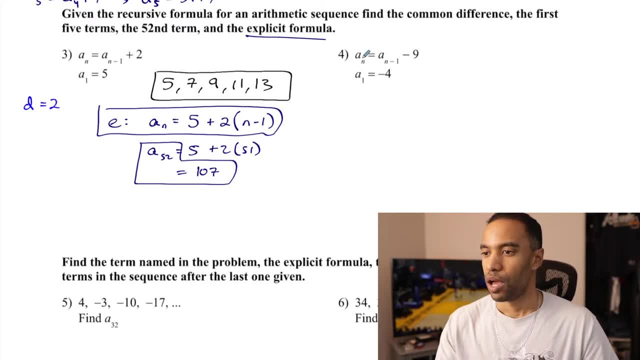 Alright, and last one here, number 4 for these problems. 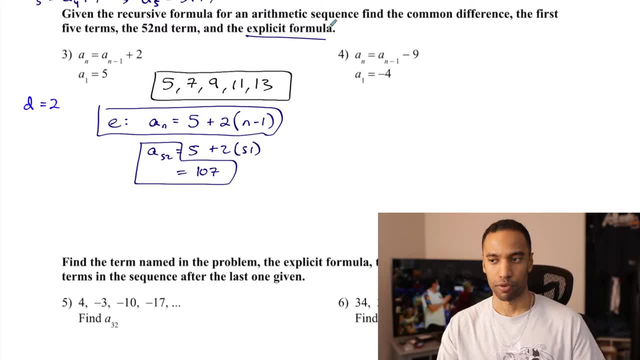 a sub n equals a sub n minus 1 minus 9 and a sub 1 is negative 4. So, common difference with this being a minus is negative 9. 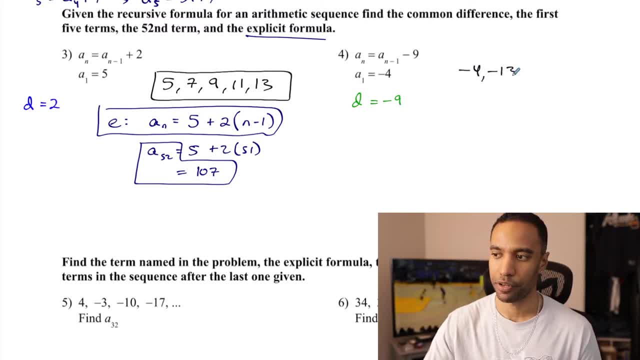 First 5 terms, we start from negative 4 and it looks like we are decreasing to negative 13 minus 9 is negative 22 and then again negative 31 and finally negative 30. So those are the first 5 terms there. 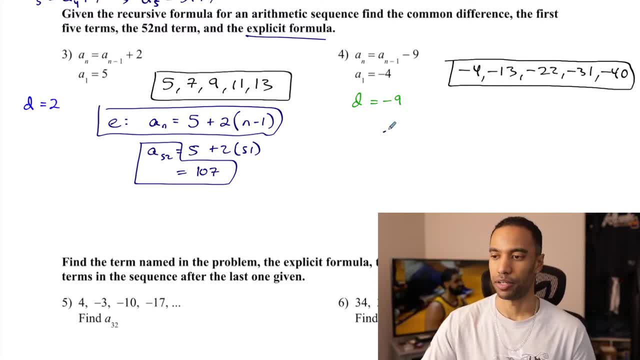 The explicit rule or formula here will be a sub n equals our first term of negative 4 subtracts 9 n minus 1 times and again, one less time than the term you're looking for and the term we're going to be looking for is 52 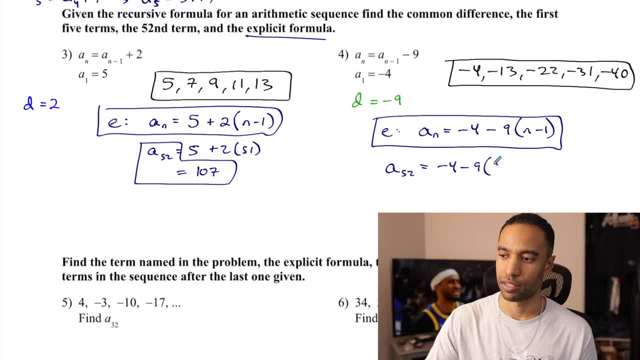 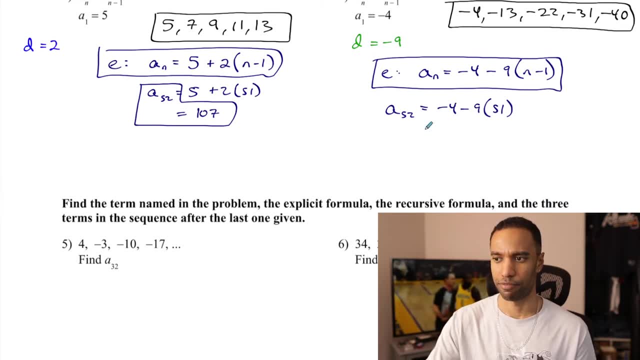 which is negative 4 minus 9 times that same old 51. So negative 459 minus 4 is negative 463. 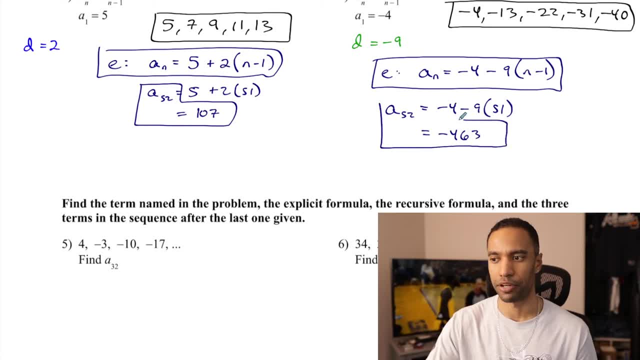 Again, big apologies. I'm saying these things out loud here so you can say, nah, this is what I calculated. 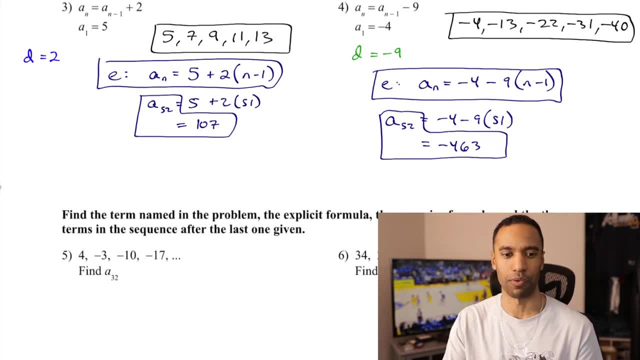 These solution guide videos aren't going to guarantee everything is right. It's a guarantee that what I say is what I believe in the moment. 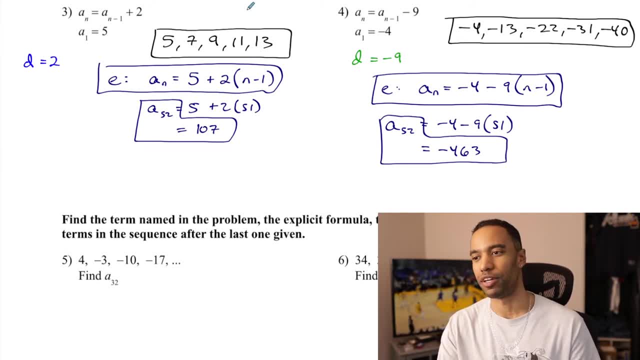 Generally, I've made mistakes before in videos and what I always tell my students as my excuse is 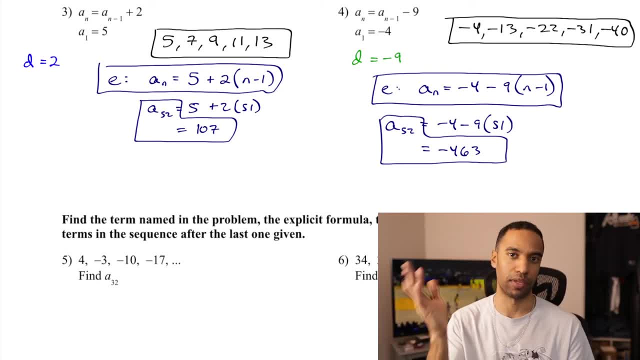 when I'm having a dialogue when I'm speaking about something I turn my brain off from what I'm focusing on. 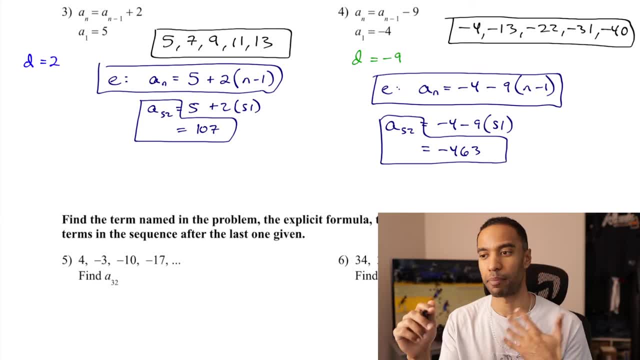 Obviously, as I'm talking through something sometimes I can catch myself, but I feel like I'm having more of a conversation with somebody to make sense of what it is that I'm doing. Was that it for these again? I always forget. Yeah, 52nd term is last there. 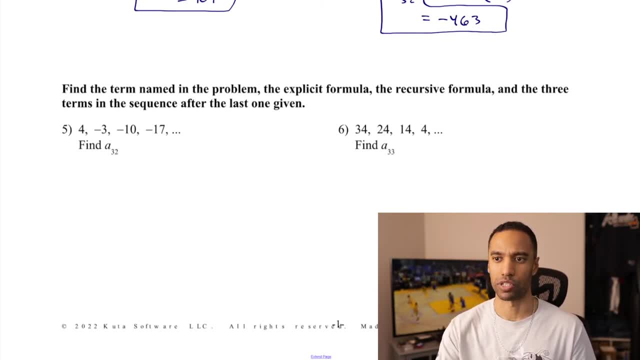 Alright, so those are those ones. Hopefully you're making a little bit of sense of arithmetic sequence provided what you just saw there. Alright, find the term named in the problem, the explicit formula, recursive formula, and the three terms in the sequence after the last one given. 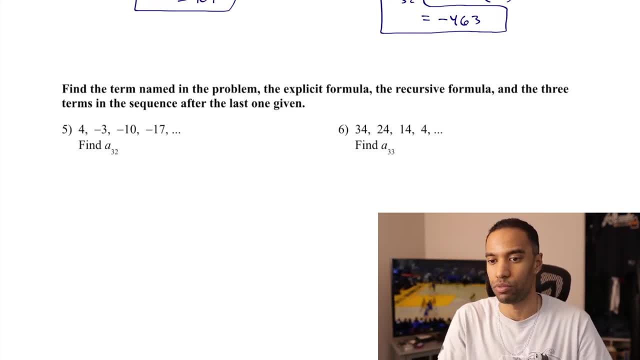 Listen, you can do this in any order you prefer. I'd probably prefer to seek out some information. Get that explicit formula to go ahead and write out the to find this one. Obviously, the recursive formula can follow along. And, you know, whether or not I'm going to use the actual recursive formula to get these next three terms, I don't know. 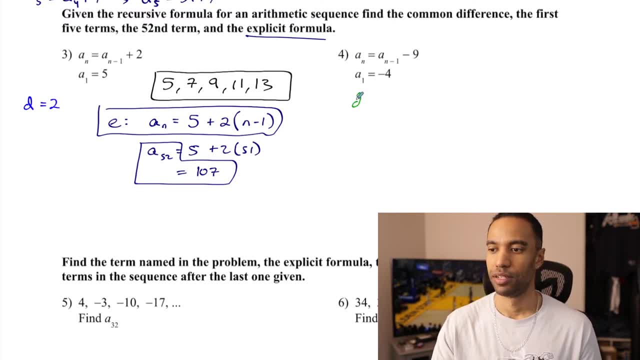 So common difference with this being a minus is negative nine. The first five terms. we start from negative four and it looks like we are decreasing to negative 13 minus nine is negative 22.. And then again negative 31 and finally negative 30.. 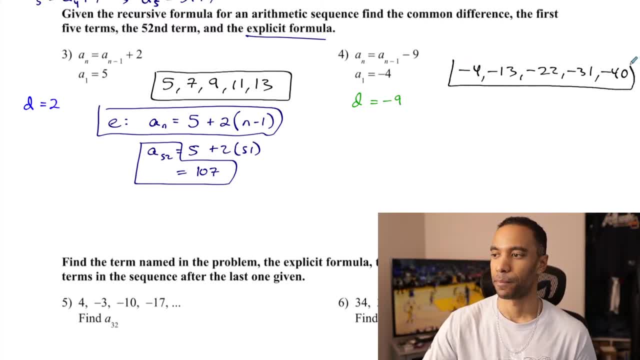 So those are the first five terms there. The explicit rule or formula here will be: a sub n equals our first term of negative four subtracts nine and minus one times, And again one less time than the term you're looking for. And the term we're going to be looking for is a sub 52.. 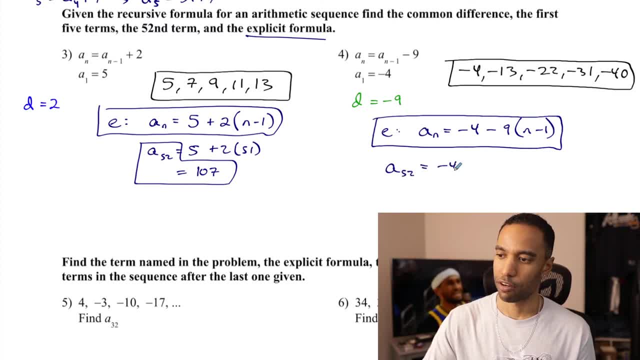 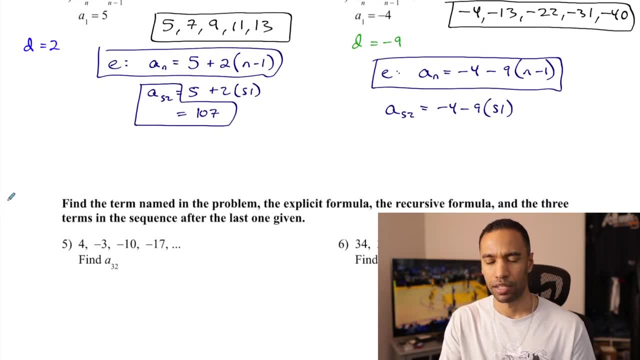 Which is negative four minus nine times that same old 51.. So negative 459 minus four is negative 463.. Again, big apologies. I'm saying these things out loud here So you can say: nah, this is what I calculated. 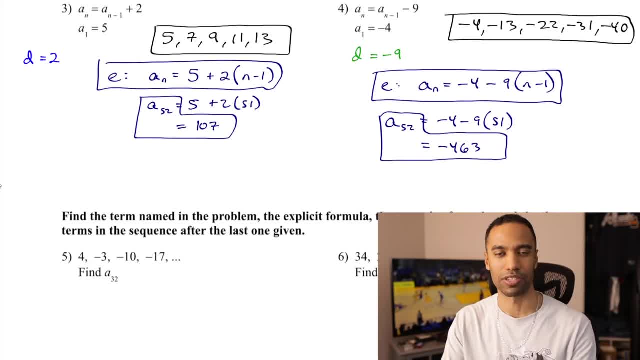 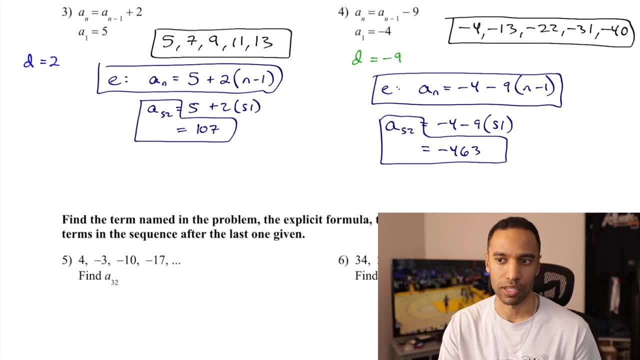 These solution guide videos aren't going to guarantee everything's right. There's a guarantee that what I say is what I believe in the moment Generally- and I've made mistakes before in videos- and what I always tell my students as my excuse is. 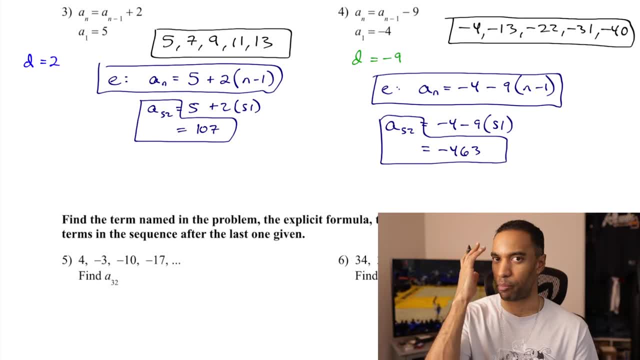 when I'm having a dialogue, when I'm speaking about something, I turn my brain off from what I'm focusing on. Obviously, as I'm talking through something, sometimes I can catch myself, but I feel like I'm having more of a conversation with somebody. 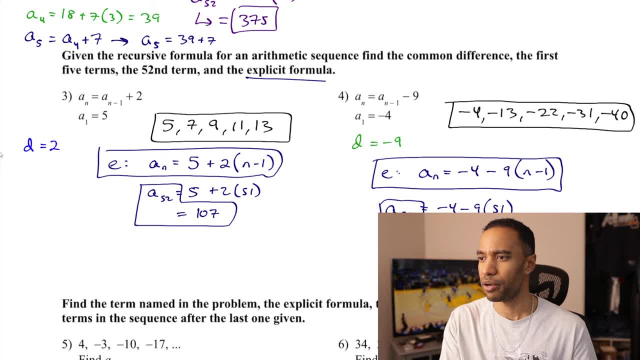 to make sense of what it is that I'm doing. Was that it for these? again, I always forget. Yeah, 52nd term is last there. All right, So those are those ones. Hopefully you're making a little bit of sense of arithmetic sequence. 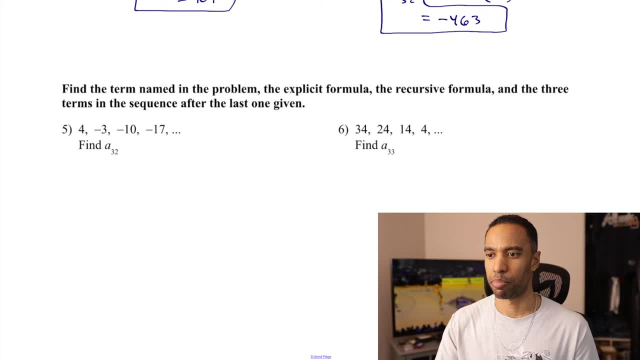 provided what you just saw there. All right, Find the term named in the problem, the explicit formula, the recursive formula and the three terms in the sequence after the last one given: And listen, you can do this in any order you prefer. 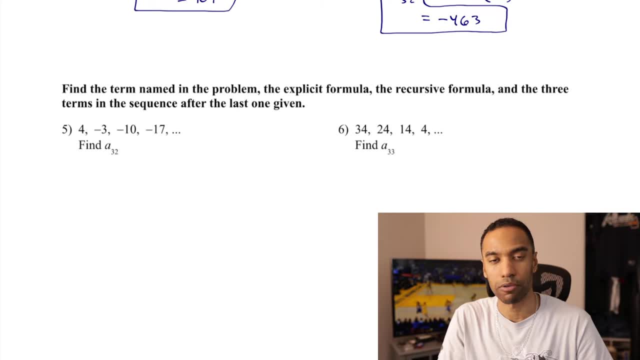 I'd probably prefer to seek out some information, get that explicit formula, to go ahead and write out the to find this one. Obviously, the recursive formula can follow along And you know whether or not I'm going to use the actual recursive formula. 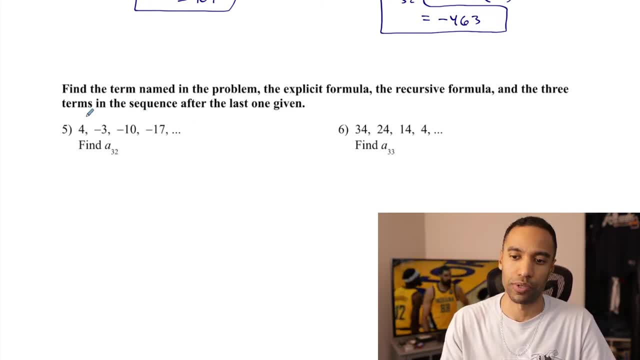 to get these next three terms. I don't know, See, what I would generally do is this. I'd say: hey, what is that common difference? Four plus what is negative three? Well, four plus negative seven, four minus seven. 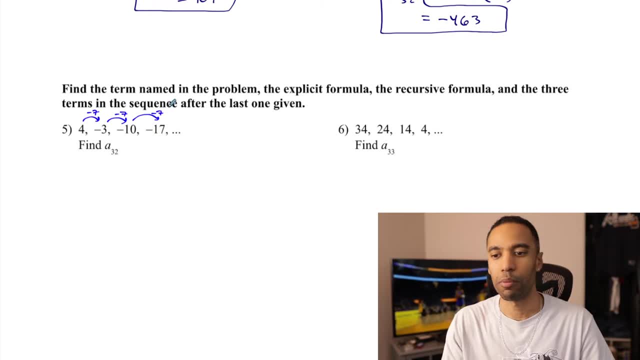 There, right Minus seven, minus seven. Now I want to call attention to something. These problems happen to have relatively simple common differences to obtain through just your knowledge of how to subtract things. But if the numbers are freakishly large, 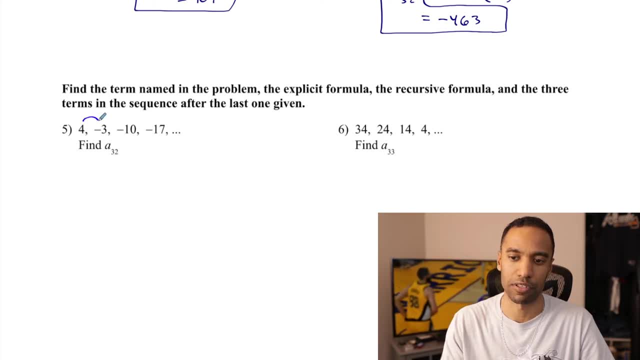 See, what I would generally do is this. I'd say, hey, what is that common difference? 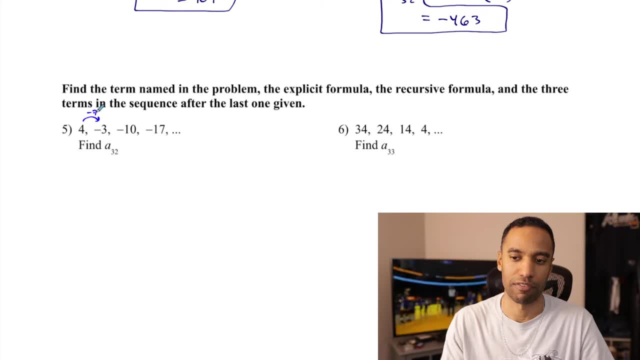 4 plus what is negative 3? Well, it's 4 plus negative 7. 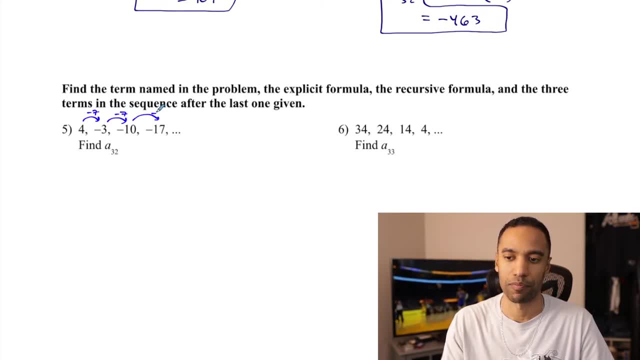 4 minus 7 there, right? Minus 7 minus 7. 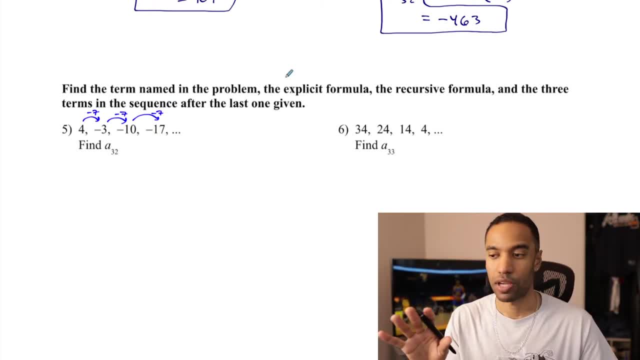 Now, I want to call attention to something. These problems happen to have relatively simple common differences to obtain through just your knowledge of how to subtract things. 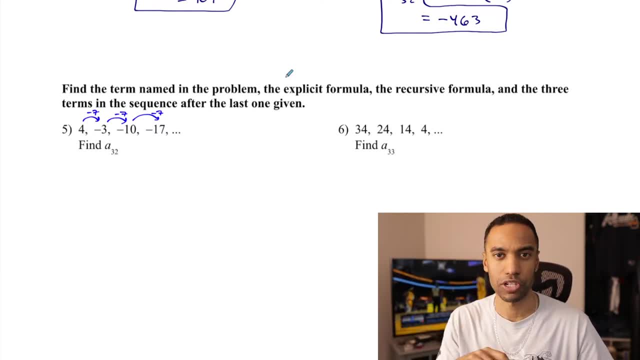 But, if the numbers are freakishly large, if there's a decimal or a fraction, or whatever, if negatives are involved, there are means to figure that out. If we're saying 4 plus some number is negative 3, then we would subtract 4 to figure out what that is. And you'd find out, oh, d is negative 7. 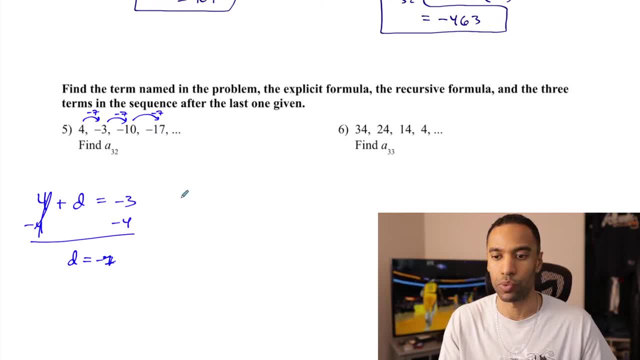 Now, if you already know it's an arithmetic sequence, you only have to do that once. 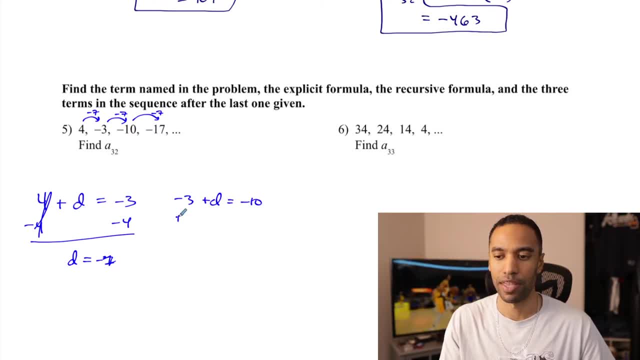 You wouldn't have to do it again, but you could. Negative 3 plus d is negative 10. 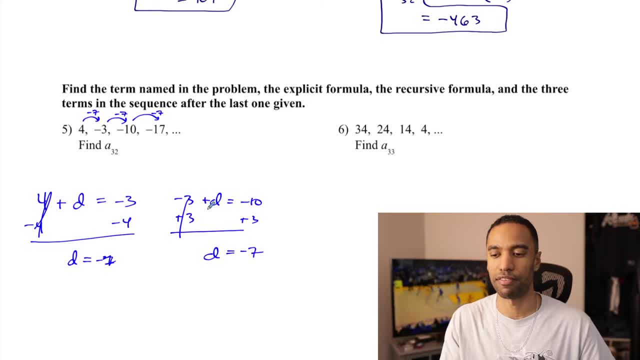 Add 3 to both sides there, and you get d is negative 7. 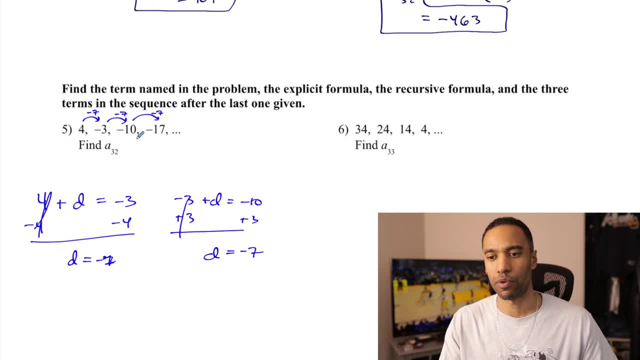 Adding 3 is also subtracting negative 3. And the point that I'm making with it 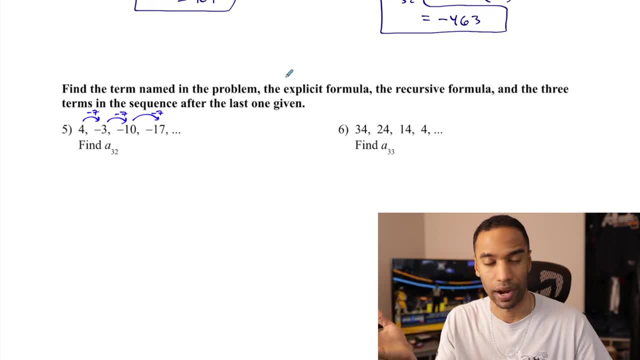 if there's a decimal or a fraction or whatever. if negatives are involved, there are means to figure that out. If we're saying four plus some number is negative three, then we would subtract four to figure out what that is And you'd find out. 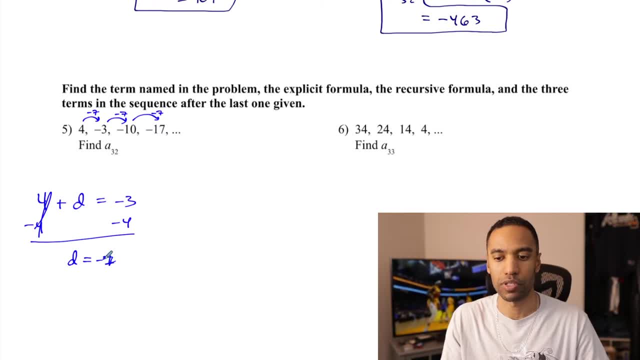 oh, D is negative seven. Now, if you already know it's an arithmetic sequence, you only have to do that once. You wouldn't have to do it again, but you could. Negative three plus D is negative 10.. Add three to both sides there. 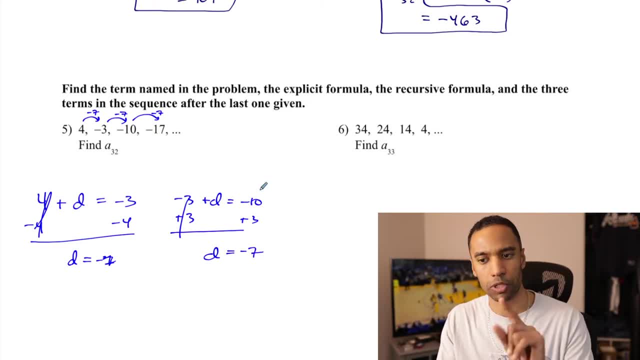 and you get D is negative seven. Adding three is also subtracting negative three And the point that I'm making with it is this: If you want to find your common difference, four plus what is this number? negative three plus what is this number? 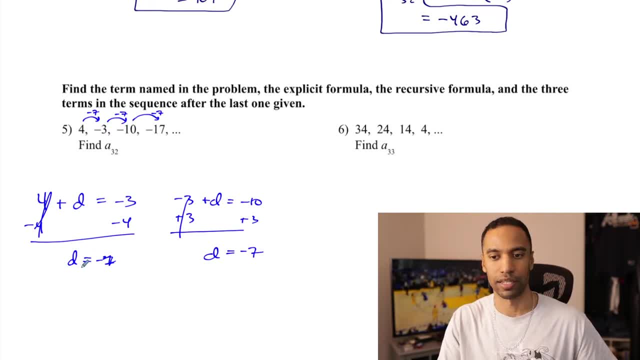 you can do a subtraction of one number from the one before it. I can say: negative three minus four is the same thing as negative 10 minus negative three, which is the same thing as negative 17 minus negative 10.. The point is all of these equal negative seven. 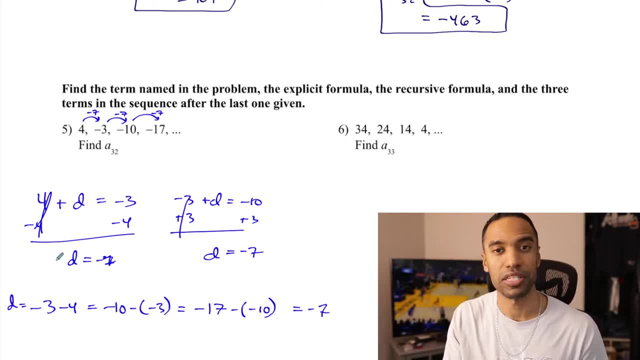 That's what makes it a common difference and that's what makes it a difference. Difference is distance between your two numbers through subtraction to find that result. You know I subtract to find the result. Minus and negative is a plus and we should get negative seven each time. 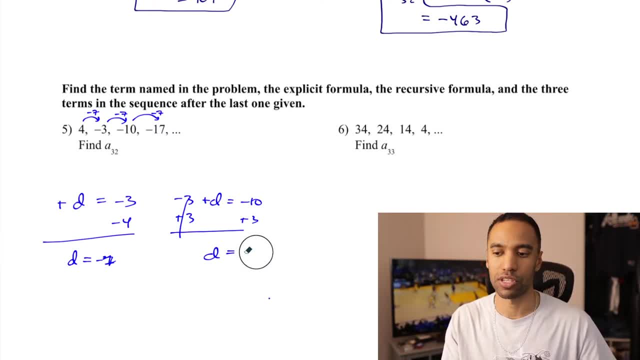 So if it's ever troublesome and you have trouble figuring out what that number is, subtract one number by the one before it in an arithmetic sequence, You will obtain your common difference. So let's find out the next three terms here by simply subtracting seven. 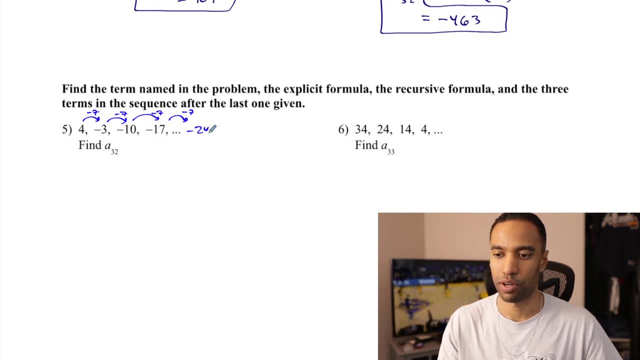 I'm going to do the last instruction first. So the next term is going to be negative 24, and then minus seven, there is negative 31,, and minus seven, there is negative 38.. All right, Find a sub? Sorry. Well, let's do that kind of last-ish. 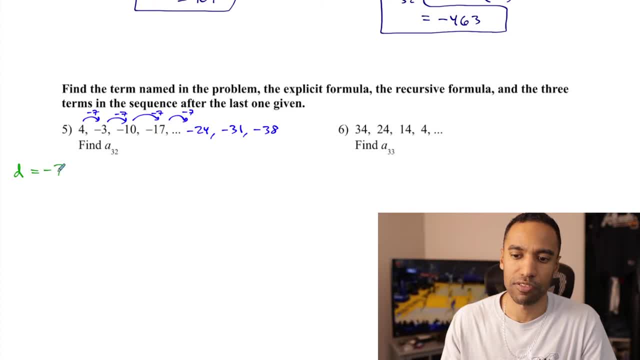 Let's dig out some more information there. So, if D is negative seven, we also know the value of the first term is four, and I mention that only because we need to include this in our formulas. right, We're going to. In fact, that's going to be the recursive formula. 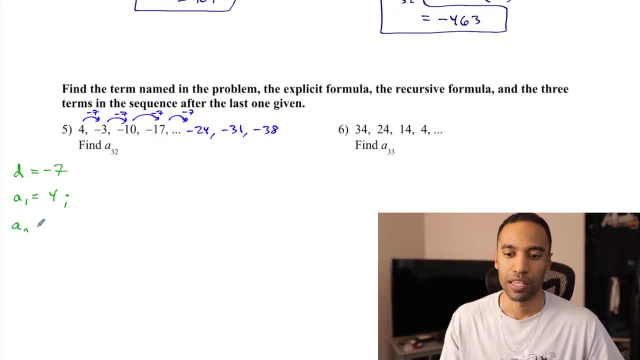 Let's go ahead and start the recursive formula right now. If A sub one is four, to find the value of some term, you take the value of the term before it and you subtract seven. So together all of these represent your recursive formula. 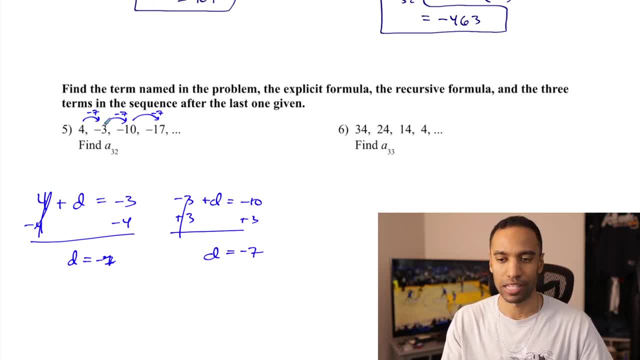 is this. If you want to find your common difference, 4 plus what is this number? Negative 3 plus what is this number? You can do a subtraction of one number from the one before it. 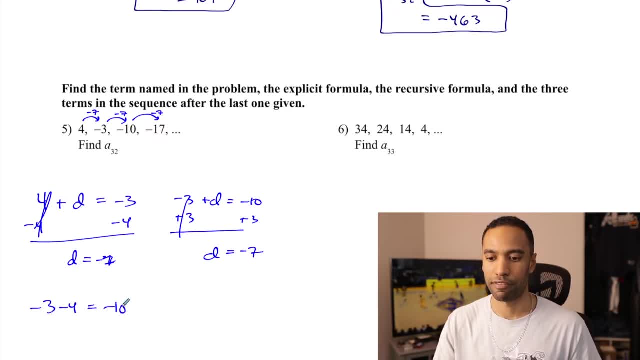 Let's say negative 3 minus 4 is the same thing as negative 10 minus negative 3, which is the same thing as negative 17 minus negative 10. The point is, all of these equal negative 7. That's what makes it a common difference. And that's what makes it a difference. Difference is distance between your two numbers through subtraction to find that result. You know, I subtract to find the result. Minus and negative is a plus. 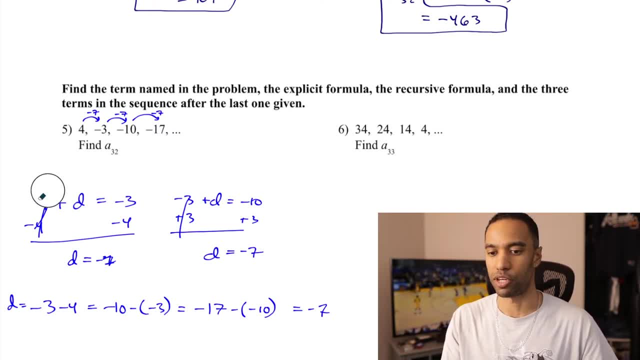 And we should get negative 7 each time. So if it's ever troublesome, and you have trouble figuring out what that number is, subtract 1 number by the one before it in an arithmetic sequence. You will obtain your common difference. So, let's find out the next three terms here by simply subtracting 7. 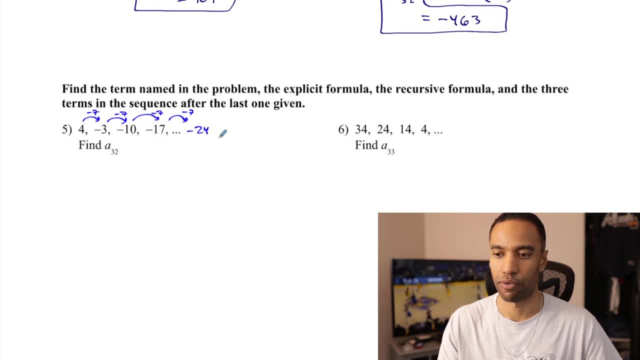 I'm going to do the last instruction first. So the next term is going to be negative 24. 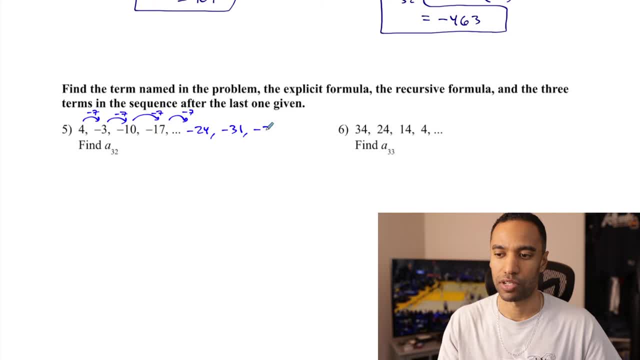 And then minus 7 there is negative 31. And minus 7 there is negative 38. Alright. 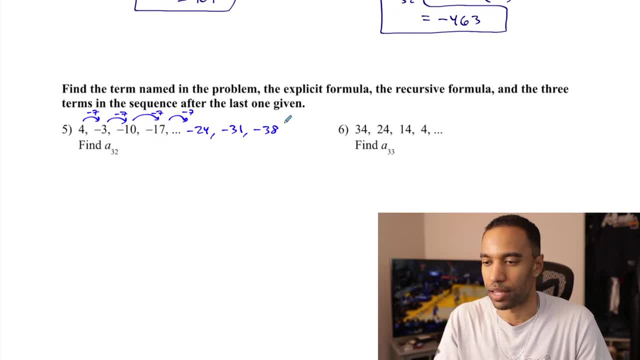 Find a sub- sorry, let's do that kind of last-ish. Let's dig out some more information there. So if d is negative 7, we also know the value of the first term is 4. And I mentioned that only because we need to include this in our formulas. Right? We're going to, in fact, that's going to be the recursive formula. Let's go ahead and start the recursive formula right now. If a sub 1 is 4, to find the value of some term, you take the value of the term before it 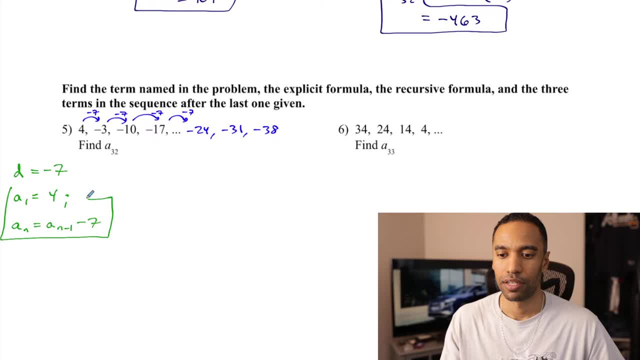 and you subtract 7. So together, all of these represent your recursive formula. Sorry about that. 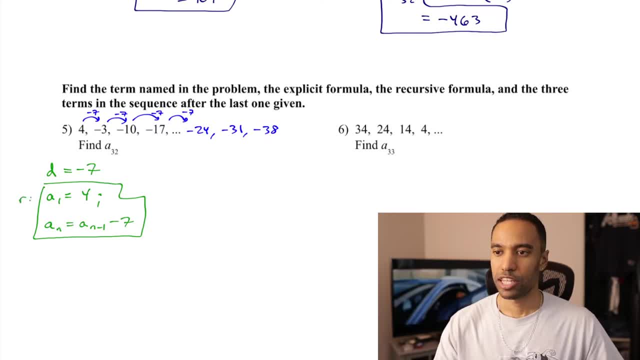 That's the recursive. What's the explicit? Well, the explicit is a sub n equals that first term of 4. 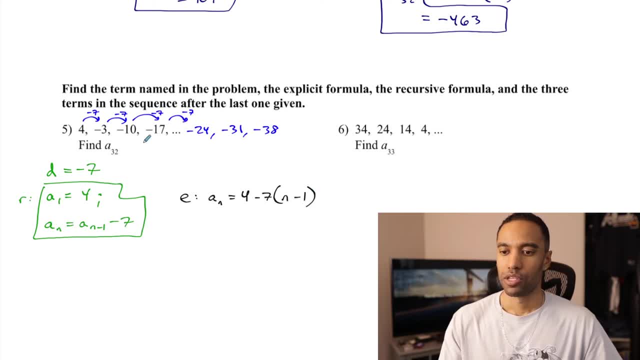 Minus 7 and minus 1 times. So a sub 32, now we're changing things up. a sub 32 is 4 minus 7 times 31. 7 times 31 is 217. So 4 minus 217 is negative 213. Like that. I want 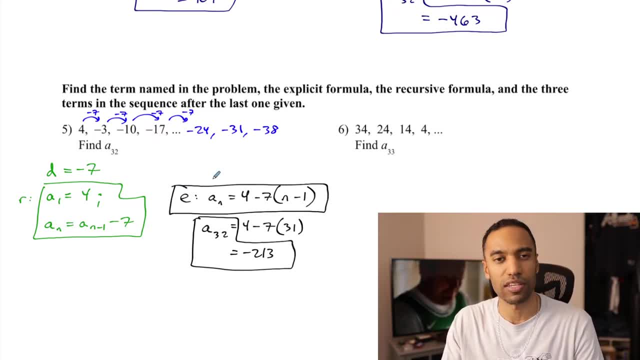 to make mention of one more thing before I move forward. And you know I didn't do this for the previous explicit rules, but I did mention that there's another formula right here for explicit rule. a sub n equals a sub 0 plus dn. 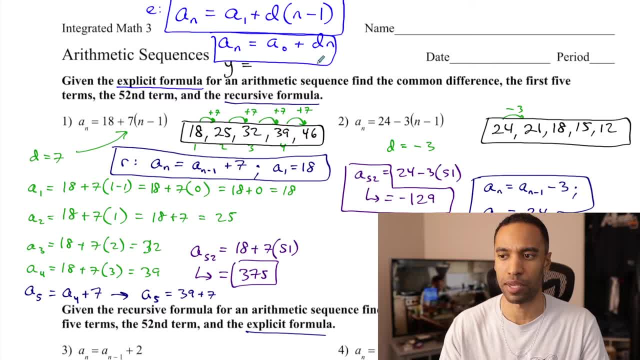 Just so you know, this is very similar to y equals mx plus b, only this is your mx and this is your b over here. Your y intercept, your slope, your input value, things like that. It's very similar to that, which is one reason why I find comfort in doing it. 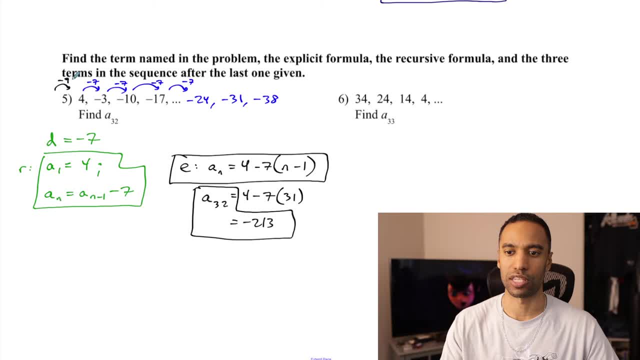 Finding that a sub 0 just means what did I have to subtract 7 to to get 4? And that number is 11. 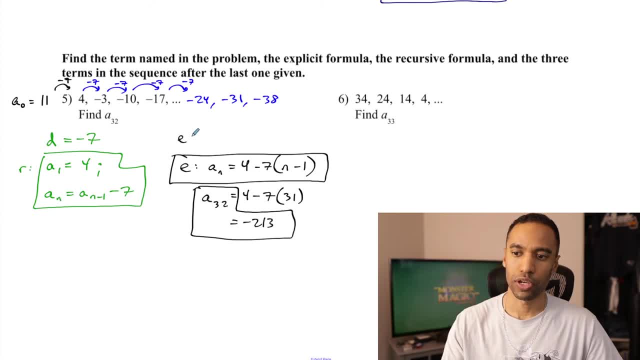 So your a sub 0 is 11. So you could come up with an explicit rule that says a sub n equals, you start from a sub 0 and you subtract 7 exactly 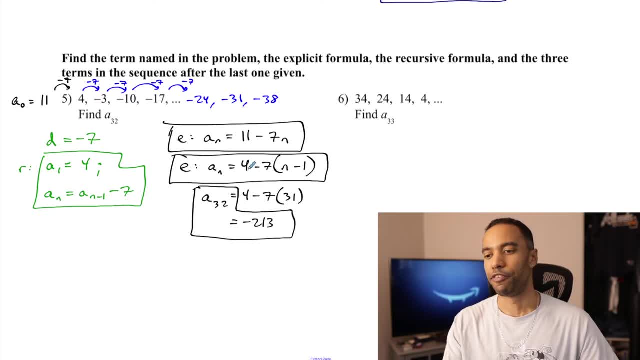 n times. This is an alternative version you could do. And if you're not sure on the formula, and you're like that's another thing to memorize, keep this in mind as well. 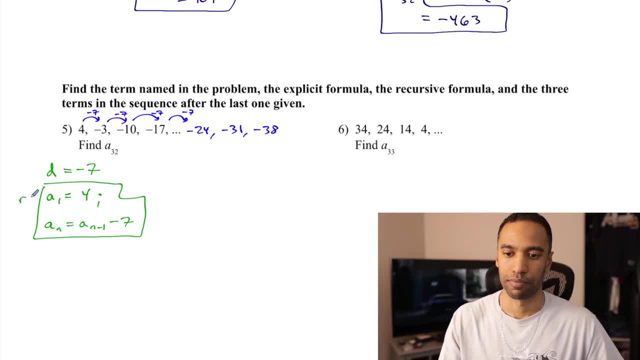 Sorry about that. That's the recursive. What's the explicit? Well, the explicit is A sub one. A sub n equals that first term of four minus seven and minus one times, So A sub 32,. now we're changing things up. 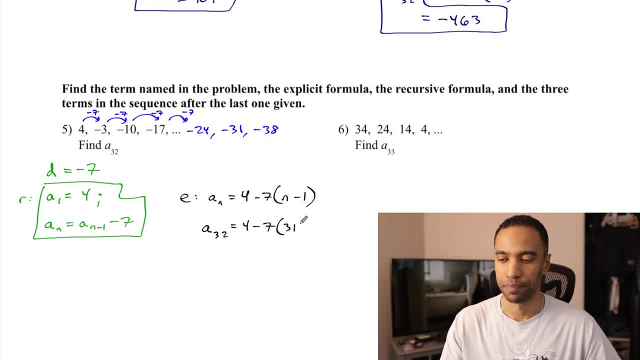 A sub 32 is four minus seven times 31.. Seven times 31 is 217.. So four minus 217 is negative 213.. Like that, I want to make mention of one more thing before I move forward, And you know, 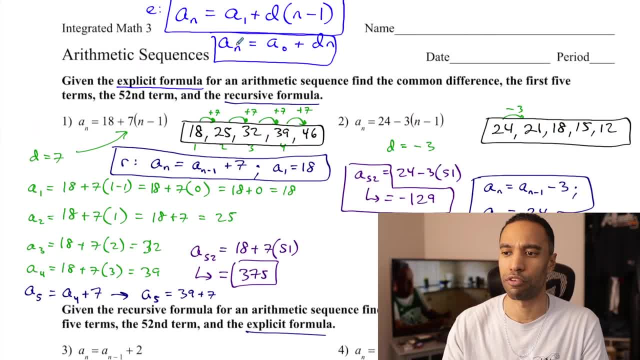 I didn't do this for the previous explicit rules, but I did mention that there's another formula right here for explicit rule: A sub n equals A sub zero plus DN. This is very just so you know. this is very similar to Y equals MX plus B. 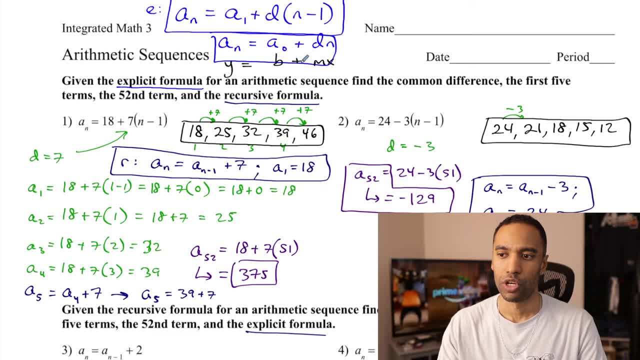 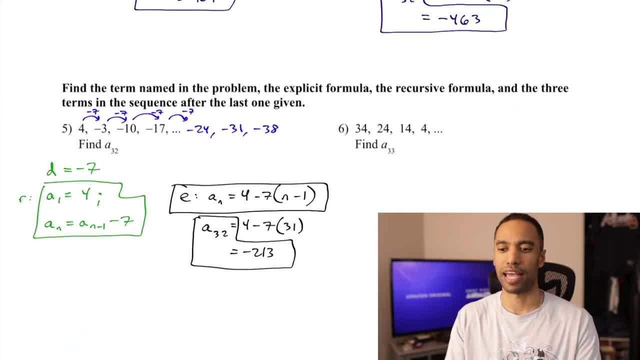 only this is your MX and this is your B. over here, Your Y, intercept your slope, your input, value things like that. It's very similar to that, which is one reason why I find comfort in doing it: Finding that A sub zero just means 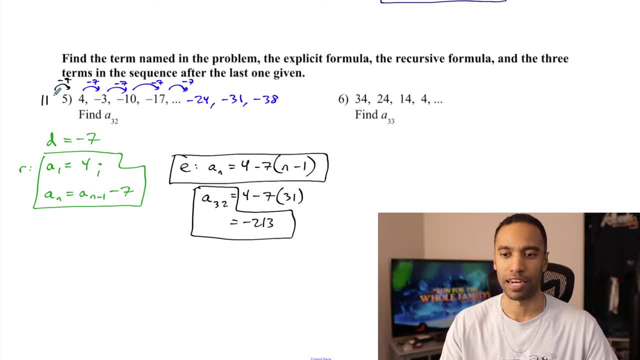 what did I have to subtract seven to to get four, And that number is 11.. So your A sub zero is 11.. So you could come up with an explicit rule that says A sub n equals you start from A sub zero. 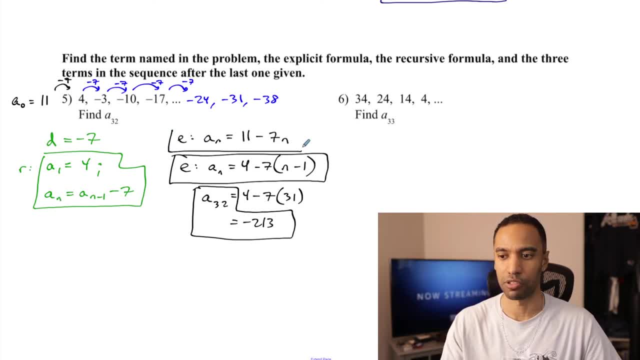 and you subtract seven exactly n times. This is an alternative version you could do And if you're not sure on the formula and you're like that's another thing to memorize, keep this in mind as well In this formula right here: 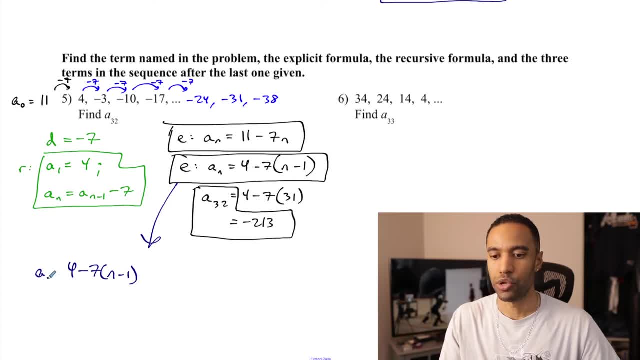 four minus seven times n minus one. you can get to this by right. these are equivalent, right. They're differently written but they're equivalent. You could get this by distributing the negative seven into the n and the negative one. 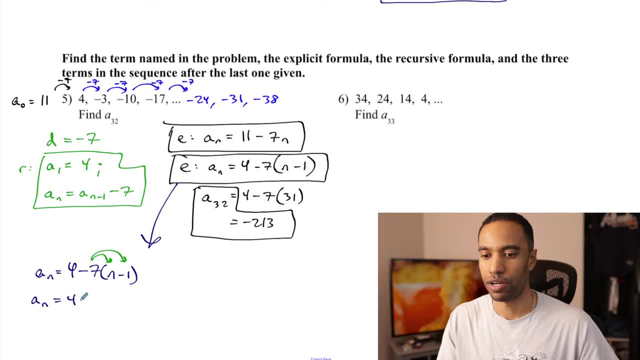 And you'll get A sub n equals four minus seven n plus seven, And four plus seven is 11.. You get A sub n equals 11 minus seven n. There are a lot of different ways you can go about and do this. 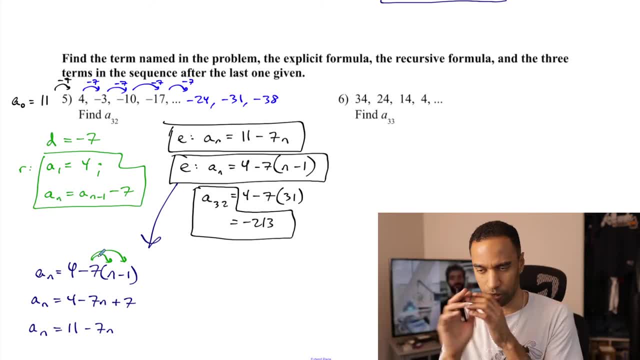 And remember, explicit formula is just. you know it's whatever it can be. If you wanted to write it this way, this is getting really bizarre. If you wanted to say oops, if you wanted to say let's start from the third term. 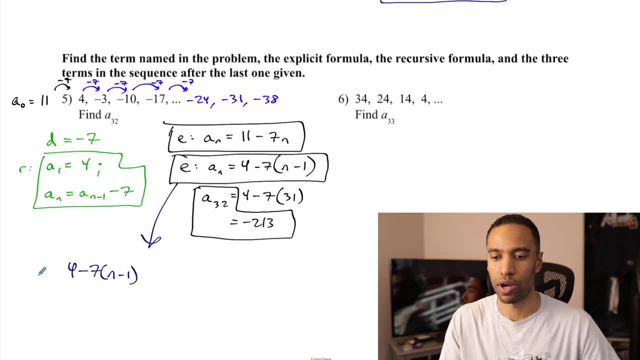 In this formula right here, 4 minus 7 times n minus 1, you can get to this by these are equivalent, right? They're differently written, but they're equivalent. You could get this by distributing the negative 7 into the n and the negative 1, and you'll get a sub n equals 4 minus 7n plus 7, and 4 plus 7 is 11. You get a sub n equals 11 minus 7n. There are a lot of different ways you can go about and do this, and remember, explicit formula is just, you know, it's 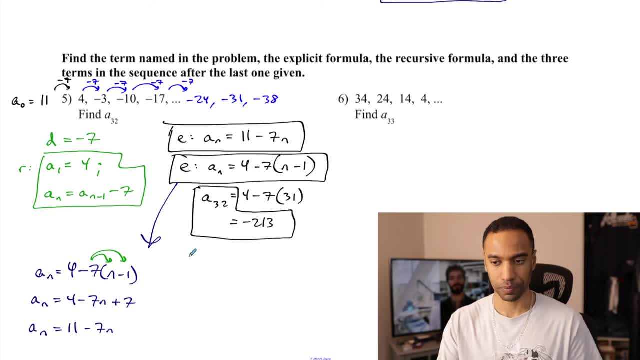 whatever it can be. If you wanted to write it this way, this is getting really bizarre. 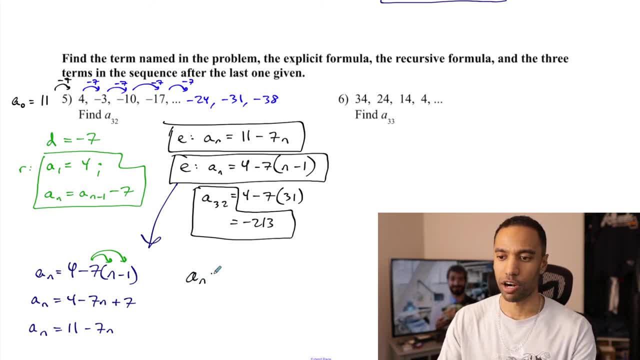 If you wanted to say, if you wanted to say, let's start from the third term, let's start from negative 10. Alright, let's do that. But now you're only going to subtract 7 n minus, whoops, n minus 3 times. Right? This will get you the same answer. This will get you equivalence. 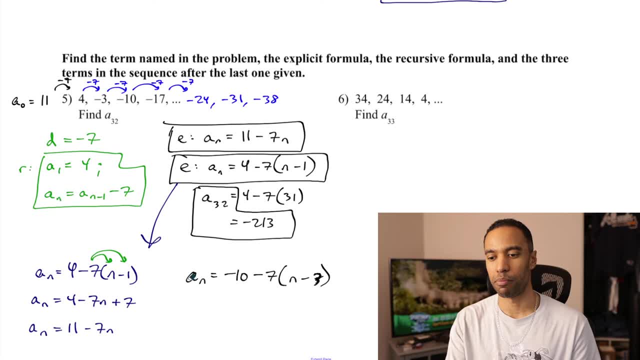 There's no one answer to this, but the fact is, if we start from the first term because it's given, then we don't have to do future calculations to figure anything out. It has the parentheses, and it's a little bothersome to see that, but it works. And I'm going to be doing the same thing for geometric sequences. I'm going to use n minus 1 for those. A sub 0 is a little harder on some geometric sequences, because sometimes you run into fractions that you otherwise normally wouldn't have had. Anyway, I'm speaking a lot. Let's keep moving forward. Number 6. 34, 24, 14, 4. 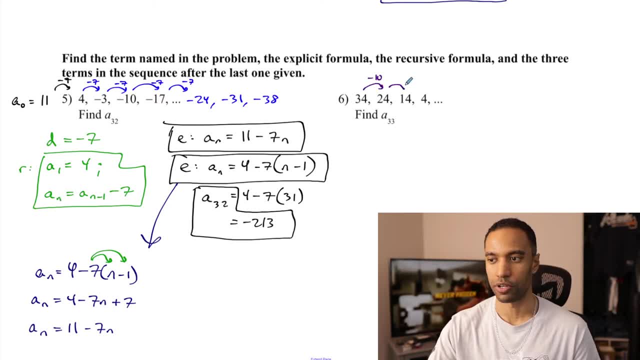 Definitely looks like you're subtracting 10. Can't tell. 24 minus 34 is 10. 14 minus 24 is 10. 4 minus 14 is also 10. So let's subtract 10 three more times for three 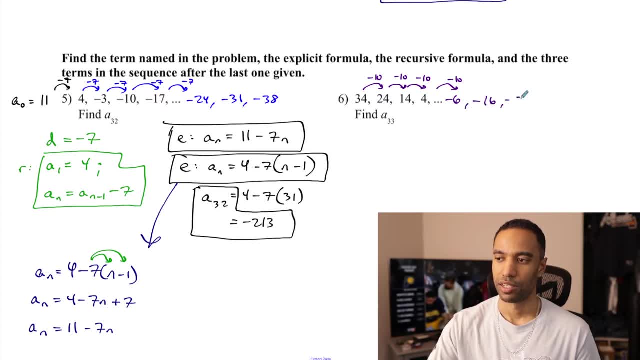 more terms. Negative 6, negative 16, negative 26. Those are three terms after the last one given. 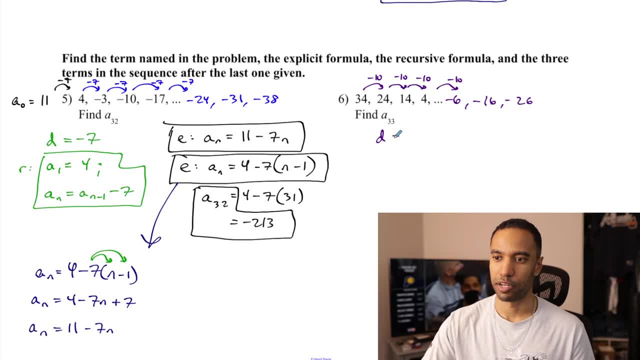 Let's get the recursive formula there after we recognize the common difference for what it was. It was a negative 10. That a sub 1, though, was before. It's the value of the first term. Given that, to find the value of any term after that, take the value of the term before it, and of course subtract 10. As I mentioned, there is your recursive formula. 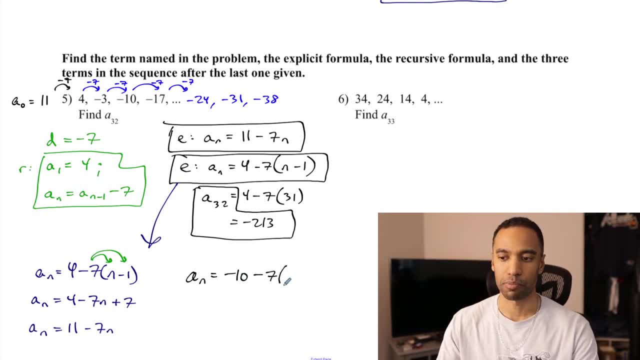 let's start from negative 10.. All right, let's do that. But now you're only gonna subtract seven n minus whoops n minus three times, right? This'll get you the same. this'll get you equivalents. 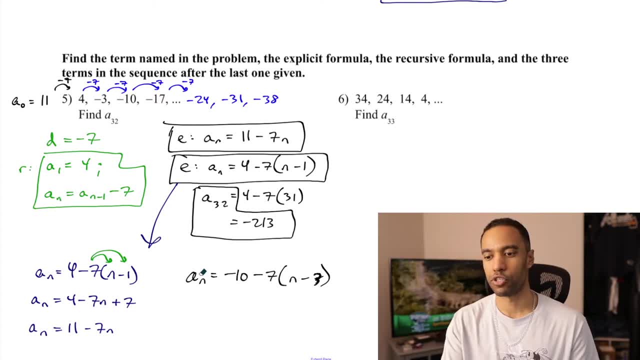 There's no one answer to this, But the fact is if we start from the first term because it's given, then we don't have to do future calculations to figure anything out. It has the parentheses and it's a little bothersome to see that. 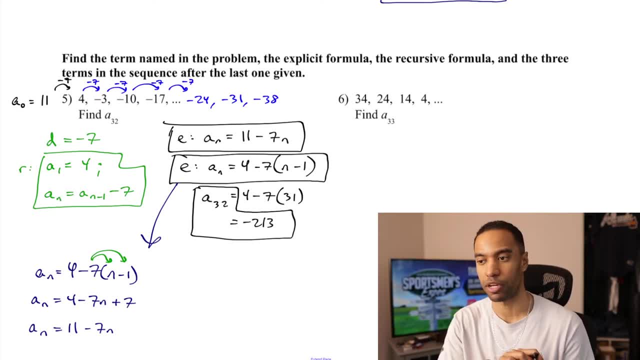 but it works And I'm gonna be doing the same thing for geometric sequences. I'm gonna use n minus one for those. A sub zero is a little harder on some geometric sequences because sometimes you run into fractions that you otherwise normally wouldn't. 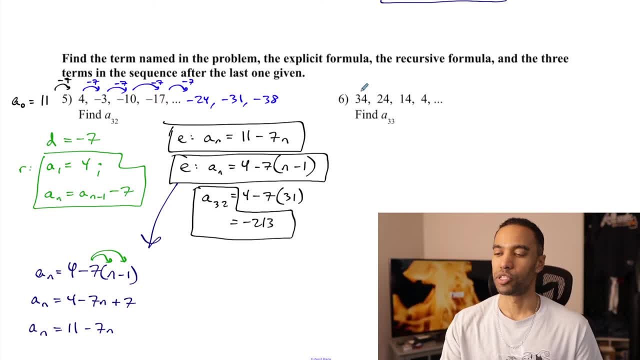 Wouldn't have had. Anyway, I'm speaking a lot. Let's keep moving forward. Number six: 34, 24, 14, four. Definitely looks like you're subtracting 10.. Can't tell: 24 minus 34 is 10.. 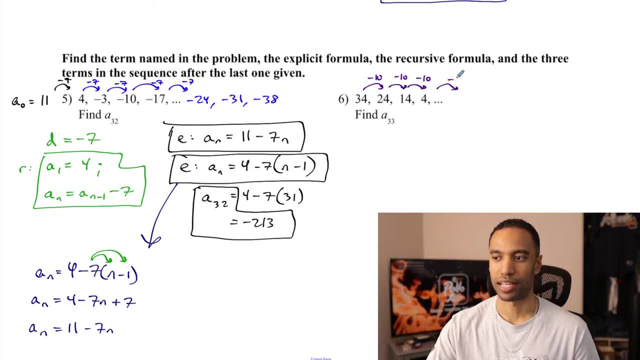 14 minus 24 is 10.. Four minus 14 is also 10.. So let's subtract 10 three more times for three more terms: Negative six. negative 16, negative 26.. Those are three terms after the last one given. 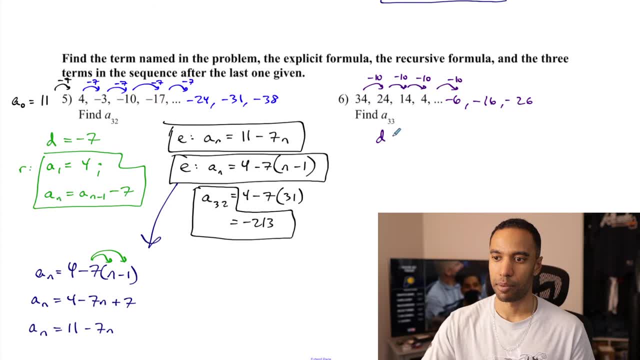 Let's get the recursive formula there After we recognize the common difference. for what it was, it was a negative 10.. That, a sub one, though, was 34.. It's the value of the first term, Given that, to find the value of any term after that. 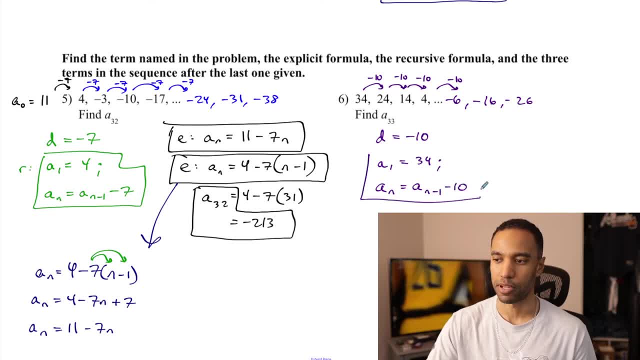 take the value of the term before it and, of course, subtract 10.. As I mentioned, there is your recursive formula, The explicit formula I want to write explicit: The explicit formula based on my a sub one version is: a sub n equals a sub one minus 10 times n minus one. 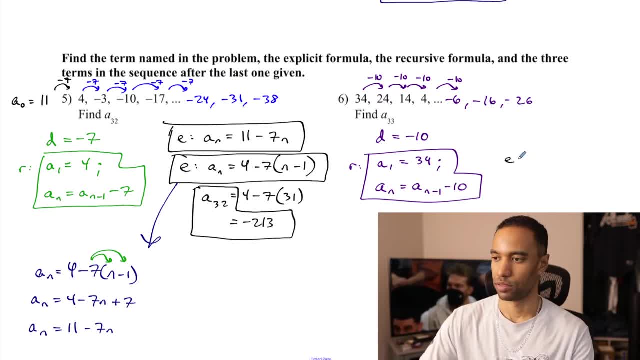 The explicit formula I want to write explicit. The explicit formula, based 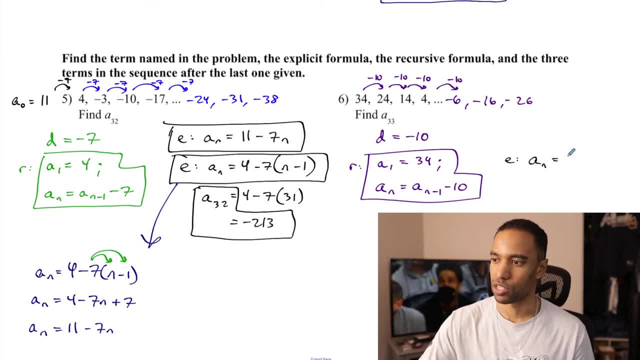 on my a sub 1 version, is a sub n equals a sub 1 minus 10 times n minus 1. 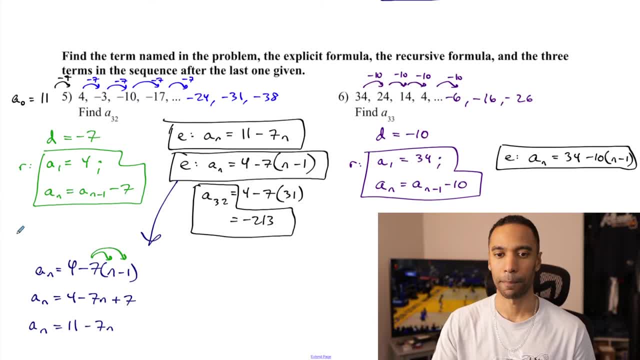 Let's use this to find a sub 33. 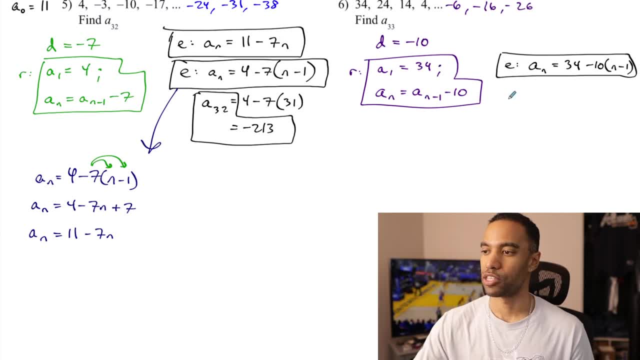 Moving up in the world from 32 to 33. So a sub 33 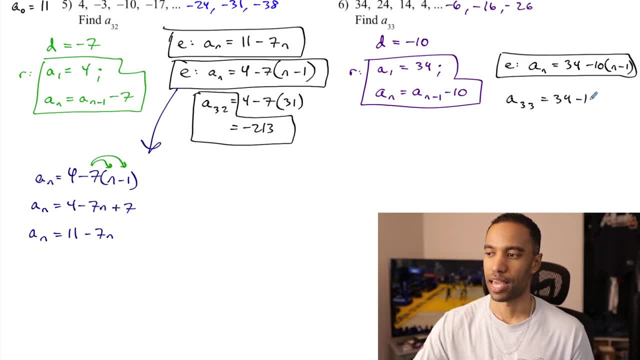 is 34 minus 10 times 33 minus 1. 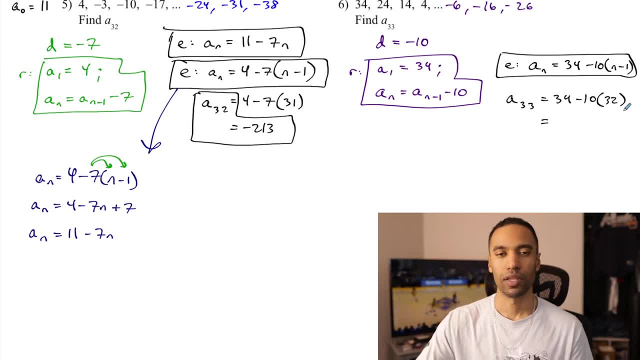 I like 10 times 32 is 320. 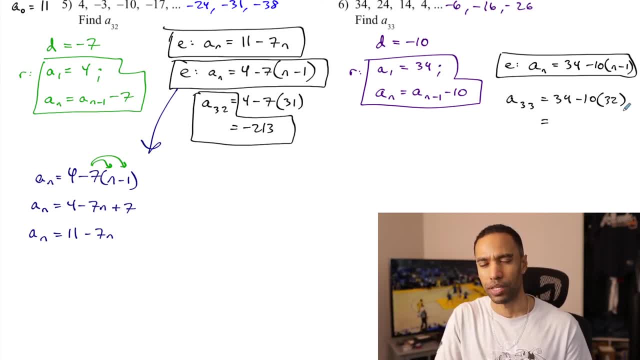 I don't know 34 minus 320. Wait, 320? 286. 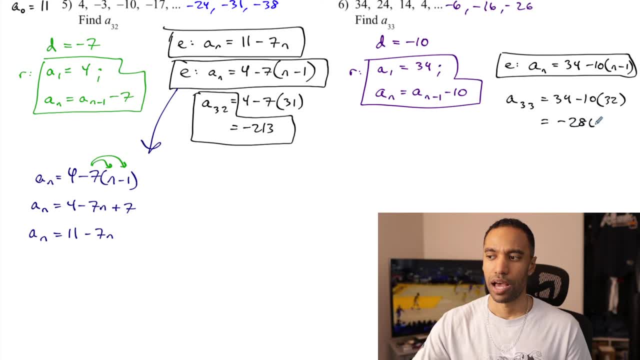 I'm getting negative 286. 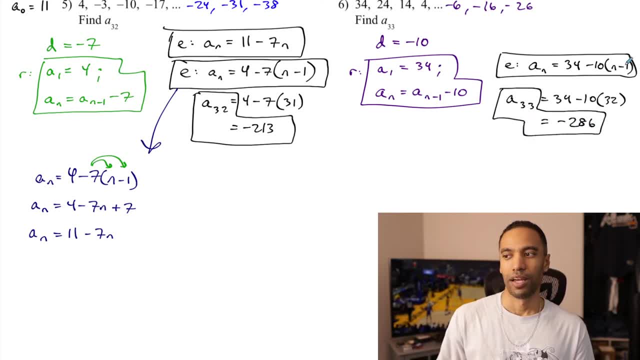 I swear, and I've said this before in some math things if you've heard me. 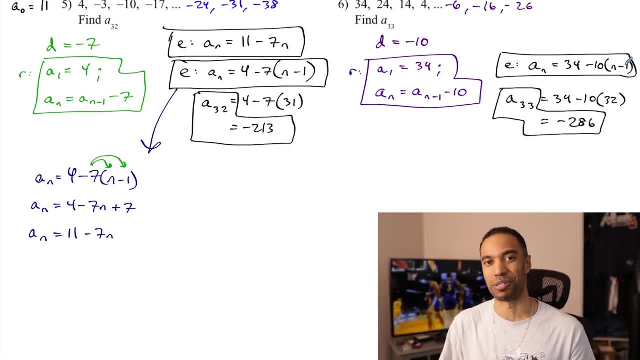 Pretty good multiplication. I'm getting really bad in addition and subtraction. 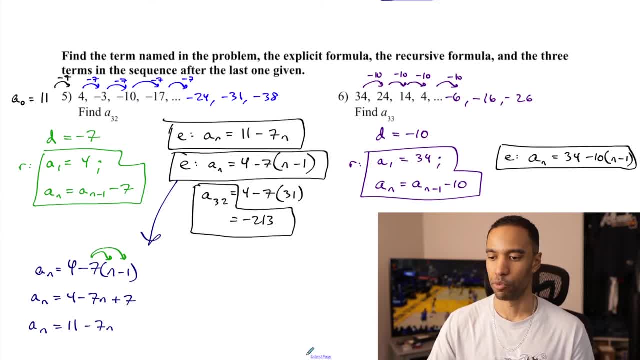 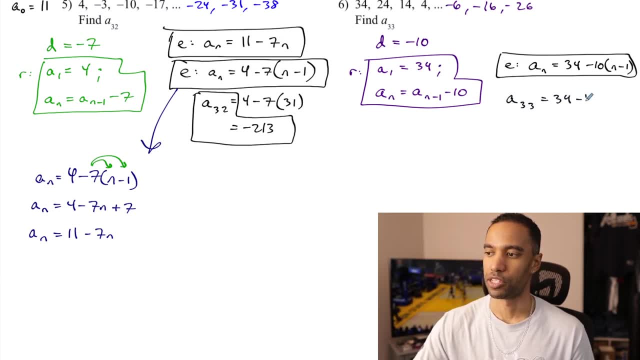 Let's use this to find a sub 33, moving up in the world from 32 to 33.. So a sub 33 is 34 minus 10 times 33, minus one, I like. 10 times 32 is 320.. 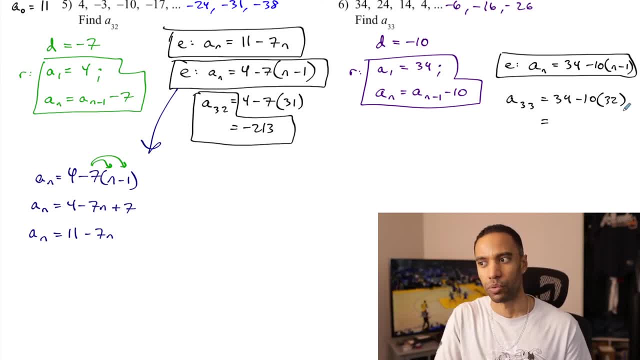 I don't know- 34 minus 320.. One wait, 320, 286.. I'm getting really negative 286.. I swear- and I've said this before in some math things, if you've heard me- pretty good multiplication. 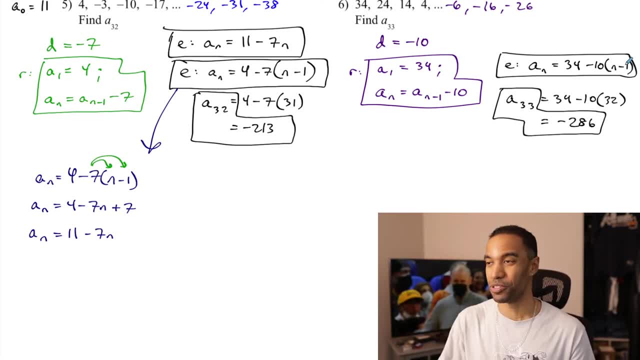 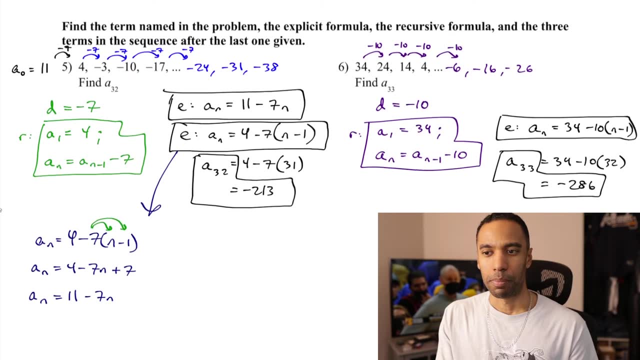 I'm getting really bad in addition, and subtraction, mostly subtraction- I'm getting really bad in it. I apologize if that's wrong, but I think it's good And that will be it for those explicit recursive next three terms and 33rd term. Mostly subtraction. I'm getting really bad in it. 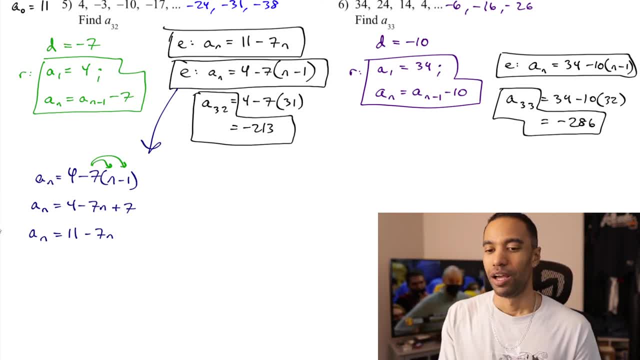 I apologize if that's wrong, but I think it's good. 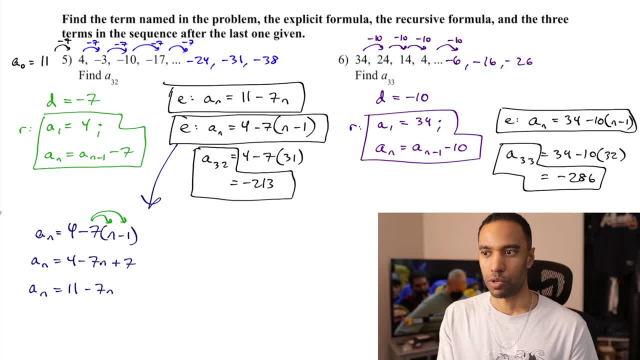 And that will be it for those. Explicit, recursive, next three terms, and 33rd term. Okay. 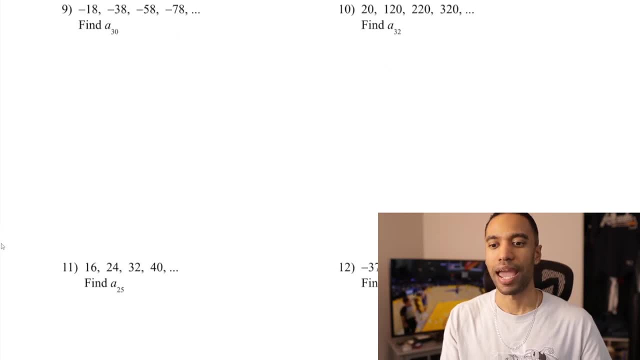 Let's move forward. I've got six more problems to do, and these are all of the same variety now as what you just saw before. So we've got a sequence. Keep doing the same thing as we did before. 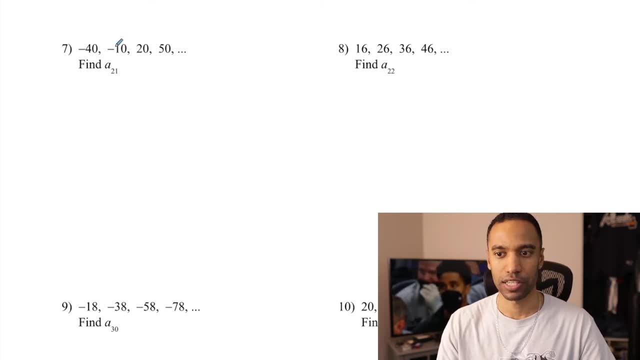 So, common difference. See, check this out. 50 minus 20. I mean, you know the answer, but 50 minus 20 is 30 right there. So we are going to add 30 to get the next three terms here to get 80, 110, and 140. 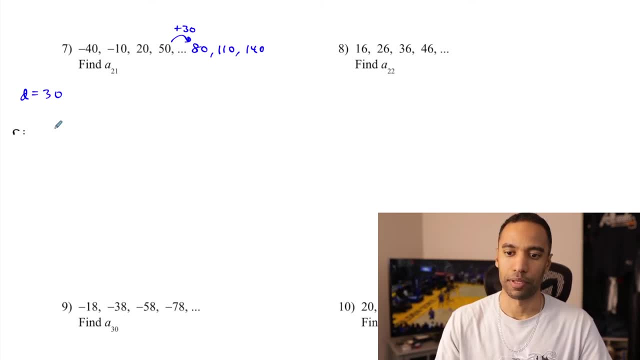 The let's do the recursive formula because I keep mentioning a sub 1. Let's start with the a sub n part. a sub n is a sub n minus 1 plus 30. And a sub 1 is negative 40. There's your recursive formula. The explicit formula. Oh my goodness. 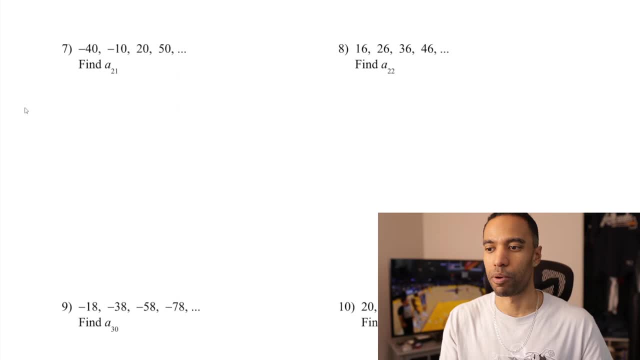 Okay, let's move forward. I got six more problems to do, and these are all of the same variety now as what you just saw before. So we've got a sequence: Keep doing the same thing as we did before. So common difference. 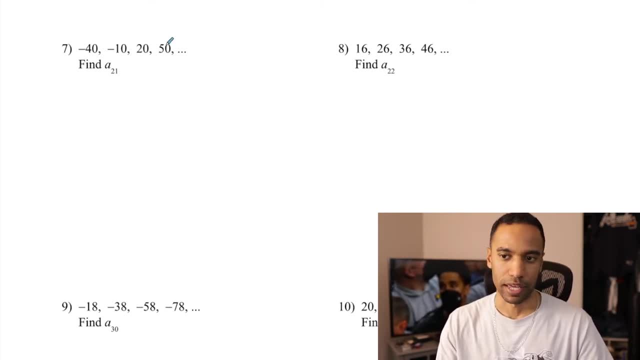 See, check this out: 50 minus 20.. I mean, you know the answer, but 50 minus 20 is 30 right there. So we are going to add 30 to get the next three terms here, to get 80,. 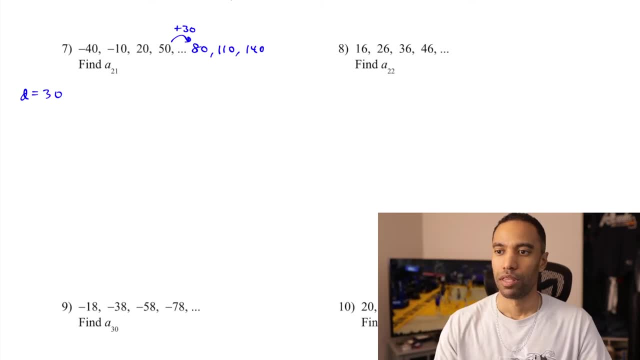 110, and 140.. Let's do the recursive formula. because I keep mentioning a sub one, Let's start with the a sub n part. A sub n is a sub n minus one plus 30.. And a sub one is negative 30.. 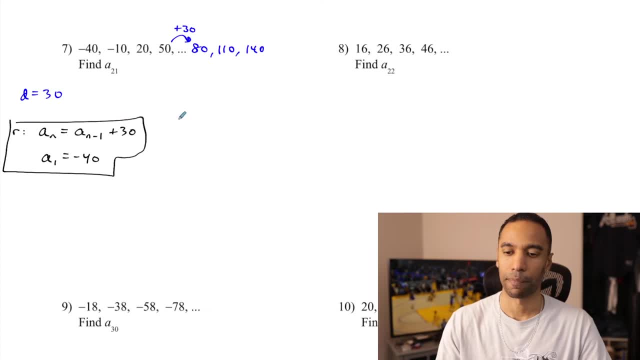 Negative 40.. There's your recursive formula, The explicit formula. Oh my goodness. The explicit formula is: a sub n equals a sub one negative 40 plus 30 times n minus one. I'll take it If you want to distribute that. 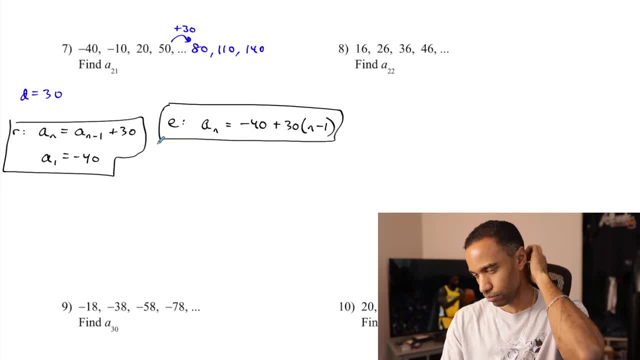 you'll get negative 70 plus 30 n and a sub 21.. A sub 21 is negative 40.. Whoa Plus 30 times 21, minus one, That's 20.. 30 times 20 is 600.. 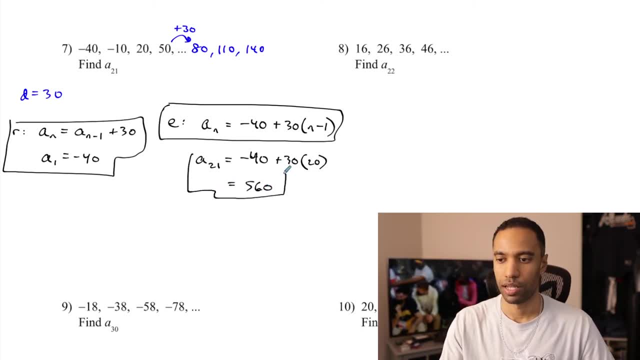 Minus 40 is 560.. So there's a sub 21.. I think that's it for that problem. Yeah, All these, I'm going to fly through the rest of them now. I only talk just to kind of break the silence. 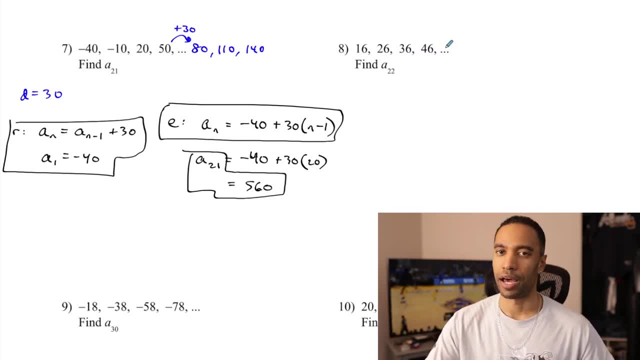 But at this point I don't know if there's more that I'm bringing on other than giving you answers, So I hope you're okay with that. Looks like we're adding 10.. What else is new? We got 56,, 66, and 76 here. 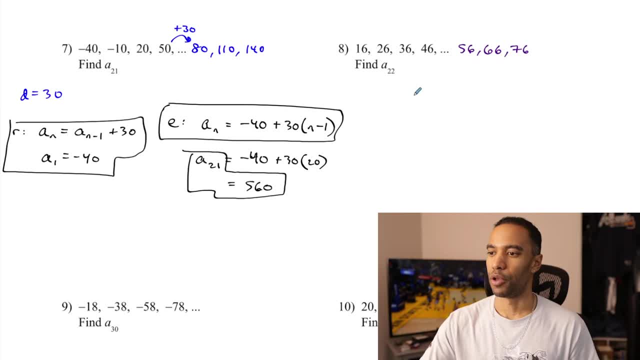 Let's see how fast we can concoct these things here. Recursive formula is: a sub n equals a sub n minus one plus 10.. We are starting from 16.. The explicit formula is a sub n equals 16 plus 10 times n minus one. 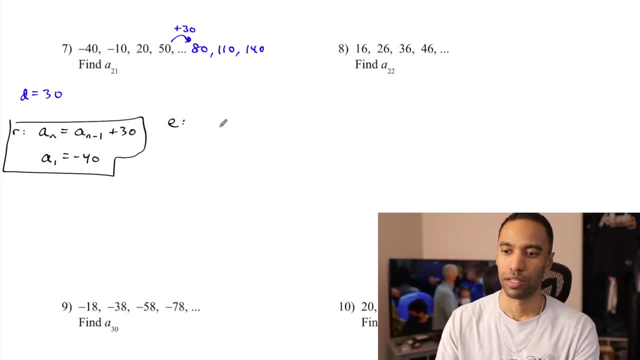 The explicit formula is a sub n equals a sub 1, negative 40, plus 30 times n minus 1. I'll take it. If you want to distribute that, you'll get negative 70 plus 30 n. 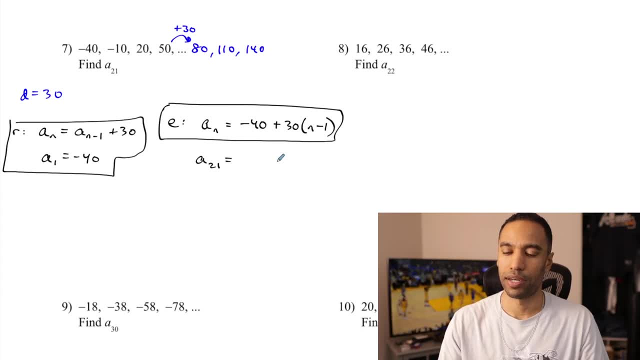 And a sub 21. a sub 21 is 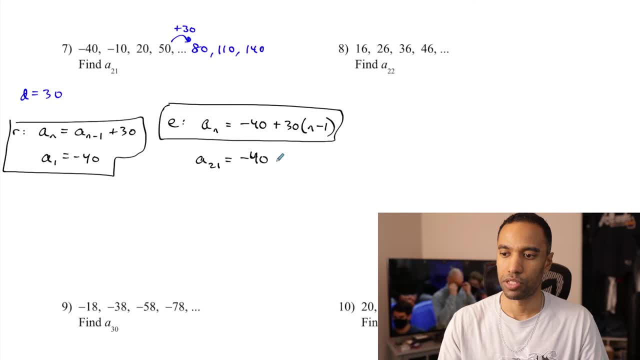 negative 40 plus 30 times 21 minus 1. That's 20. 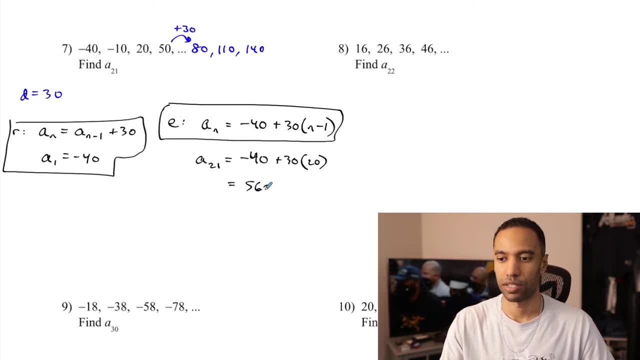 30 times 20 is 600. Minus 40 is 560. So there's a sub 21. I think that's it for that problem. 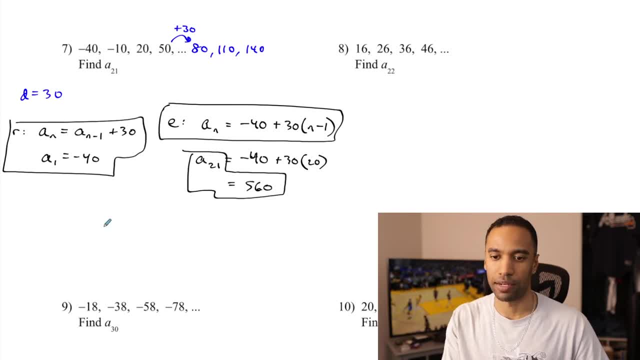 Yeah. All these, I'm going to fly through the rest of them now. I only talk just to kind of break the silence. But at this point, I don't know if there's more that I'm bringing on other than giving you answers. So I hope you're okay with that. 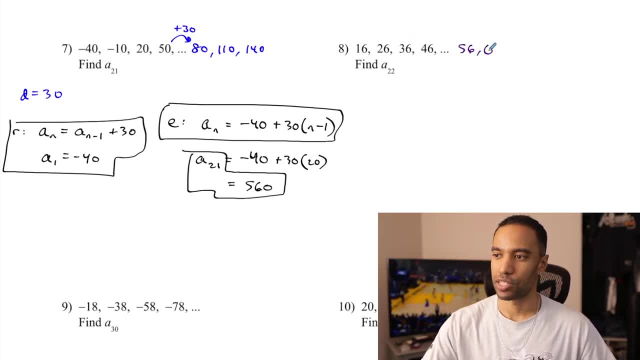 Looks like we're adding 10. What else is new? We got 56, 66, and 76 here. 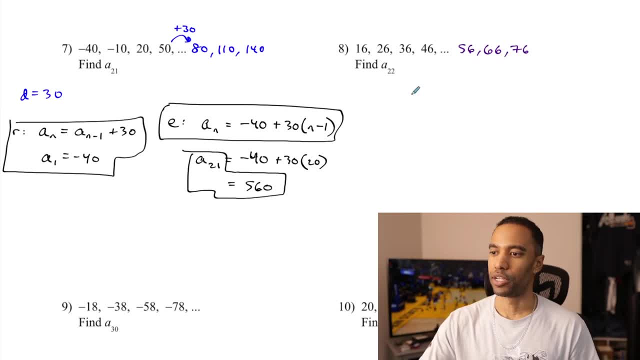 Let's see how fast we can concoct these things here. 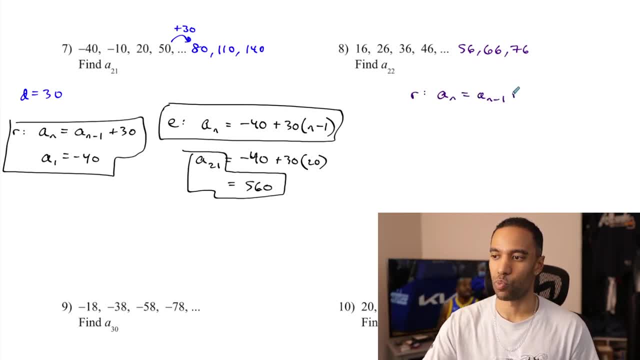 Recursive formula is a sub n equals a sub n minus 1 plus 10. We are starting from 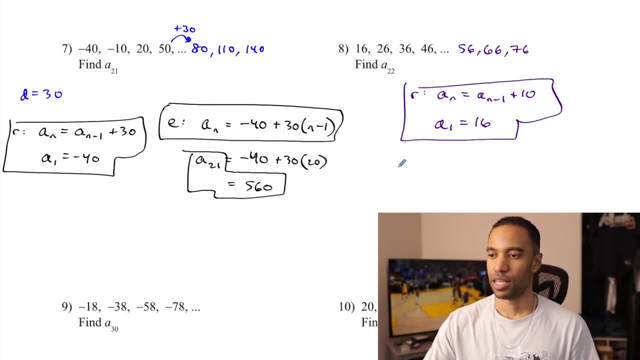 16. The explicit formula is a sub n equals 16 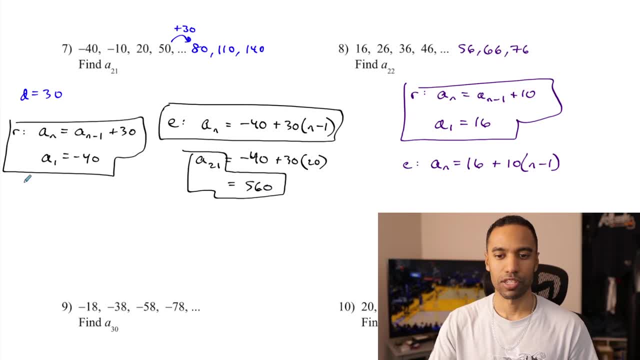 plus 10 times n minus 1. A sub 22 value the 22nd term is 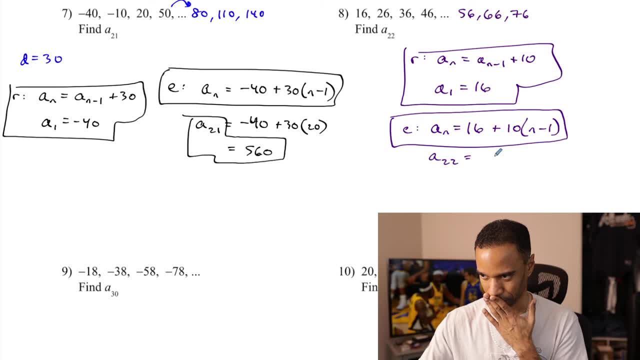 Now, my colors don't mean anything now, by the way, it seems like. A sub 22 is 16 plus 10 times 21. 210 plus 16 is 226. Okay. 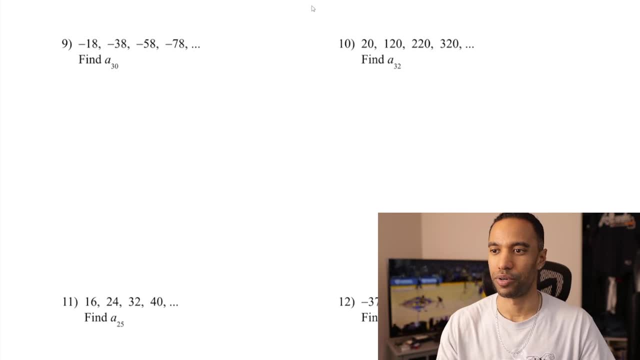 Four more. Man, I did this to my students, huh? They had to do all these? I hope they know it now. 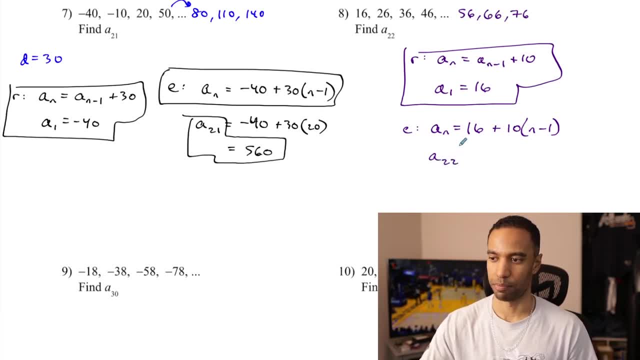 A sub 22,. the value of the 22nd term is Now. my colors don't mean anything now. by the way, it seems like A sub 22 is 16 plus 10 times 21.. 210 plus 16 is 226.. 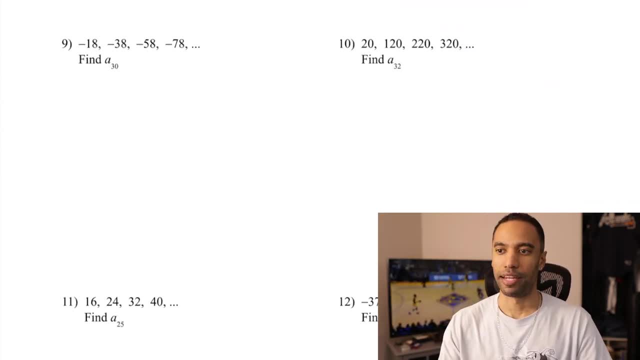 Okay, Four more Man. I did this to my students. huh, They had to do all these. I hope they know it now. Subtracting 20 each time, So now we're getting negative 98.. I'll just write minus 20 for you. 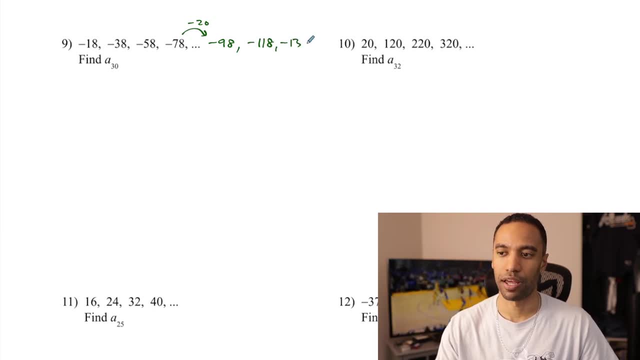 Negative 98,, negative 118, and negative 138.. Next three terms: recursion, So the recursive formula are: a sub n is a sub n minus one minus 20, where a sub one is negative 18.. The explicit rule: a sub n equals negative 18 minus 20 times n minus one. 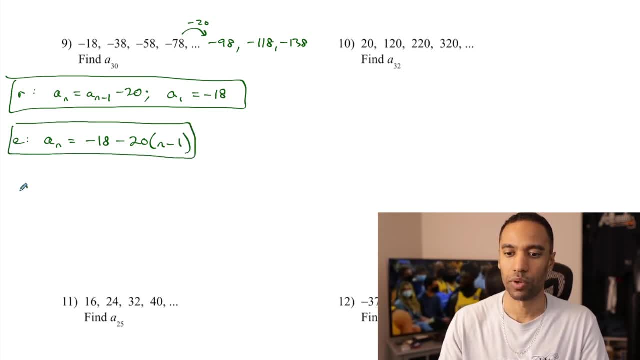 And as we substitute 30 into this thing, we'll get a sub 30 equals negative 18 minus 20 times 29.. Two times 29 is 58.. So 20 times 29 is 580.. So negative 18 minus 580 is negative 598.. 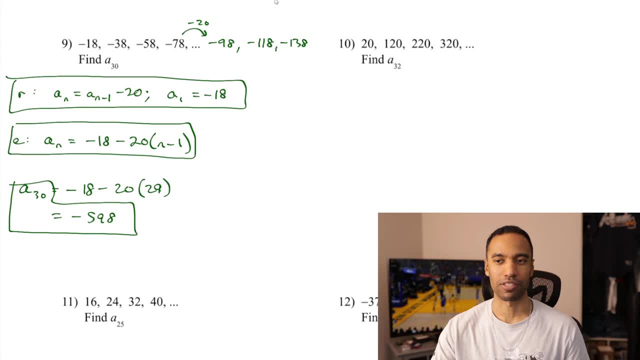 See how fast we get to go. now I feel better about things. Less to teach. There are a lot of different things we can do from problems, though, And, like I stated, coming to geometric sequences you are gonna hear about, arithmetic means. 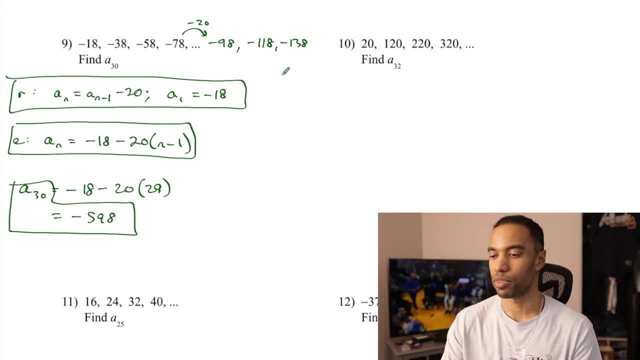 You are gonna hear about determining whether something's arithmetic, And you might see some things. They're mostly geometric, but you might find some things that are fraction or decimal based as well. All right, this time we are- ooh, we're adding 100.. 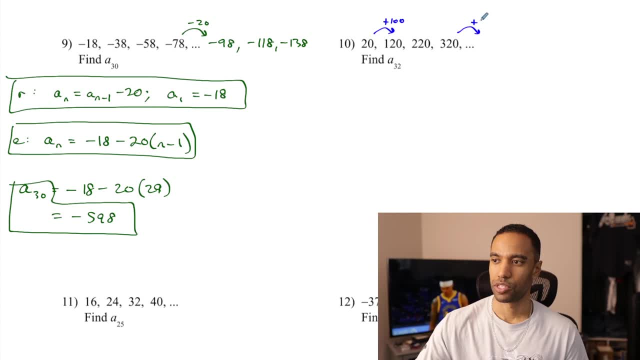 Look at us going up in the world here. So let's add 100 to some of these. What comes next? 520.. Then we got 520 and 620.. So here we go. Recursive rule: a sub n equals a sub n minus one plus 100. 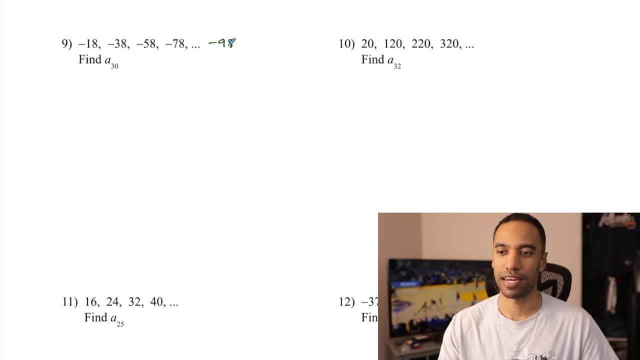 Subtracting 20 each time. So now we're getting negative 98. 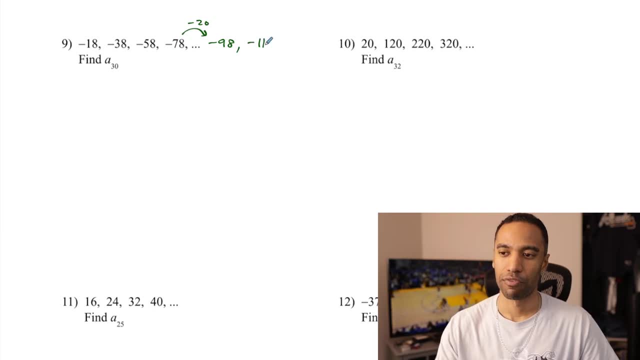 I'll just write minus 20 for you. Negative 98, negative 118, and negative 138. 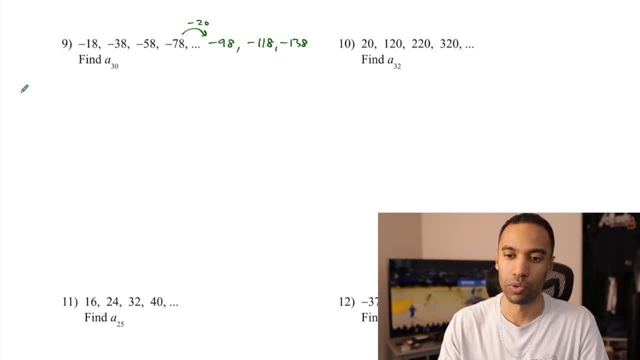 Next three terms, recursion. So the recursive 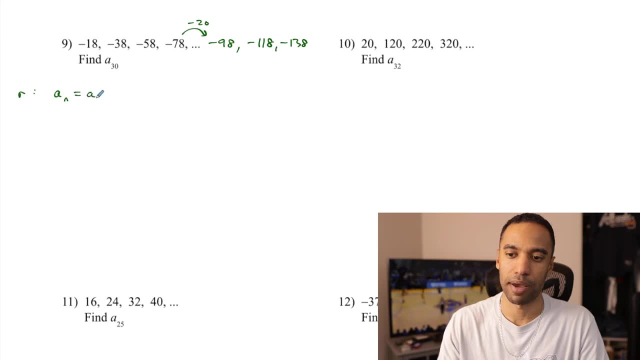 formula are a sub n is a sub n minus 1 minus 20, where a sub 1 is negative 18. 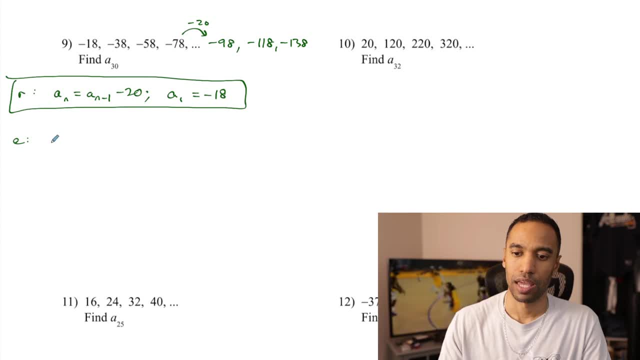 The explicit rule, a sub n equals negative 18 minus 20 times n minus 1. And as we substitute 30 into this thing, we'll get a sub 30 equals negative 18 minus 20 times 29. 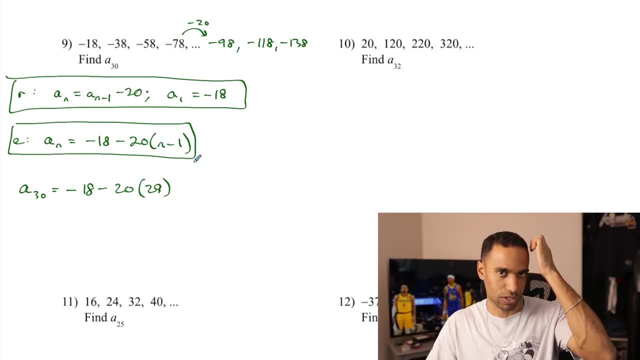 2 times 29 is 58, so 20 times 29 is 580. So negative 18 minus 580 is negative 598. 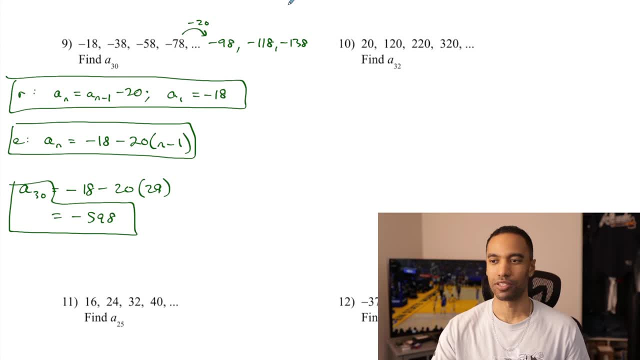 See how fast we get to go now? I feel better about things. 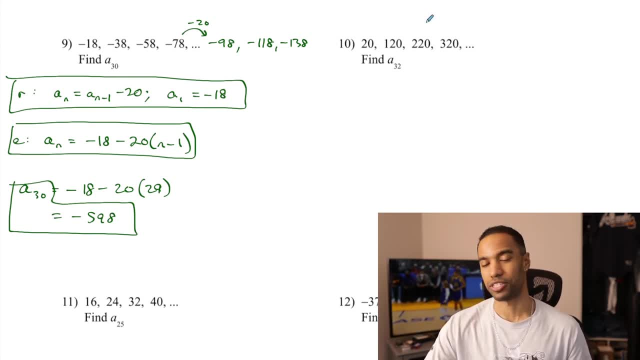 Less to teach. There are a lot of different things we can do from problems, though. And like I stated, coming to geometric sequences, you are going to hear about arithmetic means. You are going to hear about determining whether something's arithmetic. And you might see some things. They're mostly geometric, but you might find some things that are fraction or decimal based as well. Alright, this time 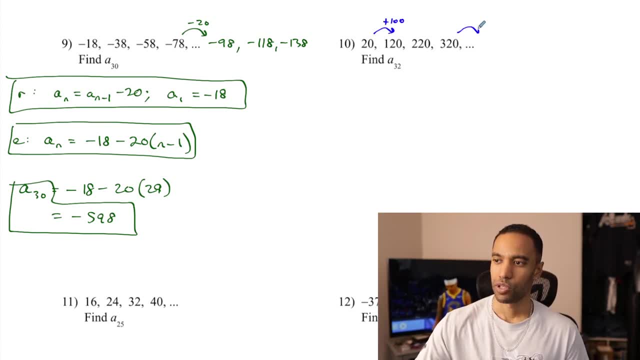 we are adding 100. Look at us going up in the world here. So let's add 100 to some of these. What comes next? 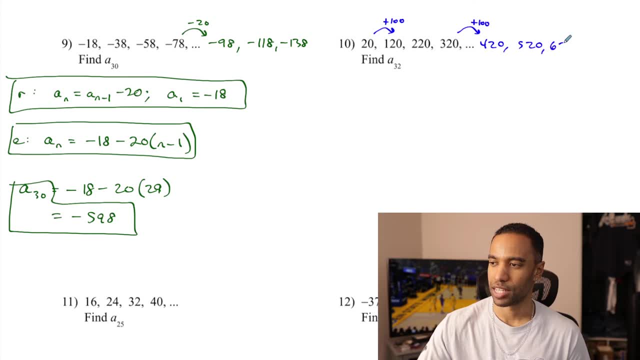 520. Then we got 520 and 620. So here we go. 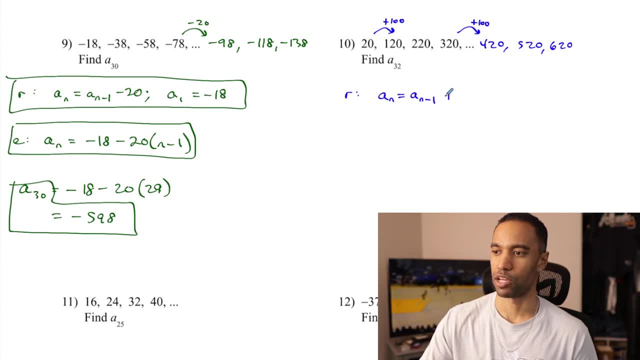 Recursive rule, a sub n equals a sub n minus 1 plus 100. 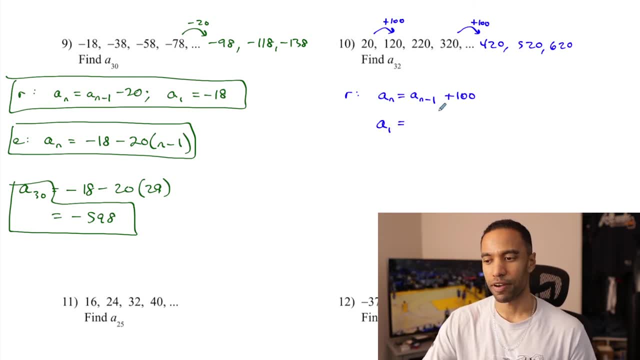 I gave so many problems. a sub 1 equals, especially if I wasn't going to do 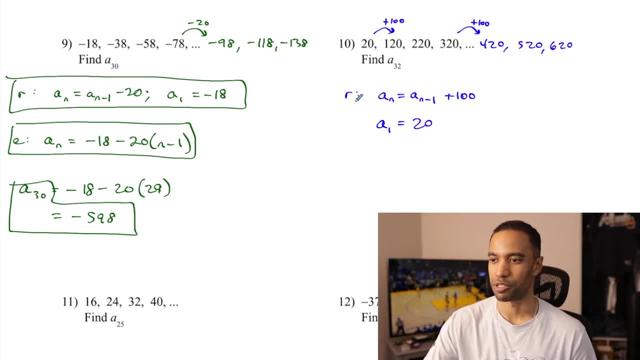 any decimals. If I wanted to really do some different things, I would have done decimals there. 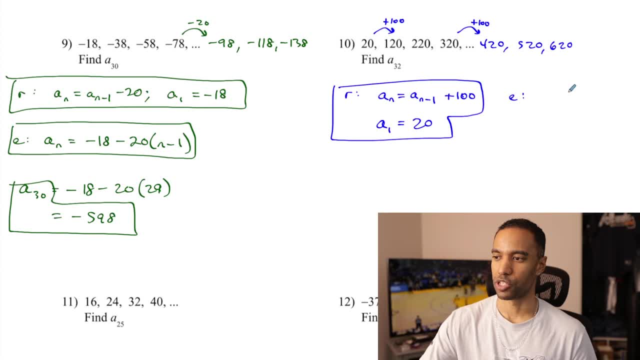 a sub 1 is 20. The explicit rule is a sub n equals the value of the first term plus 100 n minus 1 times. 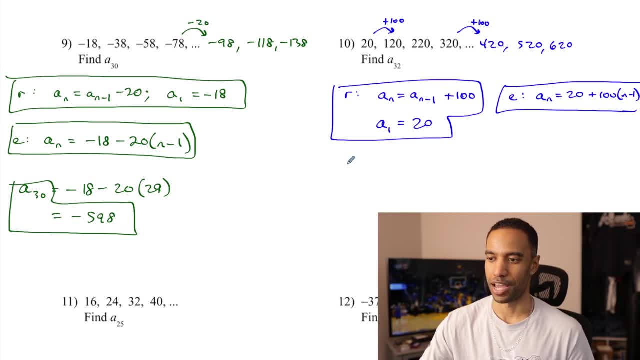 So let's add 100 31 times, right? 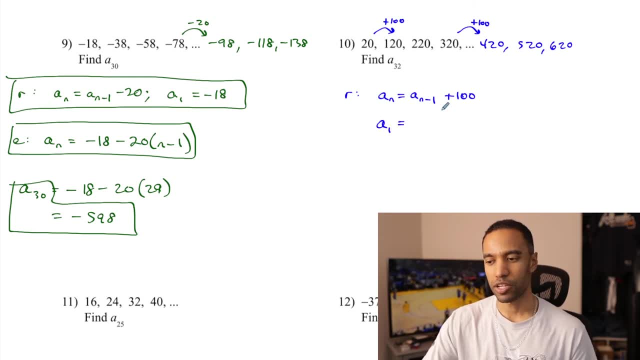 I don't know why I gave so many problems. a sub one equals, especially if I wasn't gonna do any decimals. If I wanted to really do some different things, I would have done decimals there. a sub one is 20.. The explicit rule is: a sub n equals the value. 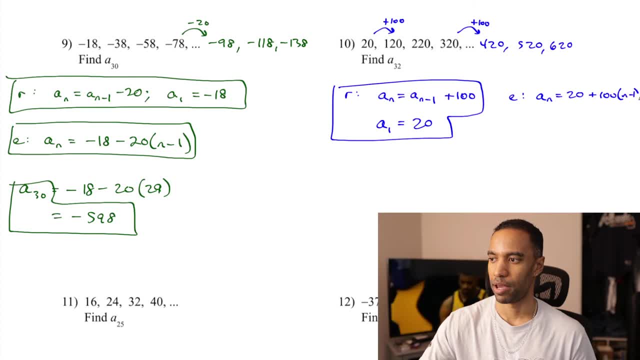 of the first term, plus 100, n minus one times. So let's add 100 31 times, right? a sub 32 is 20.. A sub 32 is 20 plus 100, 31 times 3100 plus 20 is 3120.. 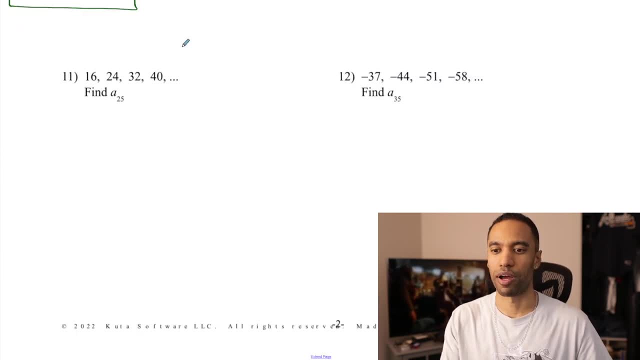 Very fast to find these when you have the explicit rule. Last two problems here: Adding eight, as that is 40 minus 32, et cetera. So let's add eight, Three mass times: 48,, 56,, 64.. 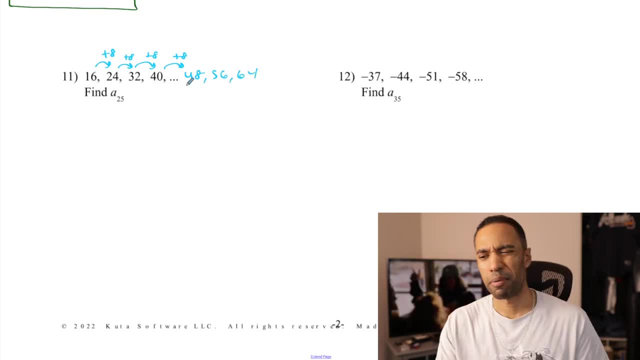 Well done. See, I'm not plugging. I'm not doing a sub five, a sub six, a sub seven. I'm not plugging them into an explicit rule that I don't even have yet, But we're gonna get it after we get the recursive rule. 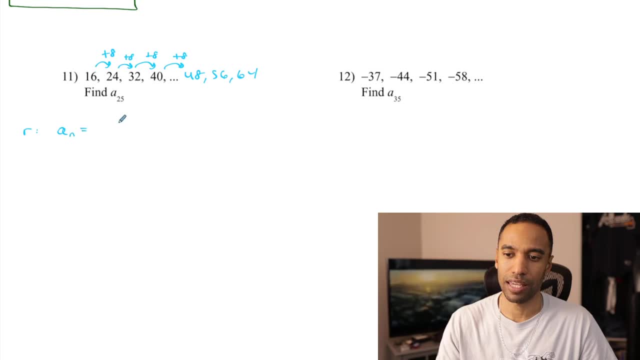 Don't mind if I do Recursive rule: a sub n equals a sub n minus one plus eight, where a sub one happens to equal 16.. The explicit rule is: a sub n equals 16 plus eight times n minus one, at least that version of the rule. 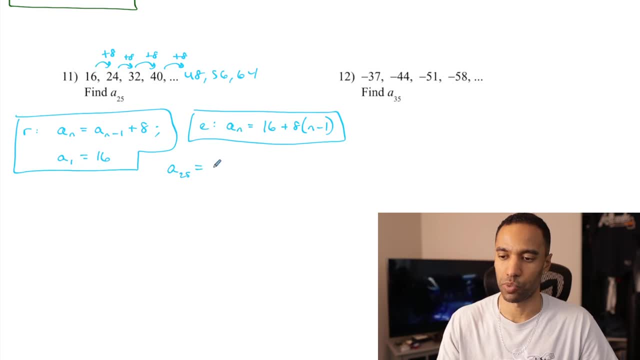 And a sub 25, based on the explicit rule, is 16 plus eight times 25 minus one is 24.. Now, eight times 24 is well, eight times 25, hear this: eight times 25 is eight quarters. 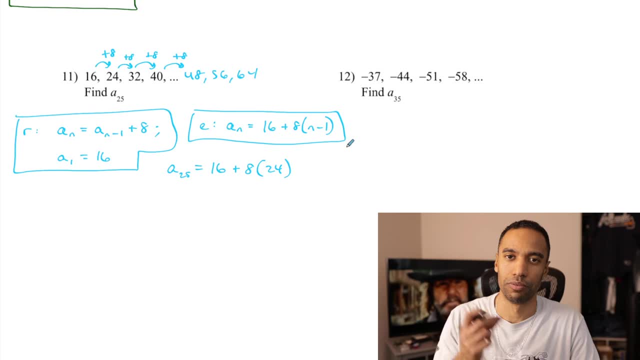 $2 is 200 minus eight is 192.. All right, Some people are just like. I can do eight times 20 and eight times four and get that. What was the number 192?? 192 plus 16 is 200.. 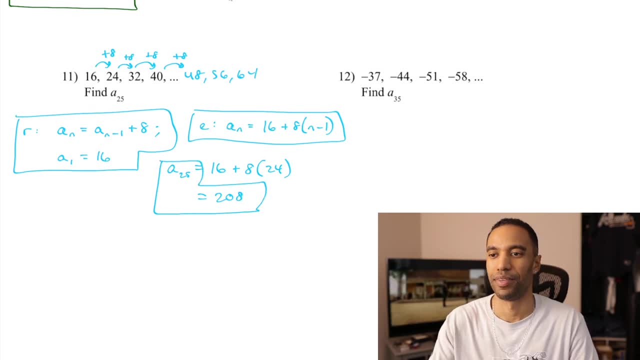 All right, Yeah, I wanted to speed through it at this point here. Last one, a little past the half hour mark. Last one: we are subtracting seven, So we're going to get negative 65,, negative 72, and negative 79.. 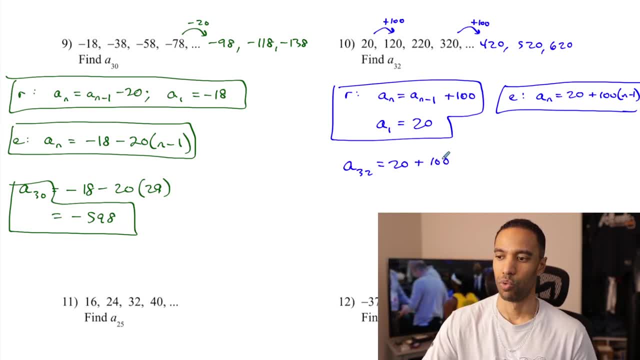 a sub 32 is 20 plus 100 31 times. 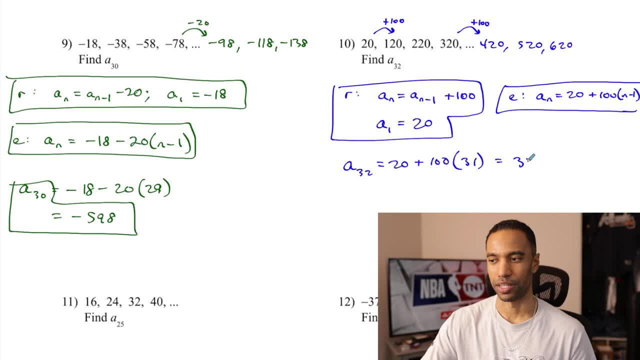 3100 plus 20 is 3120. 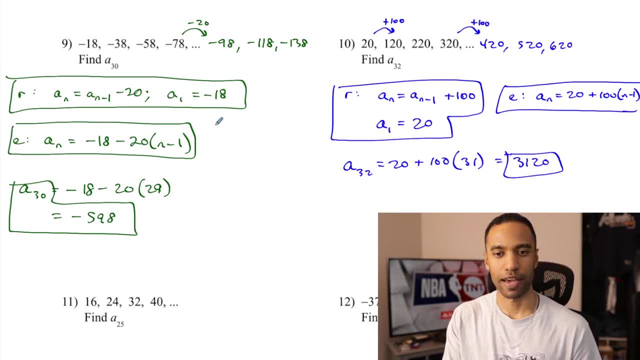 Very fast to find these when you have the explicit rule. 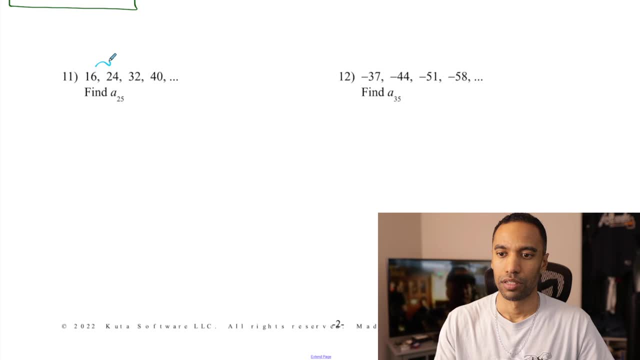 Last two problems here. Adding 8 as that is 40 minus 32, etc. 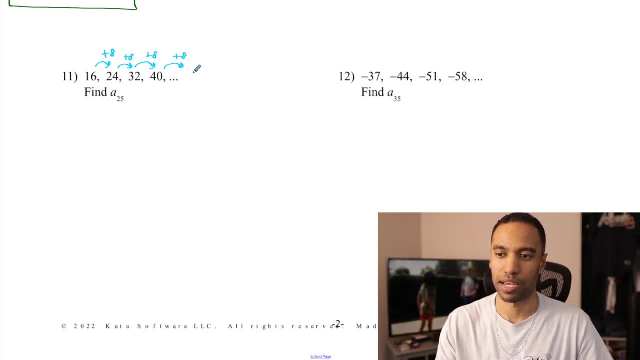 So let's add 8 3 mass times 48, 56, 64. 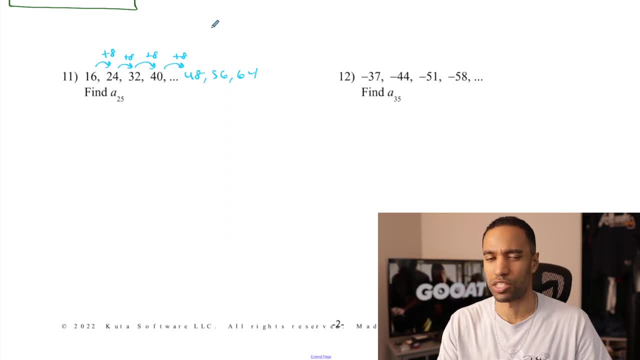 Well done. See, I'm not doing a sub 5, a sub 6, a sub 7. 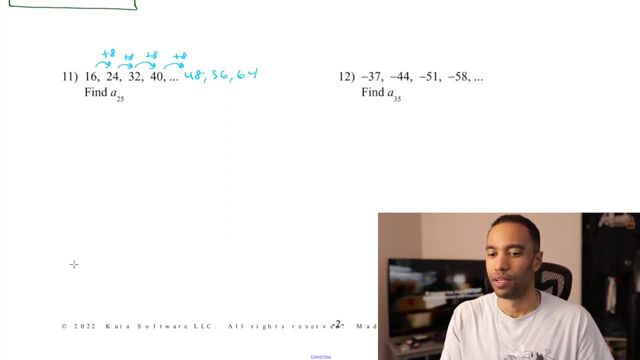 I'm not plugging them into an explicit rule that I don't even have yet. We're going to get it after we get the recursive rule. Don't mind if I do. 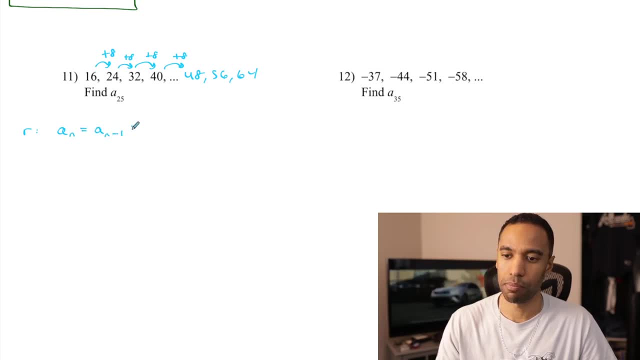 Recursive rule, a sub n equals a sub n minus 1 plus 8, where a sub 1 happens to equal 16. 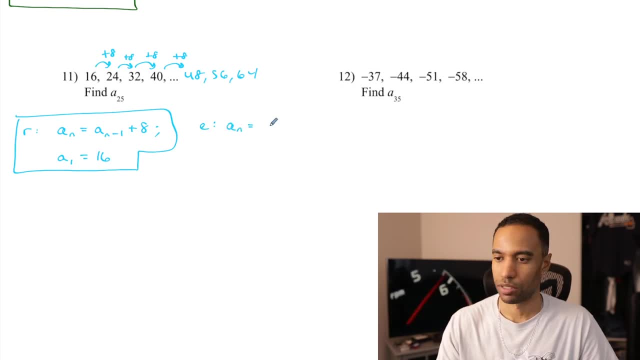 The explicit rule is a sub n equals 16 plus 8 times n minus 1. At least that version of the rule. And a sub 25, based on the explicit rule, is 16 plus 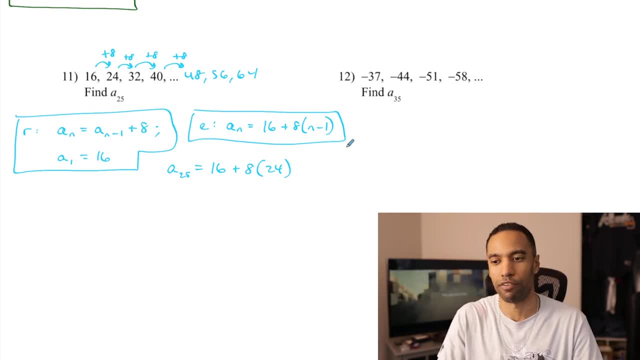 8 times 25 minus 1 is 24. Now, 8 times 24 is, well, 8 times 25 hear this, 8 times 25 is 8 quarters. 2 dollars is 200. Minus 8 is 192. 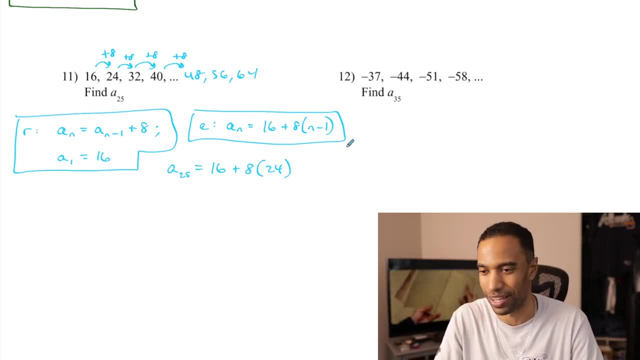 Some people are just like, I can do 8 times 20 and 8 times 4 and get that. What was the number? 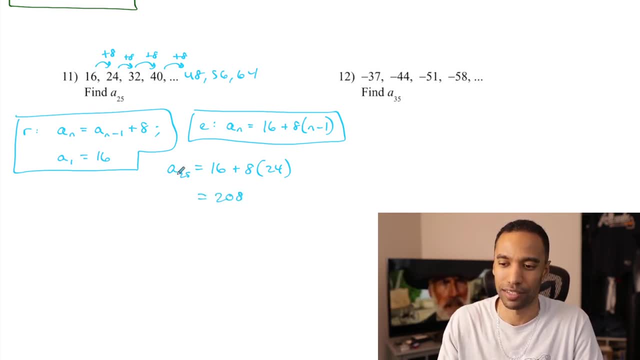 192? 192 plus 16 is 208. 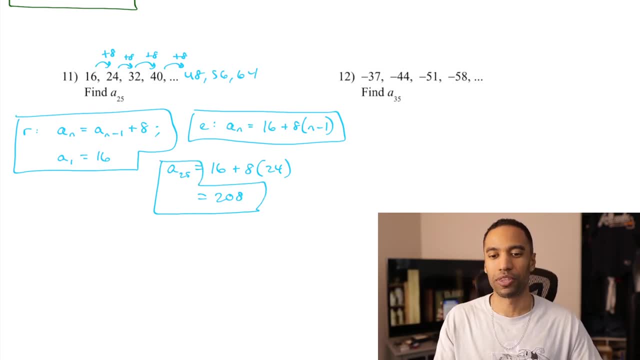 Alright. Yeah, I wanted to speed through it at this 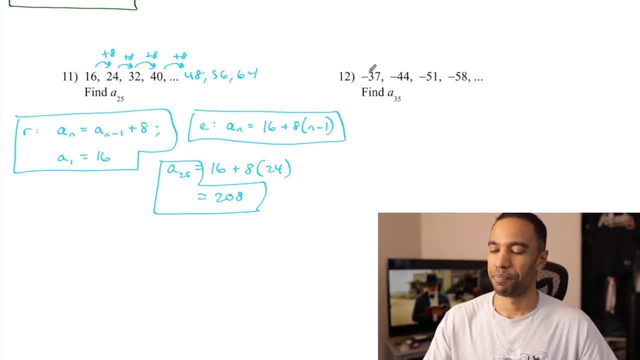 point here. Last one, a little past the half hour mark. Last one, 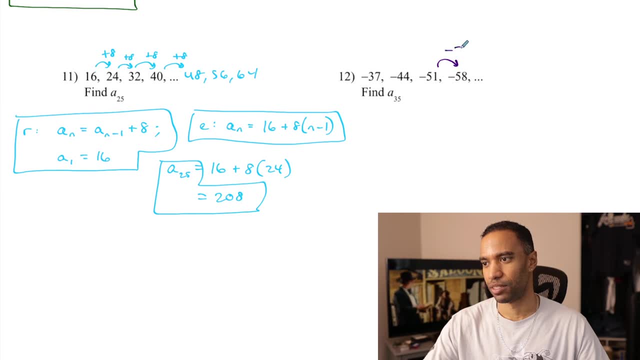 we are subtracting 7. So, we're going to get negative 65, 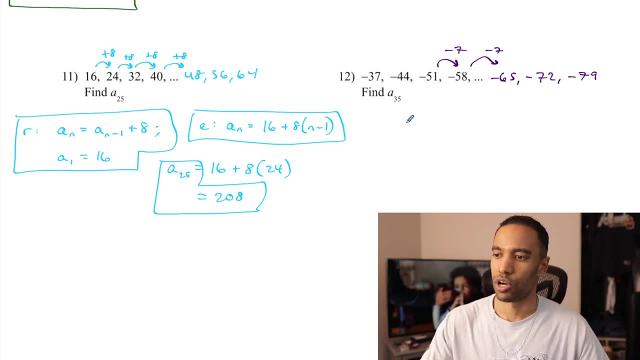 negative 72, and negative 79. So, a sub 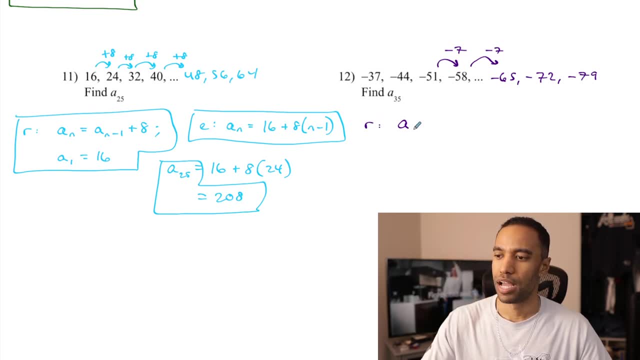 excuse me, recur, yeah, recursive rule, a sub n equals a sub n minus 1 minus 7, starting